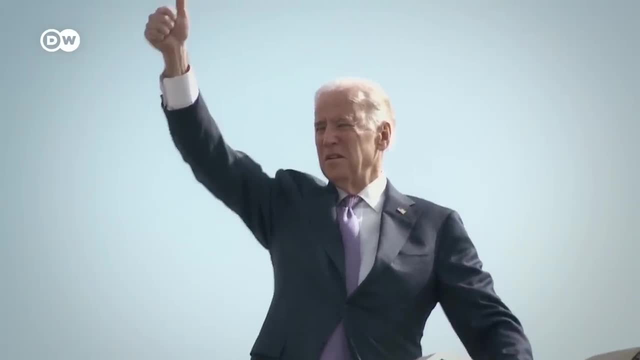 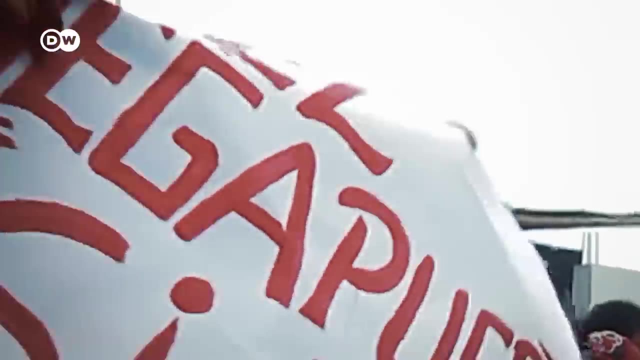 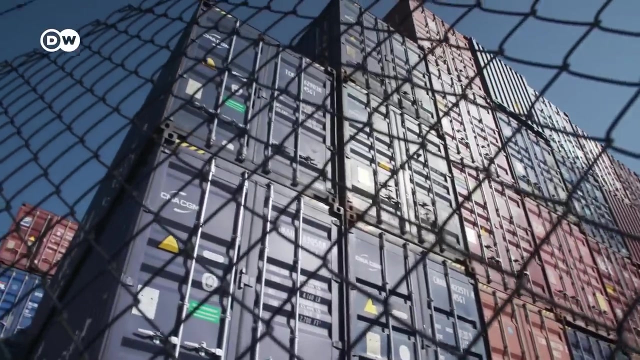 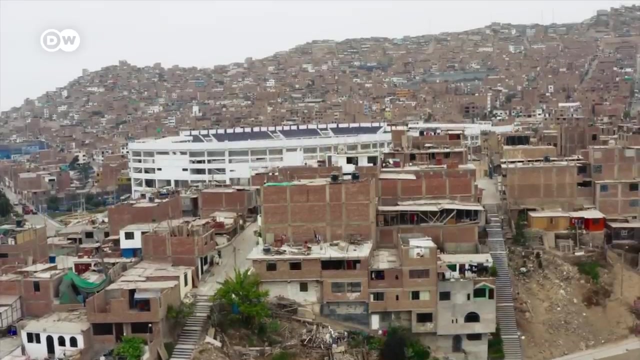 And the US continues to believe in America first, but it's the world's poor who are paying the price for this global competition. The German city of Duisburg has reawoken from the ashes of its past thanks to China. As a developing country, Peru sees few benefits from globalisation and is engulfed in poverty. 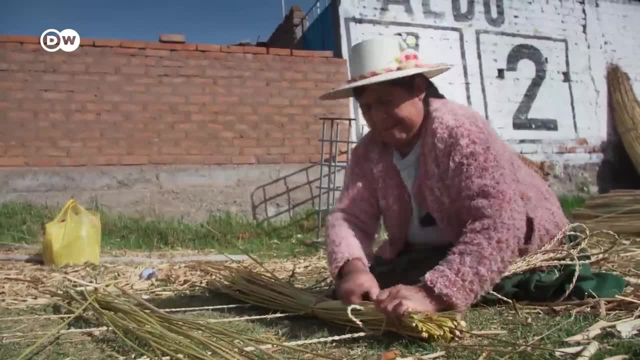 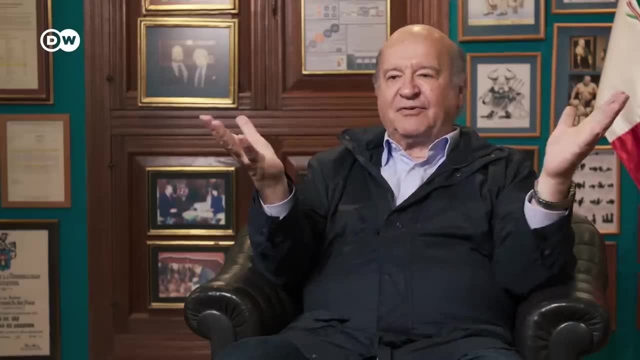 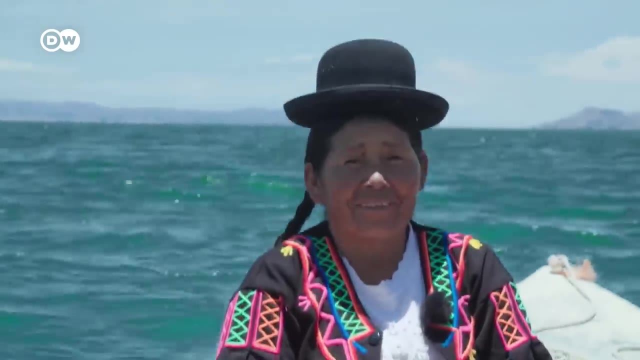 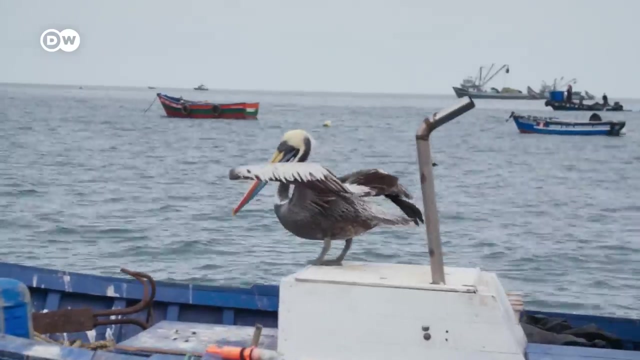 But somehow or other we've got to understand that globalisation works, but it has not reached more than 30% of the world population. Very simple: Do we really make the most of trade opportunities in a global economy, In a globalised world? 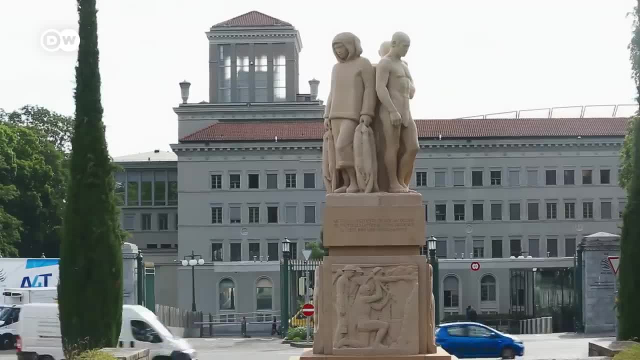 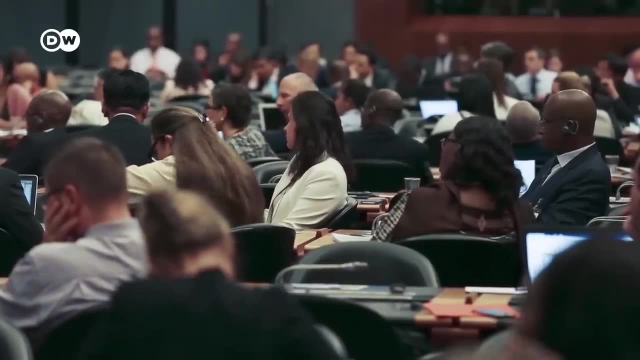 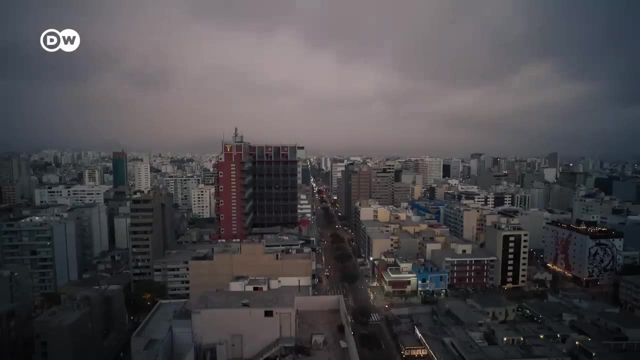 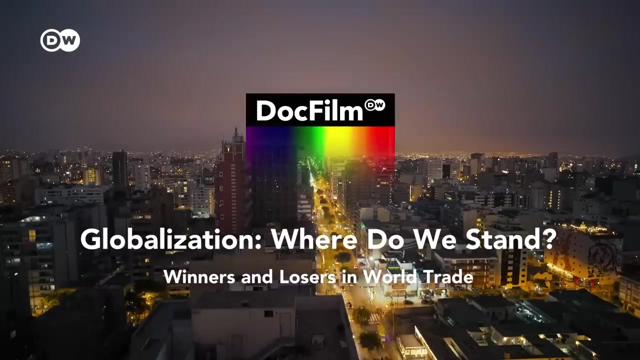 Some are questioning the World Trade Organisation as the guardian of fair trade and, with it, globalisation itself. I don't even think you can block globalisation, but we need to look carefully at who are the winners and losers. We need to look at who are the winners and losers. 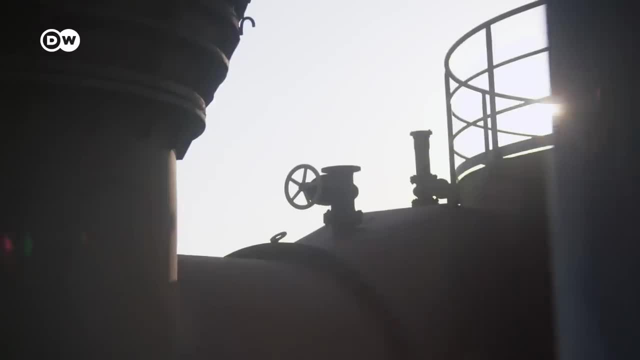 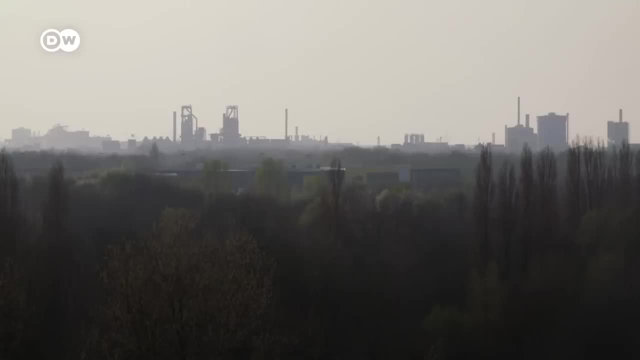 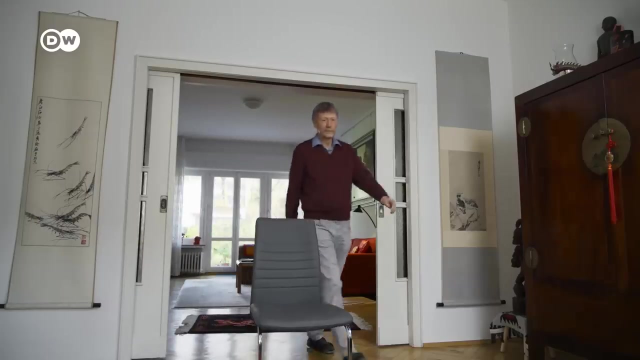 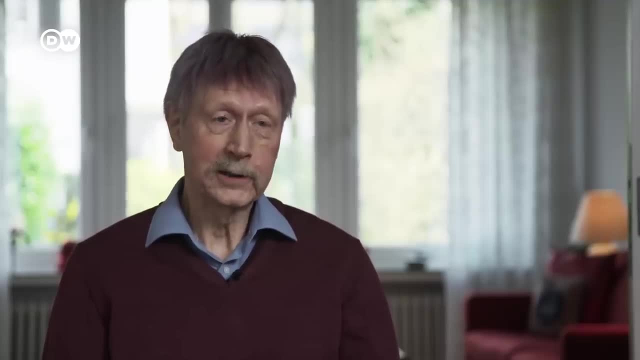 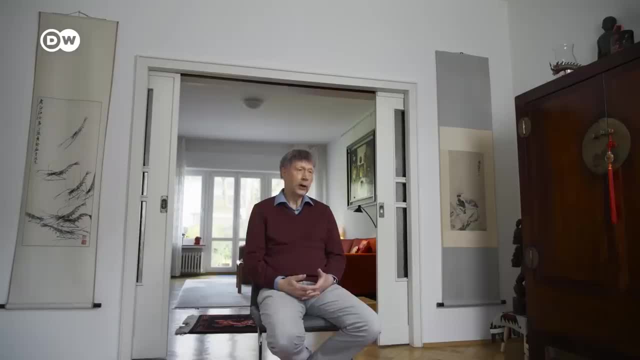 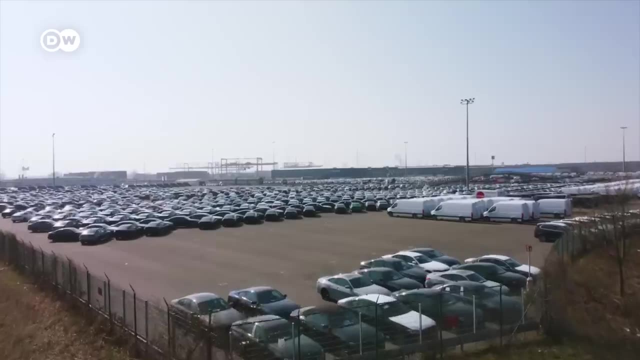 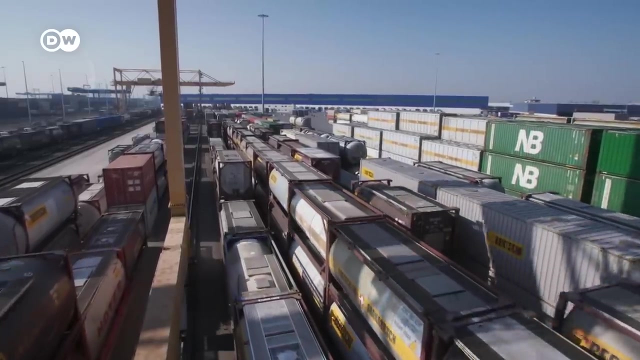 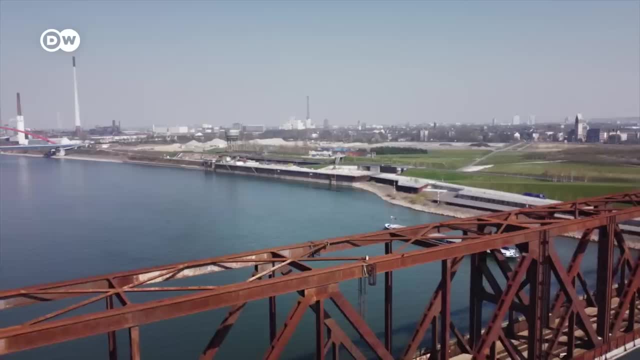 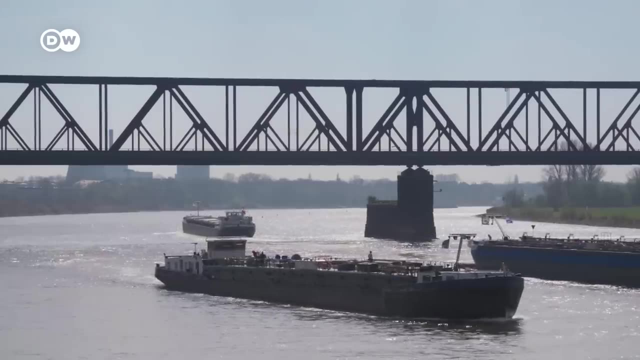 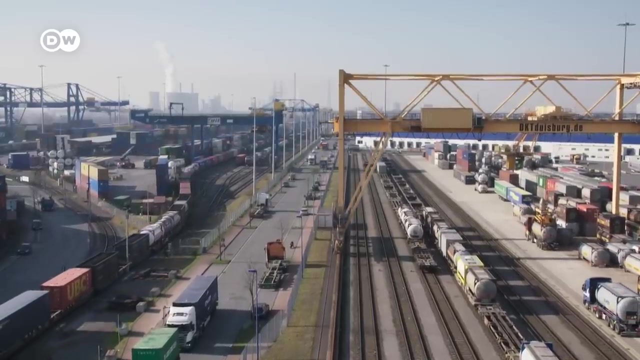 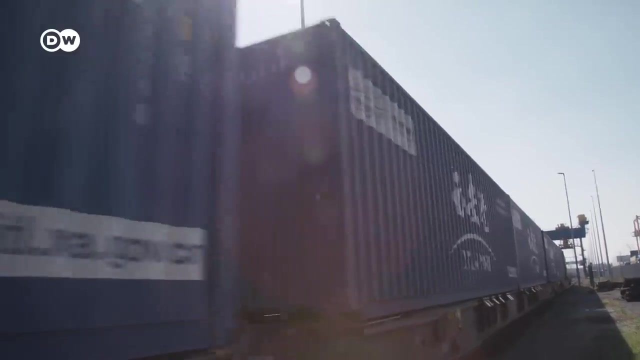 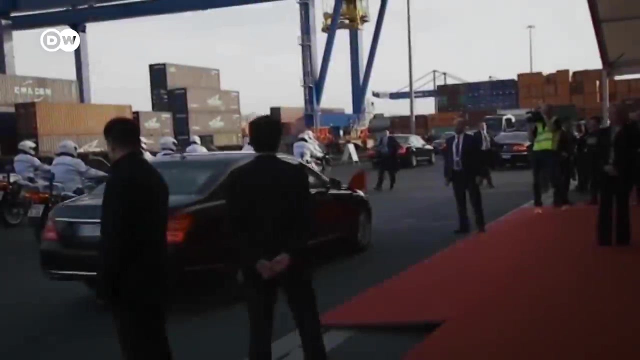 Goods arrive just as clients need them, reducing the need for costly logistics and storage. China is the port's most important trading partner. Ironically, after flooding Europe and the US with cheap steel, the economic giant has now emerged as Duisburg's saviour. 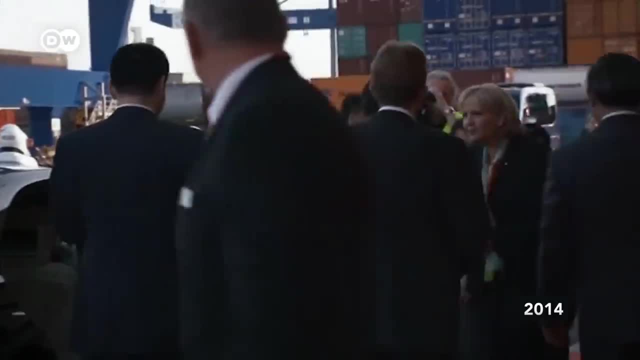 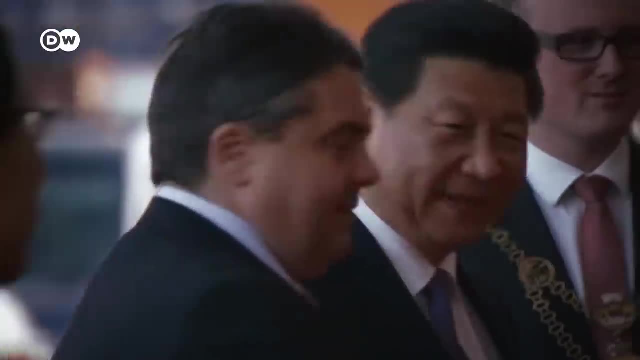 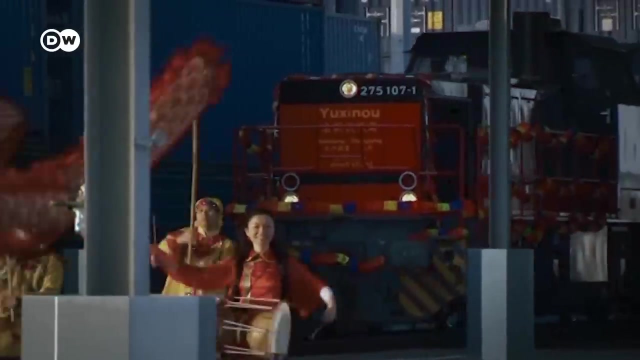 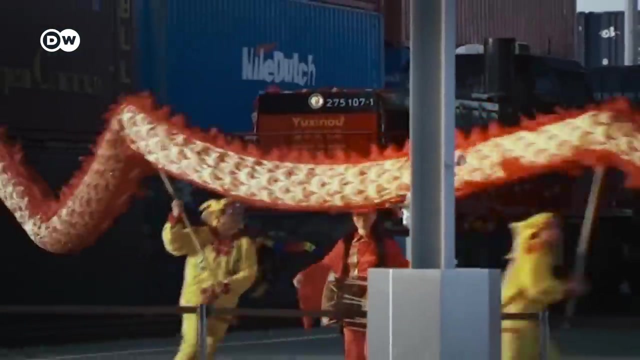 In 2014,. Chinese President Xi Jinping hailed Duisburg as the final stop on the New Silk Road And as China's gateway to Europe. Duisburg was happy to enter the alliance with its promise of dozens of freight trains every week, but negotiated carefully. 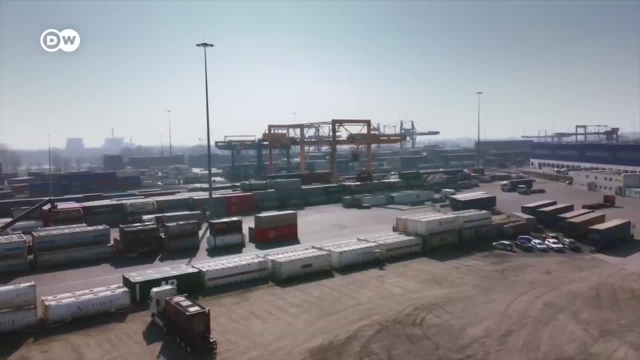 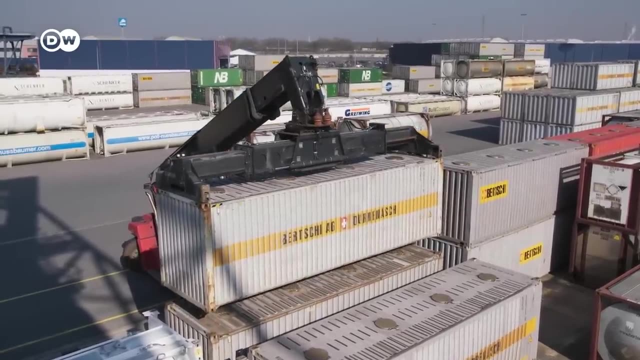 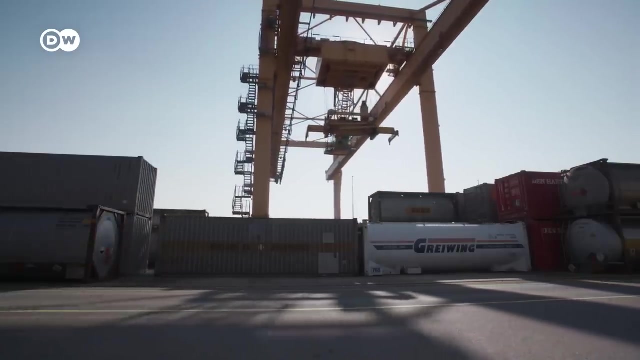 The city had been warned. China was luring countries along the route with cheap loans for the expansion of their infrastructure And, as a result of excessive debt, the ports of Piraeus in Greece and Hambantota in Sri Lanka are now in the hands of Chinese operators. 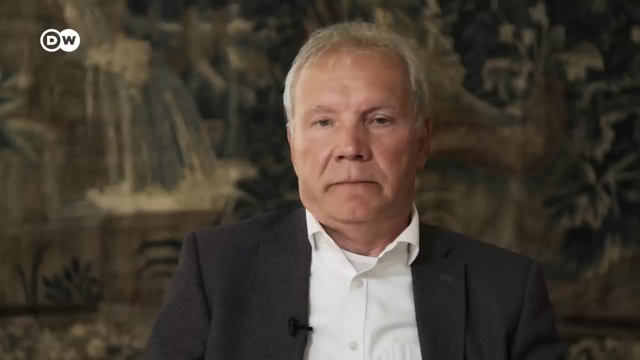 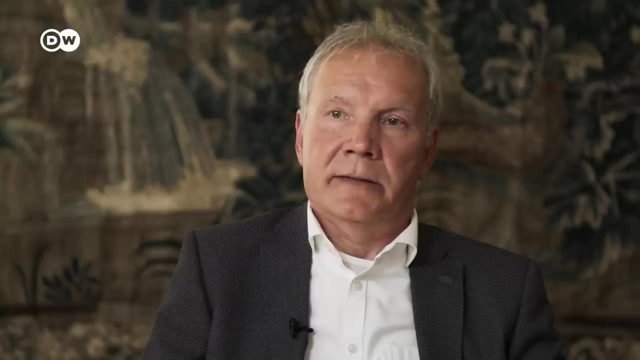 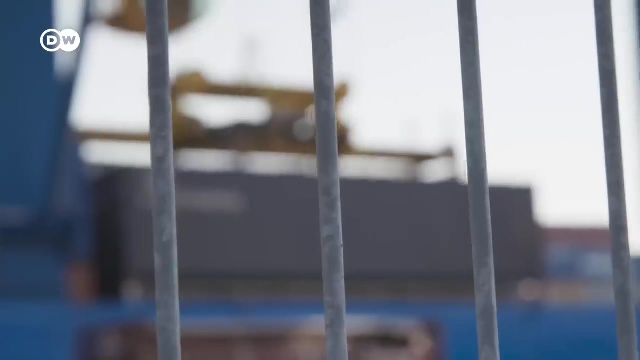 «From our point of view, it is very worrying- Or from my point of view, it's very worrying- what's happening in other parts of the world along the New Silk Road. Piraeus and Sri Lanka are not the only troubled ports with financing. 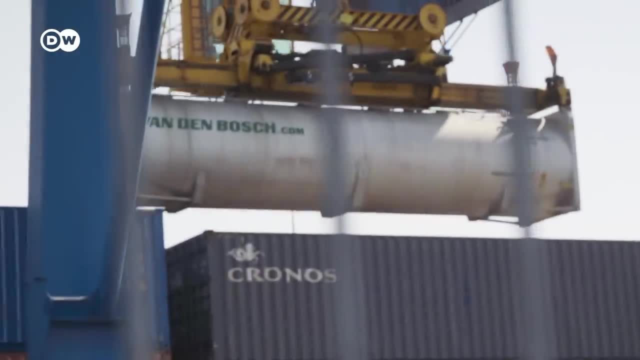 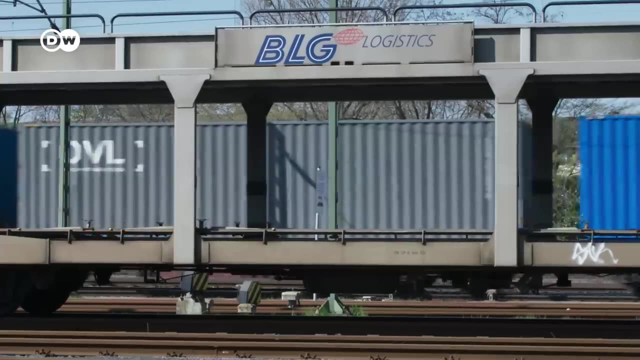 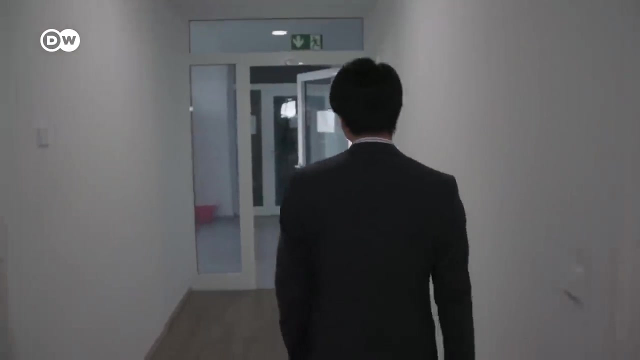 It's not the only one. It's fundamentally different. here in Duisburg, All of the port infrastructure belongs to the port». Transport by ship would be cheaper. Nevertheless, some 60 freight trains arrive from China every week. For the return journey, the wagons load up goods from all over Europe. 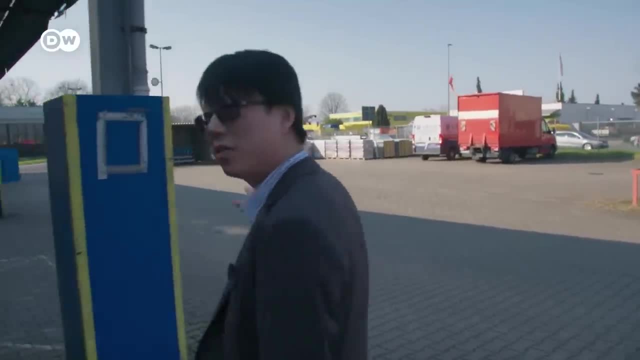 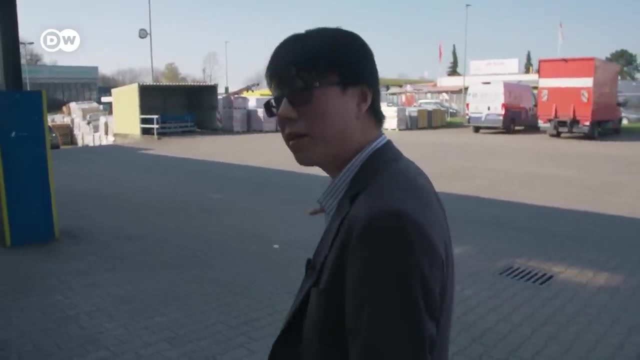 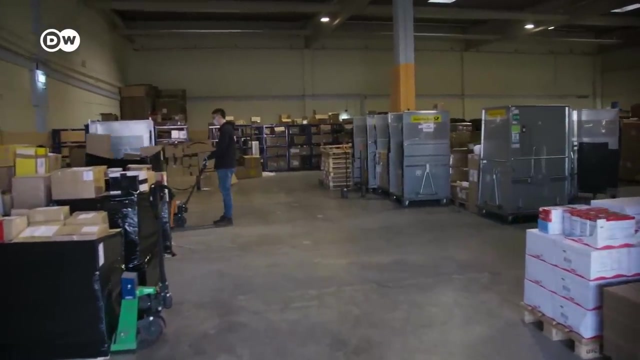 «There are about 70 employees so divided in the UK, China and Germany». About 70 employees are spread across the UK, China and Germany. We pick up e-commerce parcels with our own vehicles. These have just come in from France today. 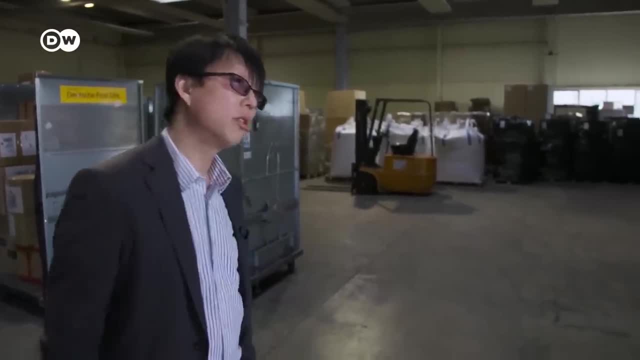 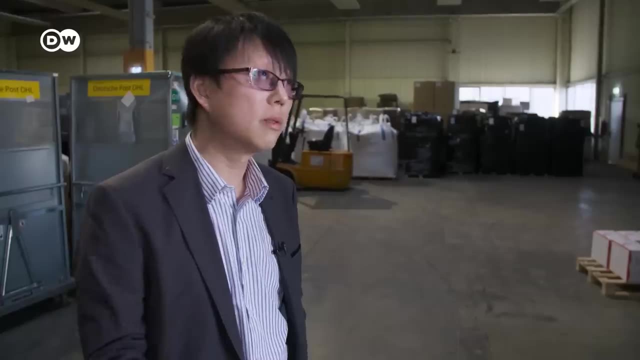 We'll load them into containers and then they'll go to China by rail. They'll reach China in two weeks, in two to three weeks. It's very fast. at the moment, The Chinese know Duisburg. When you arrive here from Beijing, you don't even see Berlin. 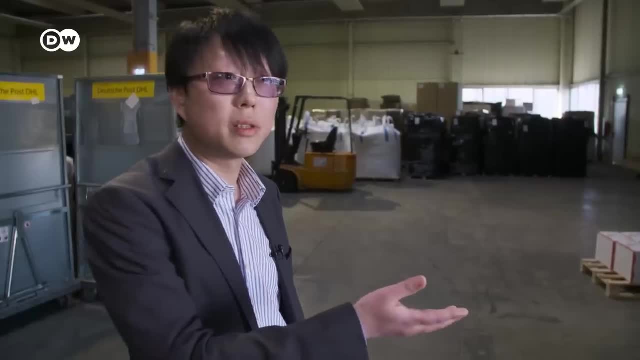 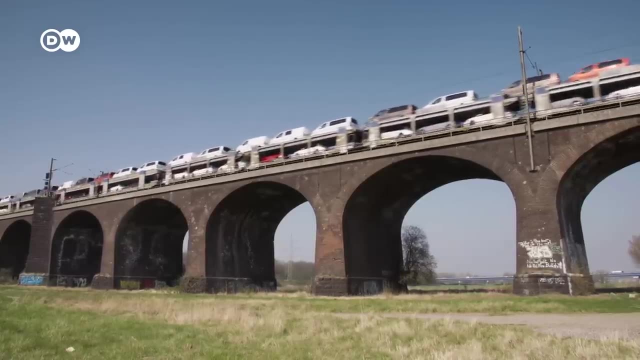 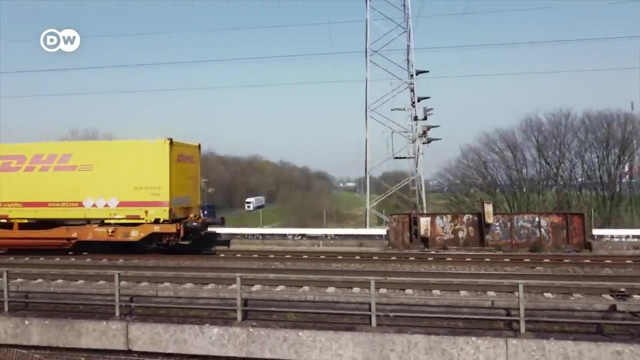 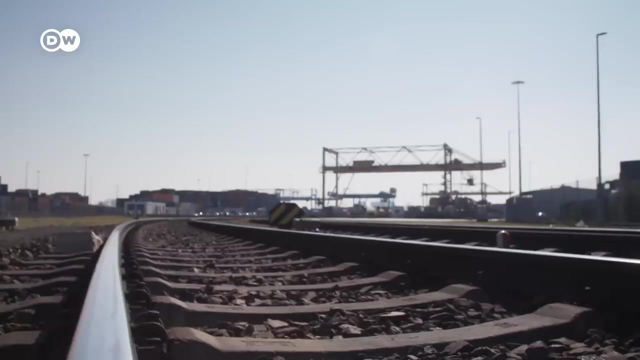 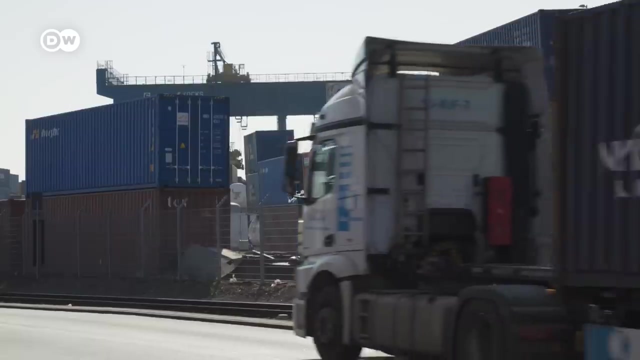 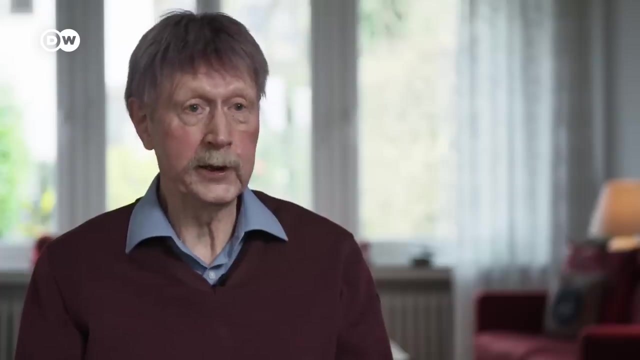 You see Duisburg as the center of Europe. Empty tracks have become an increasingly common sight since Russia marched into Ukraine. Supply chains are vulnerable, a risk, But Duisburg is preparing for the future. You can't lean back and say we have 60 trains a week from China. 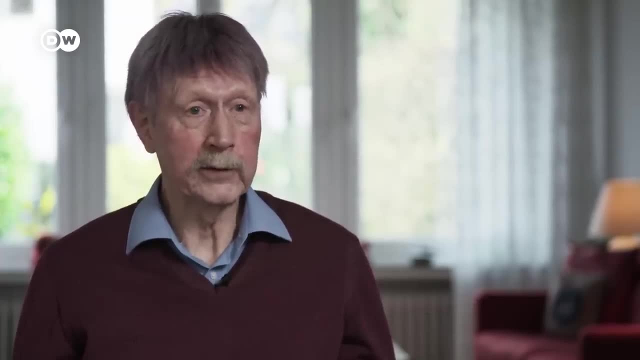 Who knows whether this will continue, And we have to consider alternatives. Duisburg has also invested in Trieste, for example, to build a site there that could be supplied via Turkey and southern Europe. Duisburg is already developing alternatives, Without a plan. 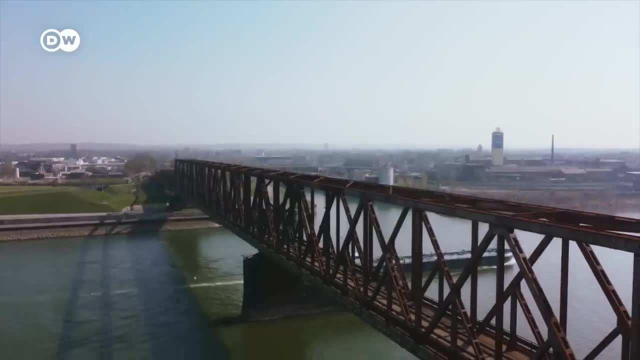 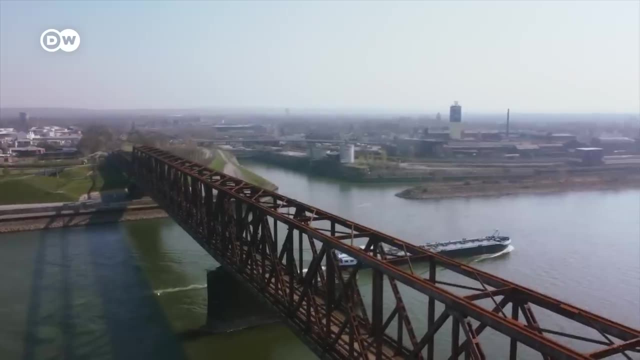 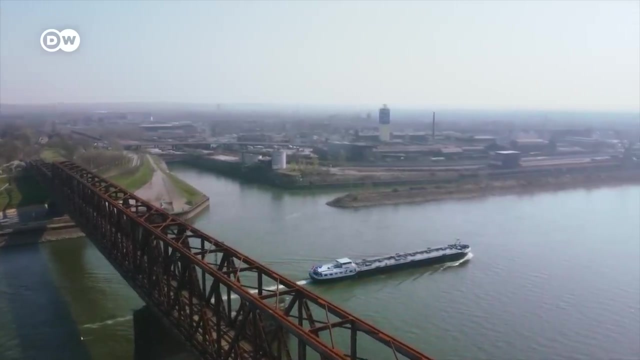 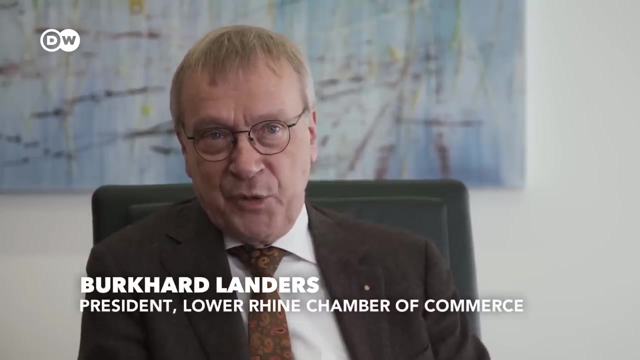 Abandoning the concept behind this port. Duisburg's strategy in the global logistics and transport battle seems effective. Forge alliances, but stay independent and flexible. I think what the corona pandemic of the last two years has shown us is that global trade. 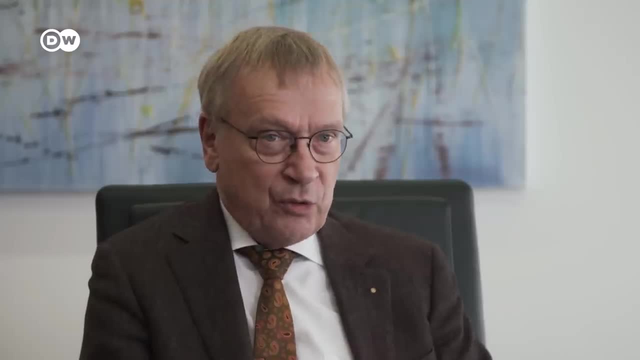 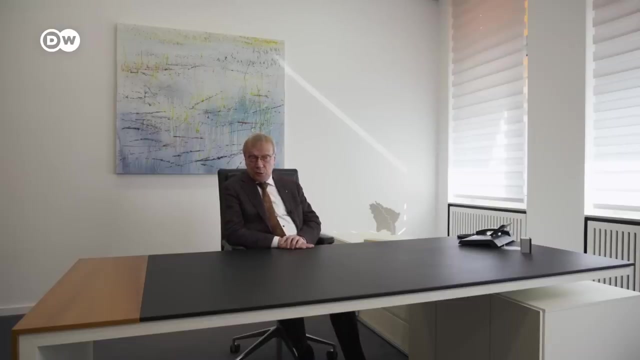 is more intricate than we suspected. It's easy to think that supply chains will also take the lead, So we have to adjust to having multiple suppliers in several countries to try to limit the geopolitical risk. One consequence will probably be more expensive products, Because what China is offering is very attractive. 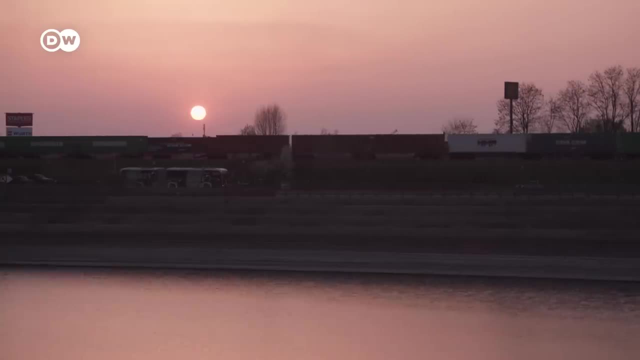 It's a very technologically advanced country. Chinese competition will increase in markets where it is not yet so clearly felt. So we need to experience the Chinese competition in the markets where we are not yet so clearly aware that China has a threat. China is a very sensitive country. 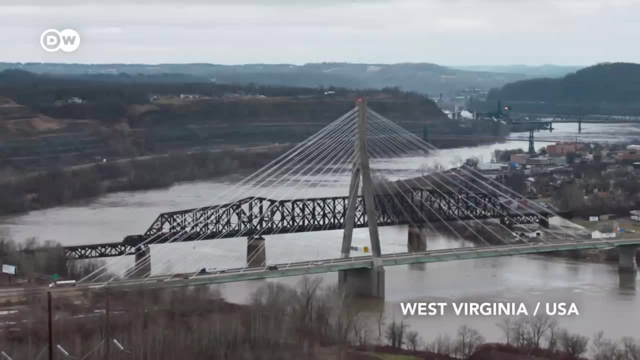 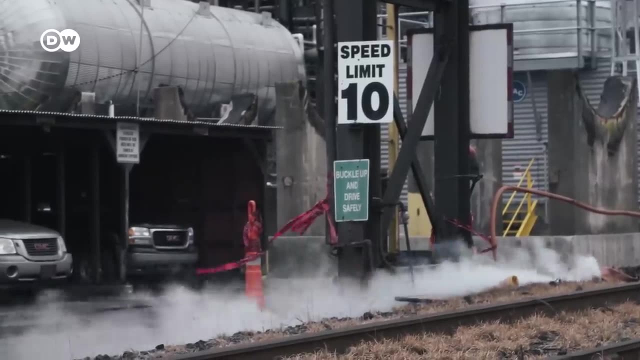 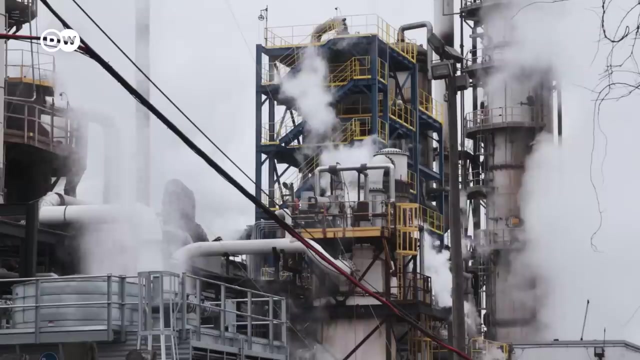 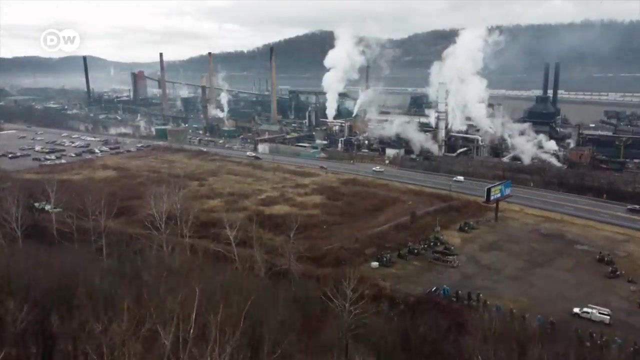 not so clearly yet". Unlike Duisburg, the American steel industry is having a hard time developing new markets, even though it's been fighting cheap competition from overseas for 40 years. Follensbee, West Virginia Coke for steel production is produced here, But now this? 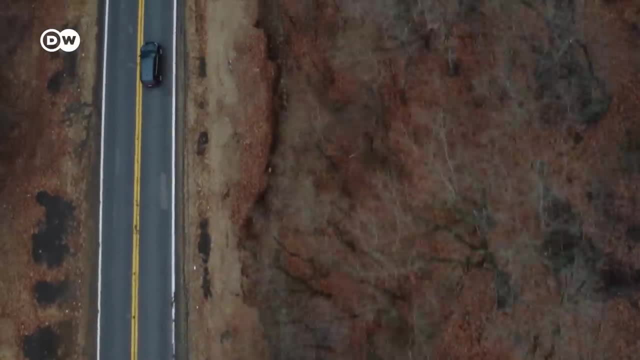 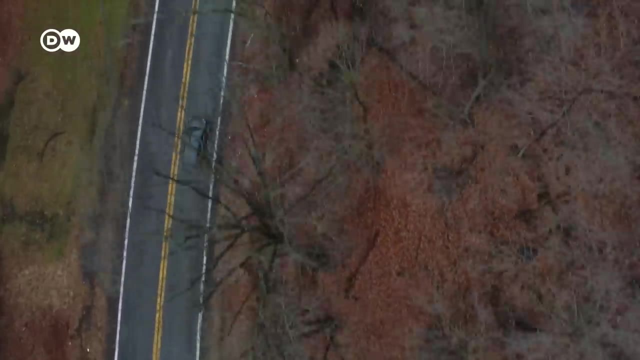 plant in the famed American Rust Belt is closing. Um, you know, I'd love to sit here and say that steel is going to be here forever. but 20 years ago, 40 years ago, if you were in Pittsburgh, you didn't think steel was going. 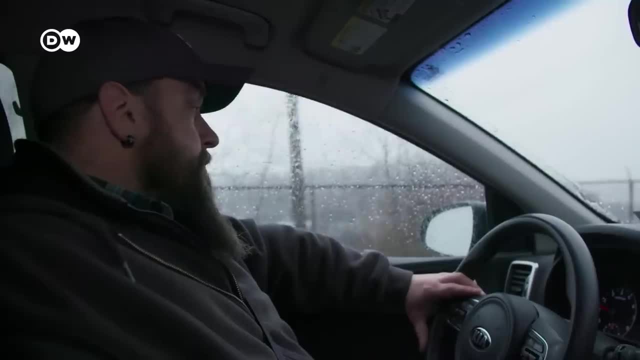 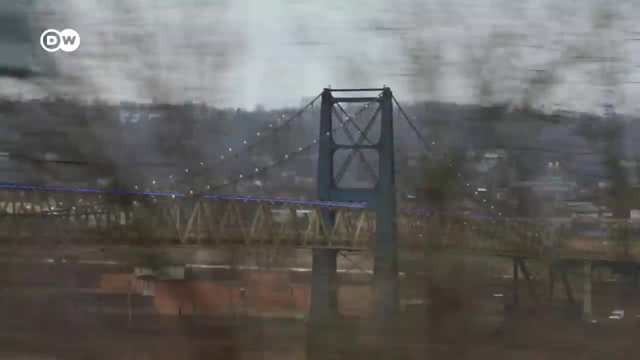 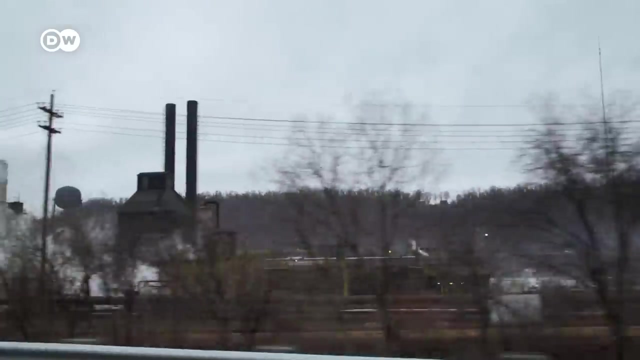 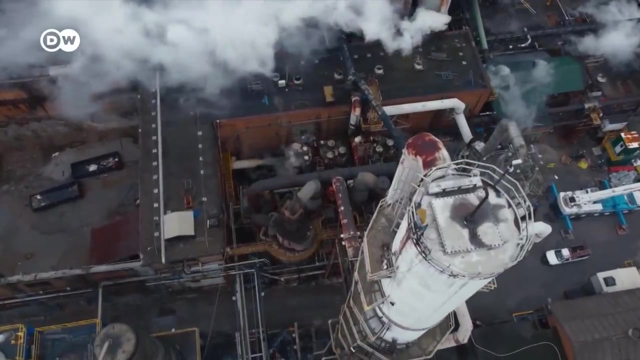 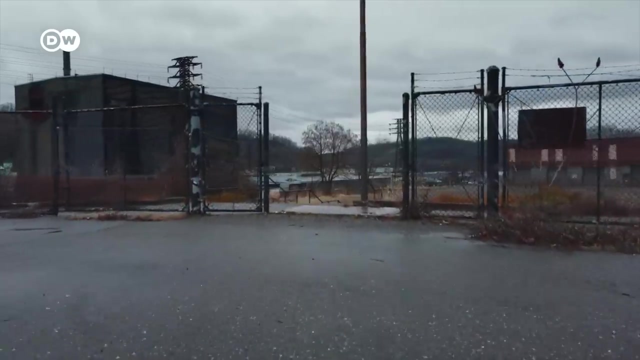 away forever, But there's almost nothing left there. Steel made the USA rich and powerful. The railroad, machine and automobile industries were the biggest customers. Two hundred and eighty-eight people will now lose their jobs when the Coke plant closes, And nearby Weirton has seen the closure of several steel mills since the 1990s. 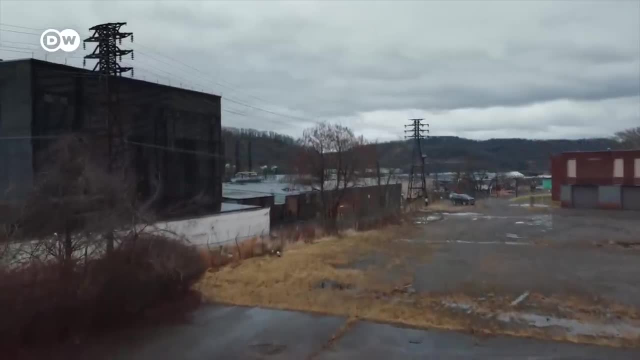 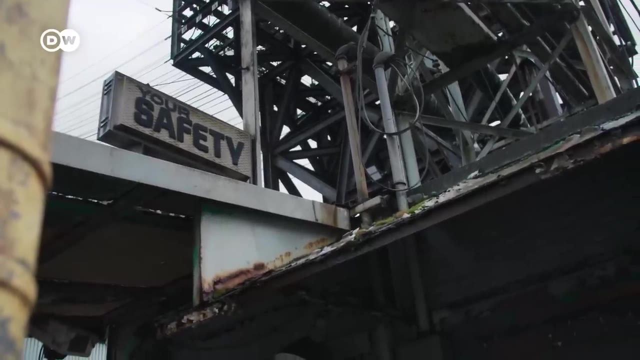 I saw this happen at Weirton. Weirton used to be basically totally just on their own down there. They didn't have to do to depend on anything. They made their own center And then they shut the coke plant down. They said: we can buy coke cheaper on the market, And that was true They could, But once they could no longer make those products, and then these companies that were selling it had control of it. they started raising their prices. As early as 2002, global trade meant cheap steel for markets. 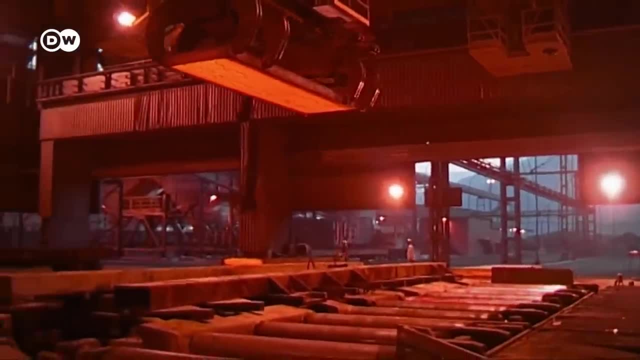 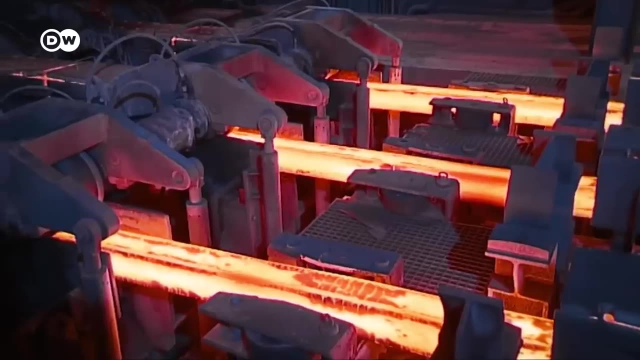 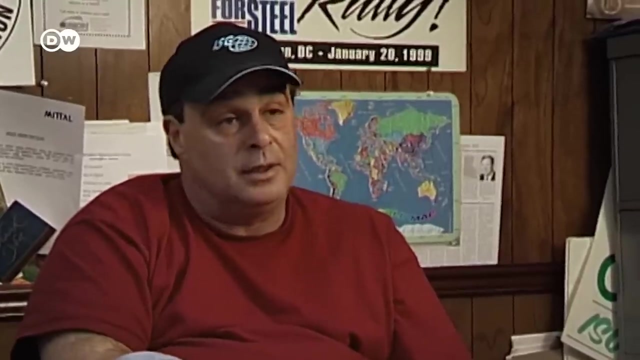 everywhere. To protect the US, President George W Bush decided to impose import tariffs on foreign steel. The World Trade Organization, the WTO, the arbiter of free and fair trade, was caught in the crosshairs. US unions backed the move. 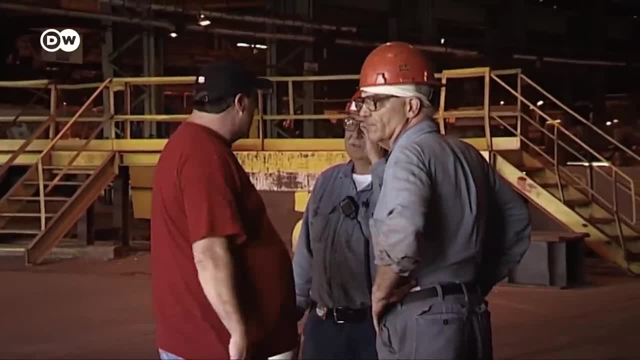 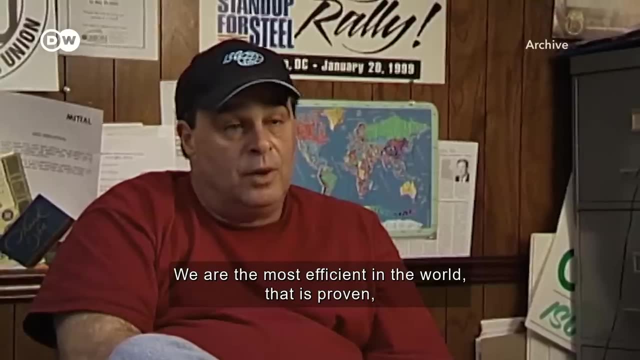 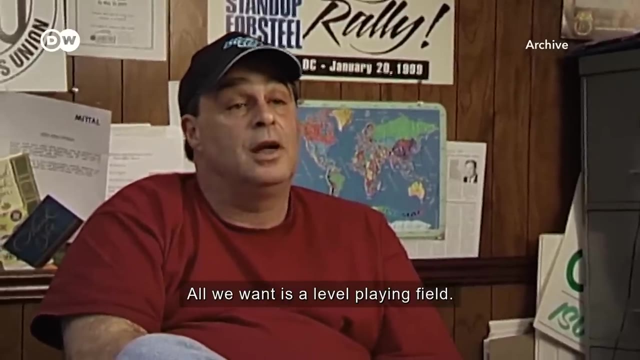 American steel workers feel cheated. Other countries have become more competitive than the US, But at what cost? We are the most efficient in the world. That is proven. All we want are the same conditions. You can't compare the US with Brazil or China or Indonesia, where there are no. 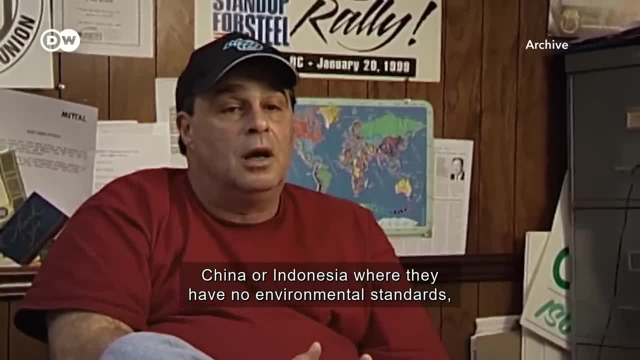 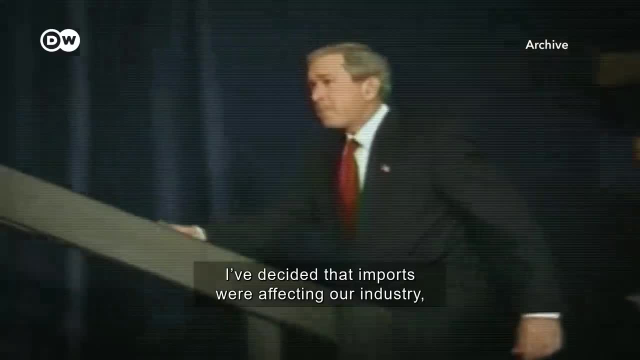 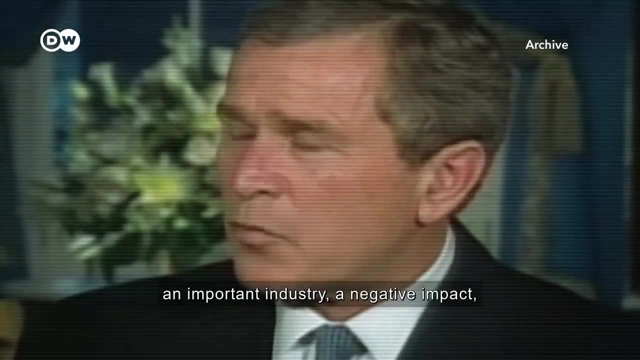 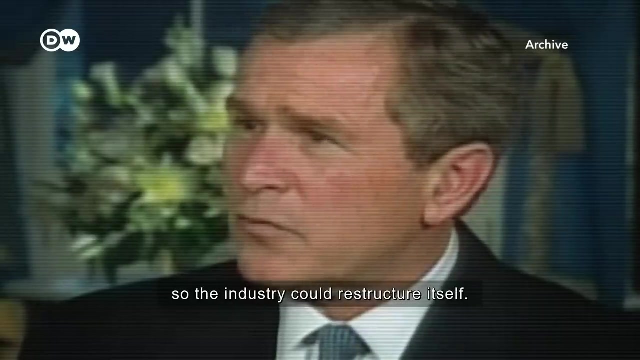 environmental standards, no health and safety regulations, Or they don't have no environmental standards, They have no health and safety. I've decided that imports were severely affected. our industry And important industries I have a negative impact. Therefore, we provide temporary relief so that the industry can restructure itself. 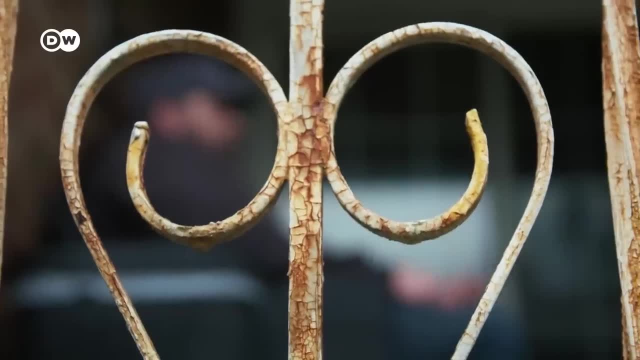 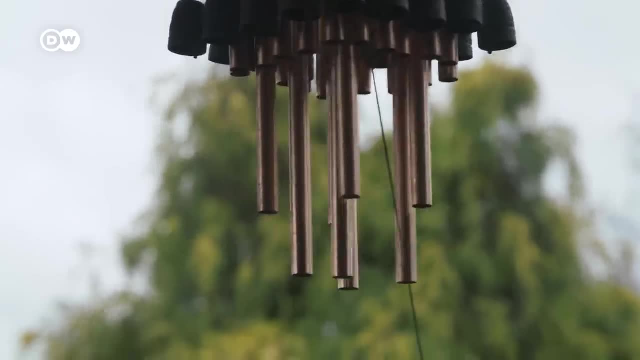 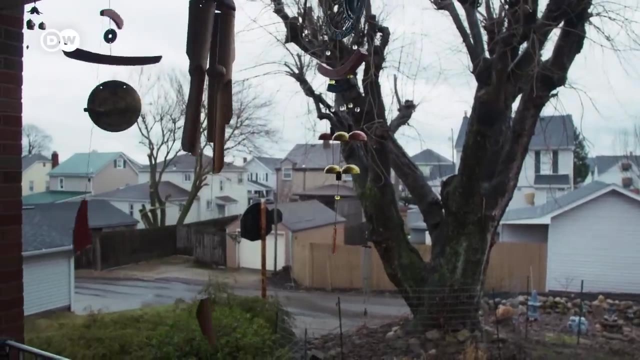 President Trump also imposed punitive sanctions. Now Joe Biden's promise to allow European steel access to the US market is a rousing distrust Of globalization as well. It's a very globalist administration. We were independent energy-wise and we gave it up in. 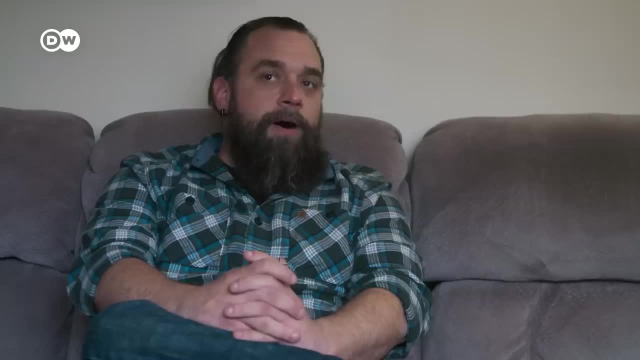 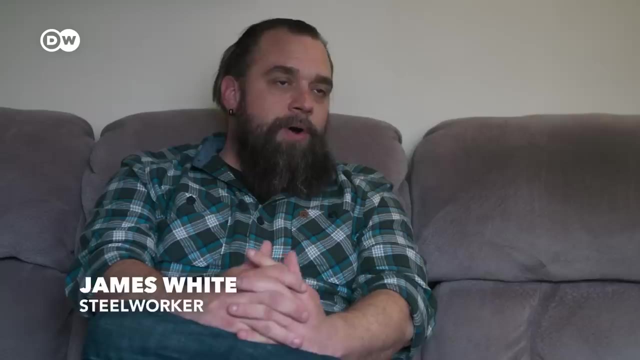 a couple of years, And all in the name of free markets and globalization. But that doesn't sound free to me And, don't get me wrong, that probably worked out For a lot of people with a lot of jobs in other parts of the world. 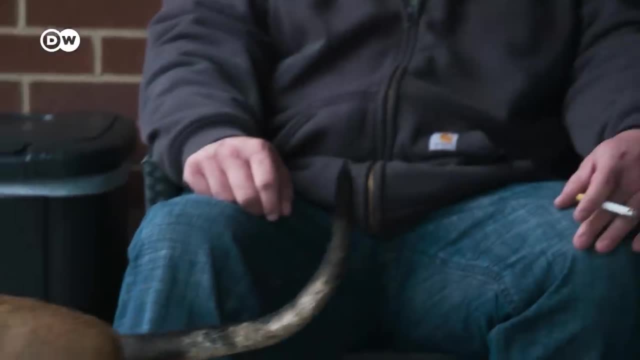 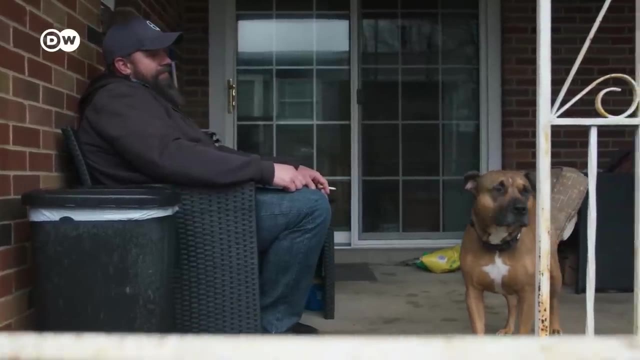 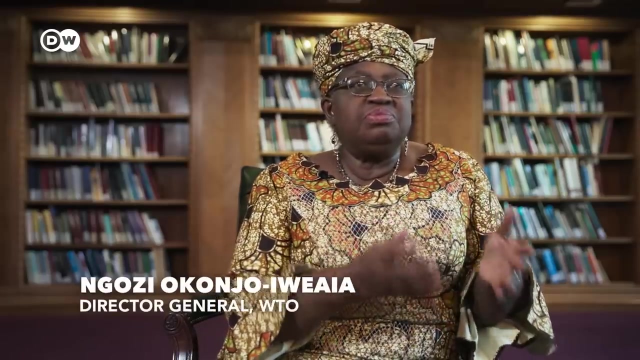 But it costs some here in this part of the world. Globalization has lifted a billion people or more out of poverty. Now, that doesn't mean that it's perfect. It's not. They're obviously poor people within rich countries who have been left behind. 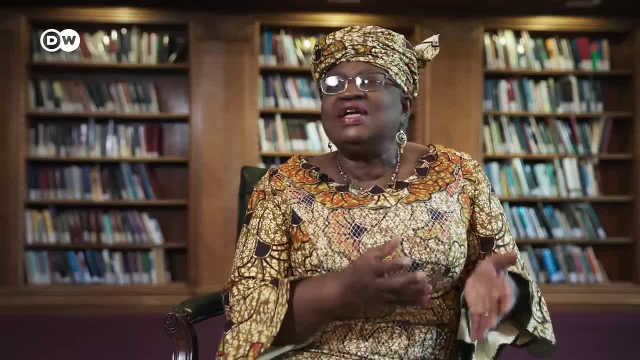 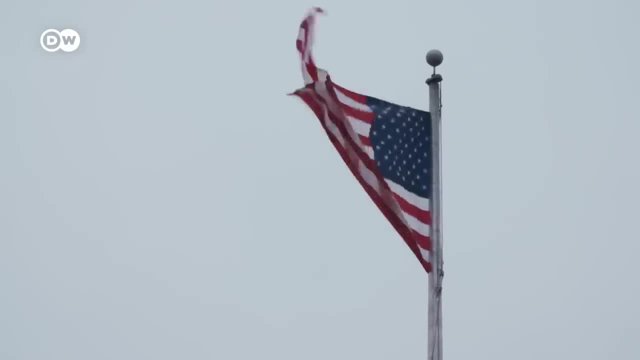 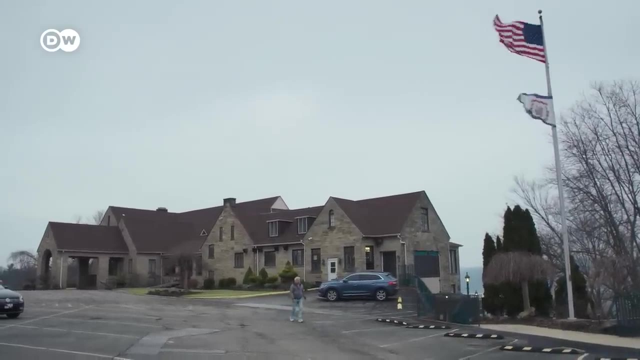 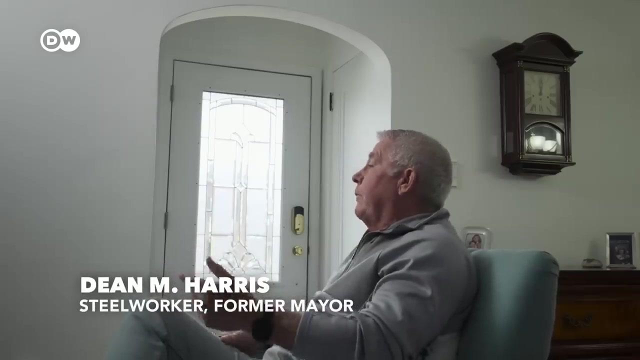 And in those cases their governments did not have the active money- labor market policies- to help solve the situation where they lost jobs. you know, there was a point in the 80s when national steel was was gonna close weirton steel down. we were division of national and I was laid off for 18. months, you know, and not just me, I mean. the whole town was laid off for quite some time. you know our town's a survivor, you know we'll get through it. in weirton fewer than 1,000 jobs remained of 14,000. there is room for new. 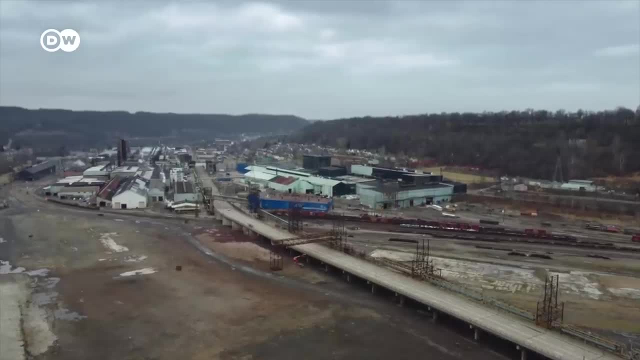 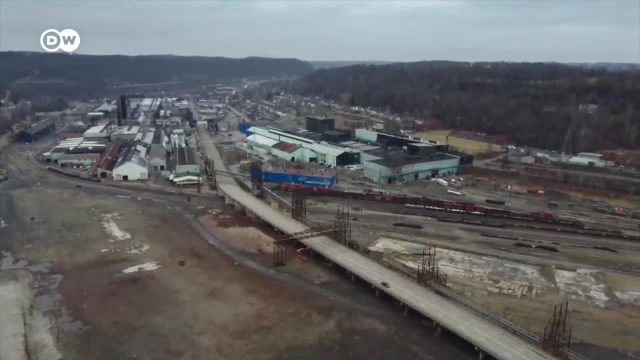 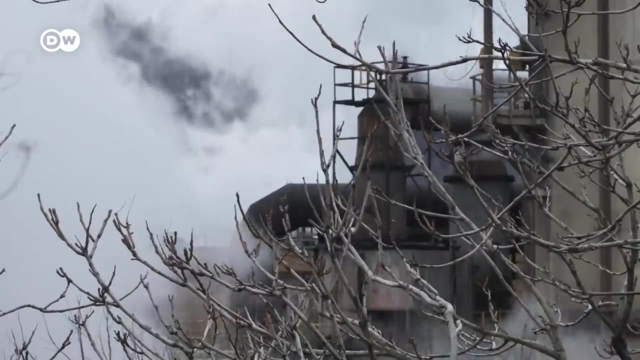 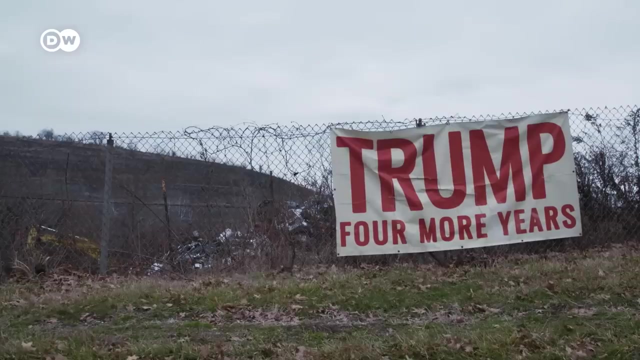 industries, but the America first approach casts a long shadow. instead of acting globally, people here act nationally. steel companies are reluctant to take advantage of the situation and they're not willing to take advantage of the opportunities offered by multilateral trade. they turn instead to government subsidies. in 2018, in a trade dispute with China, President Trump initiated new tariffs on. 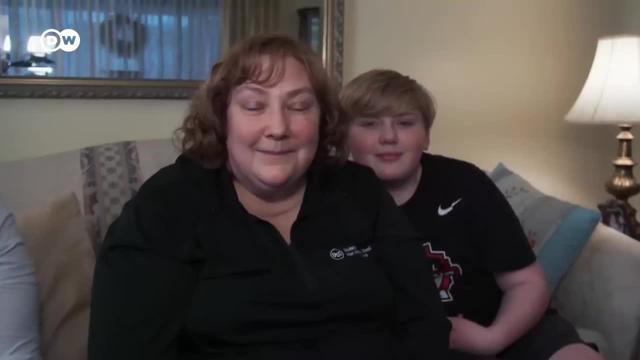 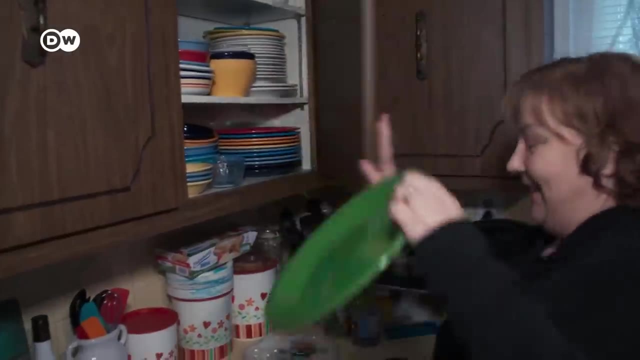 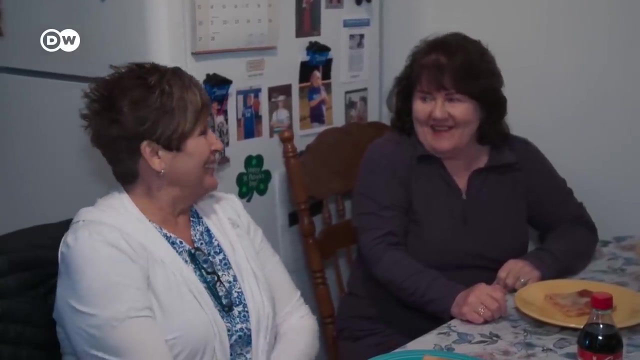 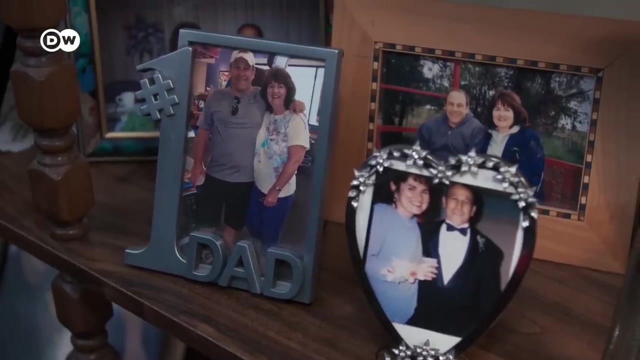 imported steel, winning plenty of support in weirton. it ended up helping us immensely both times, first when President Bush did it and then the other and then again when President Trump did it. it helped our workers to whether the the cheap steel that was coming in the Guerrera Thompson family has lived off. 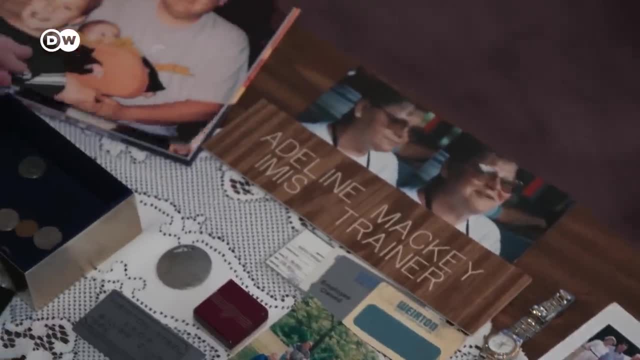 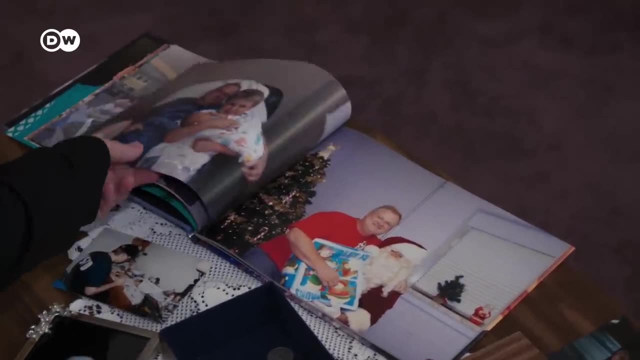 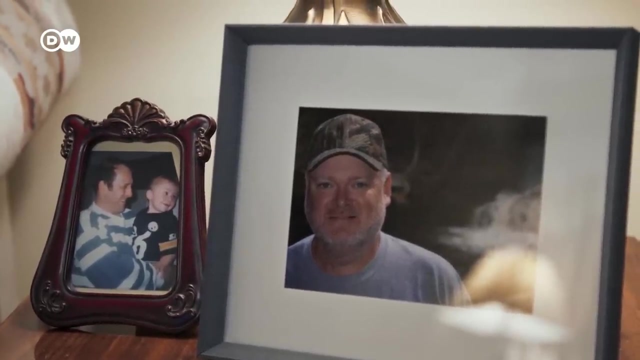 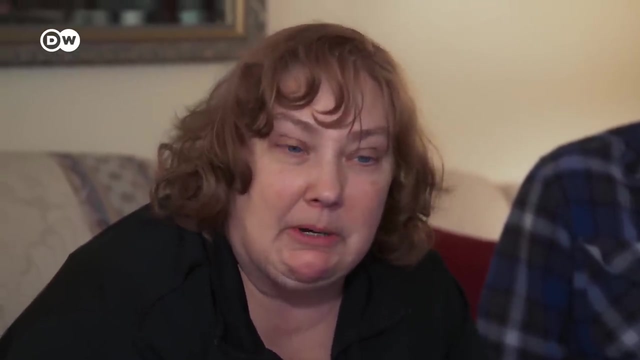 steel for generations, but Karen recently became a widow after her husband, Carl, a steel worker and staunch Trump supporter, died from covert 19 shooting. they now have two children and a six year old in the country. if anything he was proud of besides his children, it was to be a steel worker. 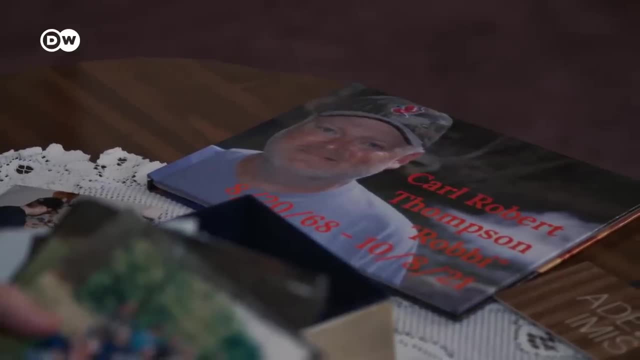 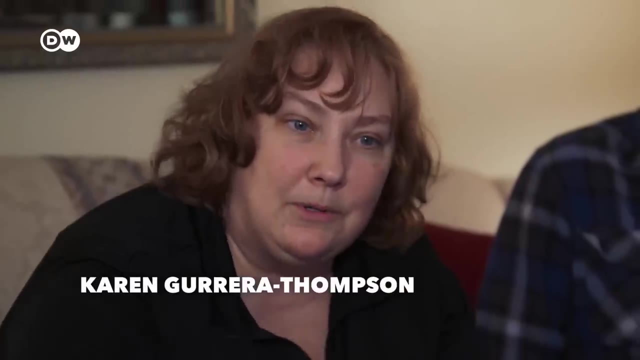 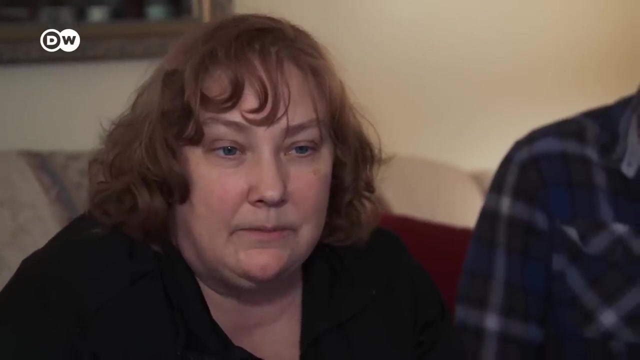 like his grandparents and his parents, but when he worked in the mills it was always pretty good for us. it was times of struggle, times of of of get you know when the mill wasn't doing so good. Less than 1,000 work there now. 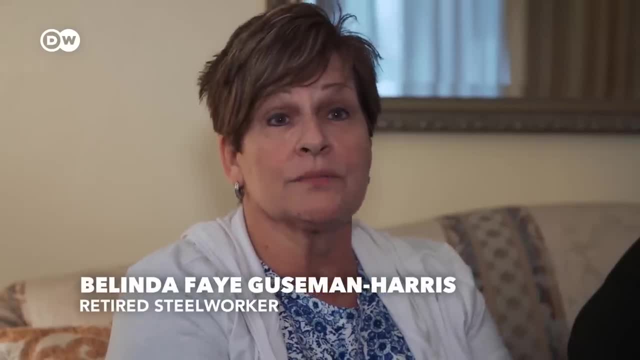 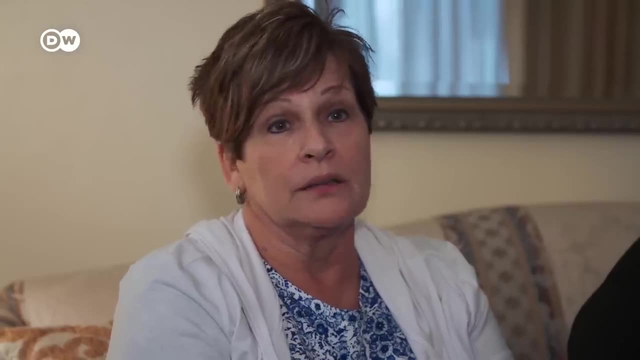 and it's from downsizing, you know, getting rid of jobs, farming out the work. You know they gave it away and wasn't going to pay top dollar when they could get it somewhere else a lot cheaper, you know. I think we need to be able to take care of ourselves. 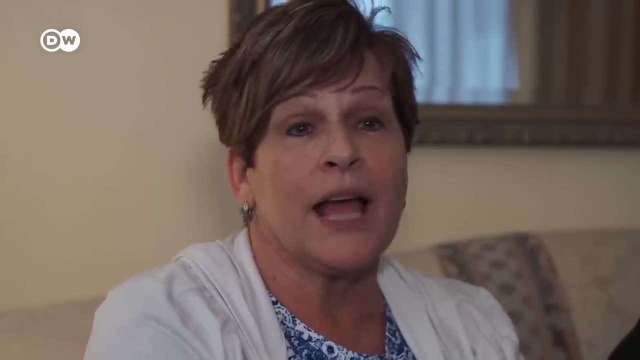 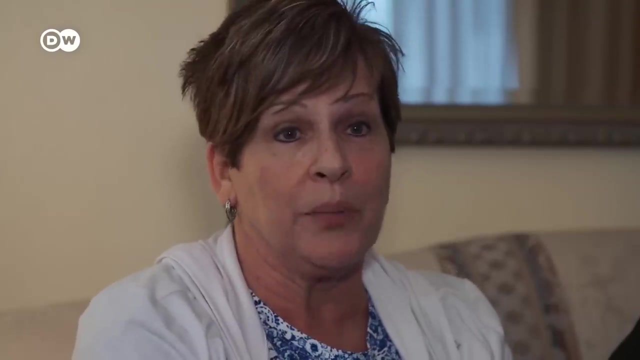 not just our country. Every country should be self-sufficient, because I don't see China selling us armored plate to build tanks for another world war, if God forbid that happens. I just watched it for years. I'm like we're never going to be able to protect ourselves. because we don't have the manufacturing to do it. The way China conducts business with the rest of the world, it's the same thing: Everybody's out for their national interests. So once the globalization gets so big, then it's inevitably going to contract. 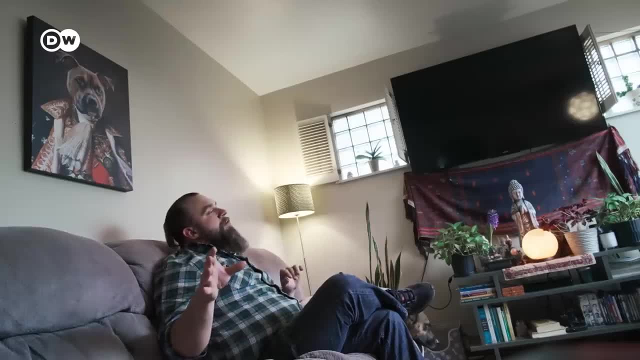 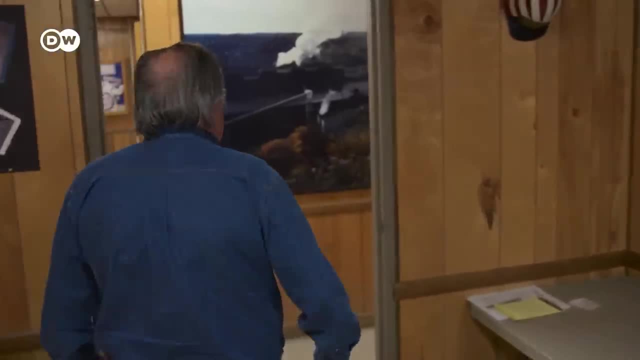 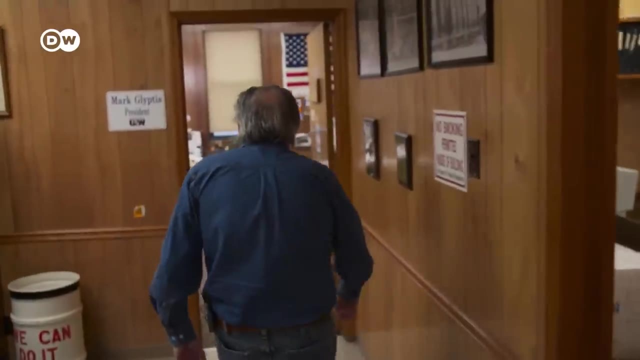 once people start feeling a little bit nervous about their neighbors growing too strong, growing too wealthy, then we're going to start worrying about our own national interests. Our government betrayed America, betrayed the American steel worker, and they'll do so again today. 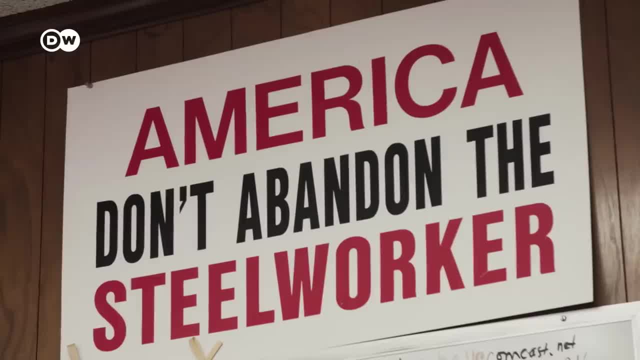 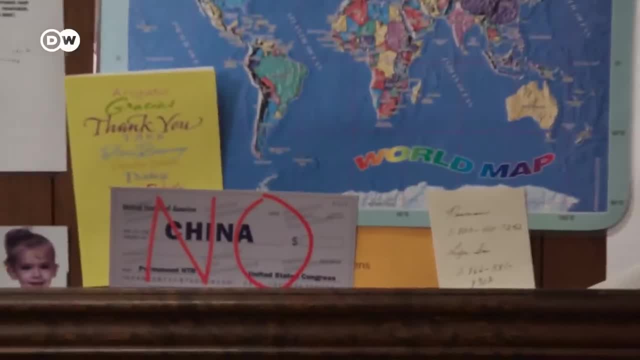 We just had a bridge collapse in Pittsburgh. We can't even get the steel to rebuild the bridge from America. You have to go overseas. and China is one of the major culprits. They have built so many steel mills. they don't have the same set of rules that we have. 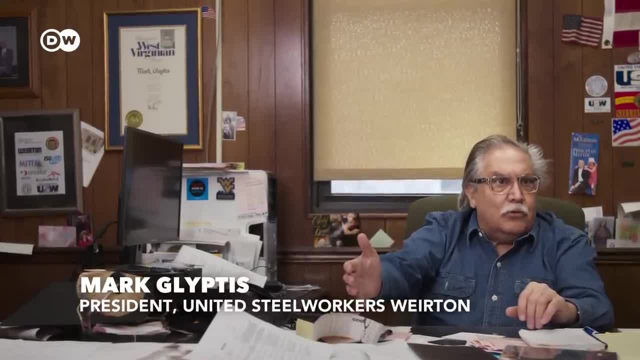 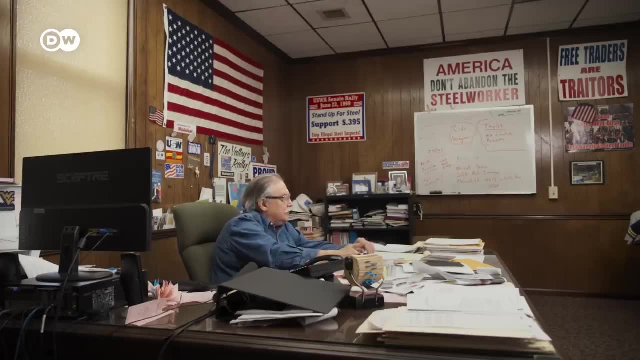 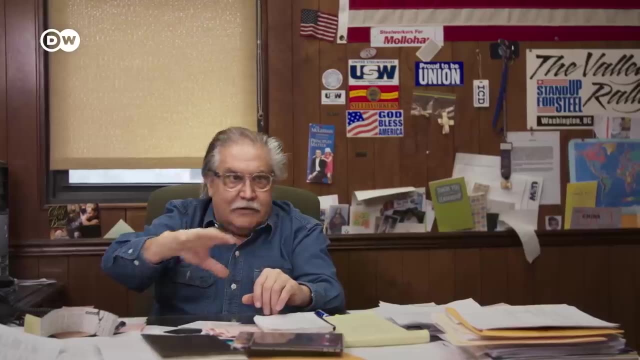 They don't care about their environment, which, environmentally, all countries ought to be required. all mills ought to be required to have a clean process. But China, it's a filthy country, okay, And it's a dirty country. They don't care about their environment. 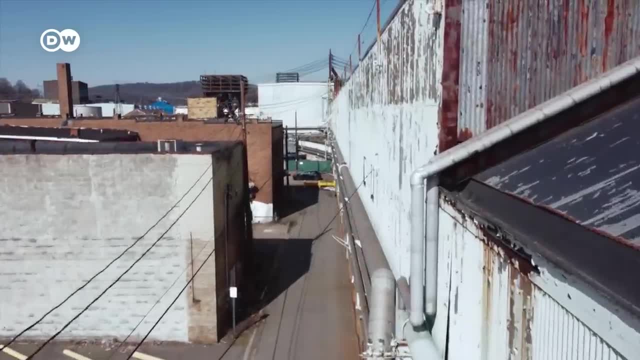 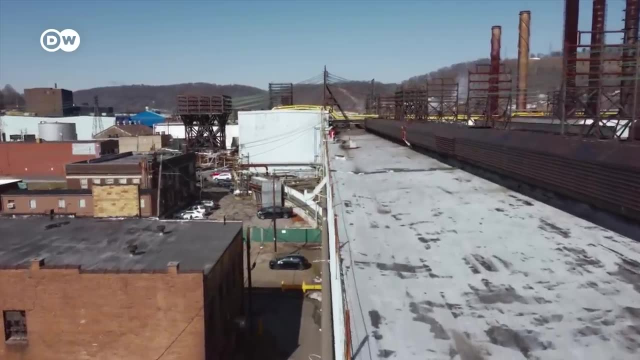 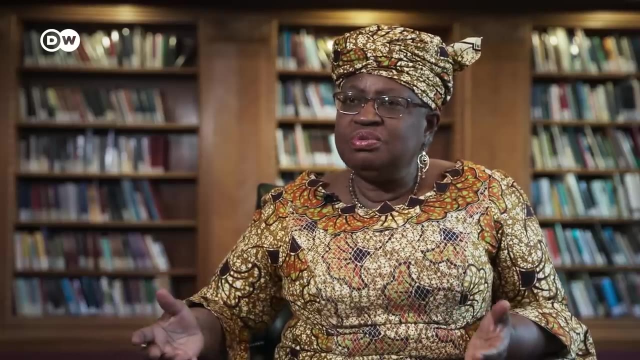 They don't care about the people. So many countries are coming up, maybe some of them faster, some of them not so fast, so let's not exaggerate. But you know China for sure, And some of these developments were not really thought through. 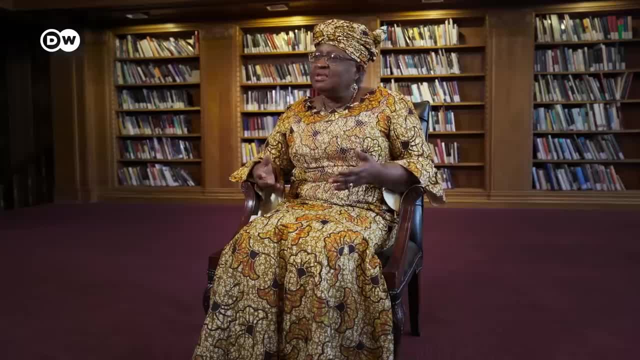 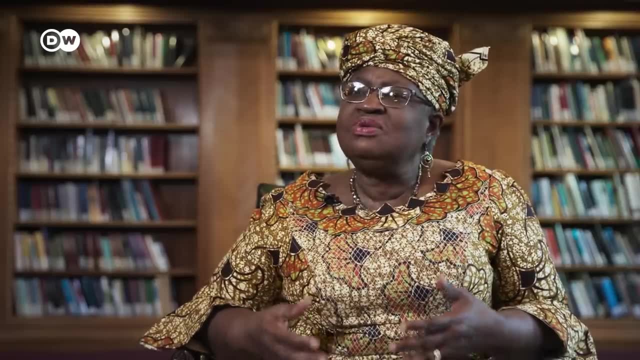 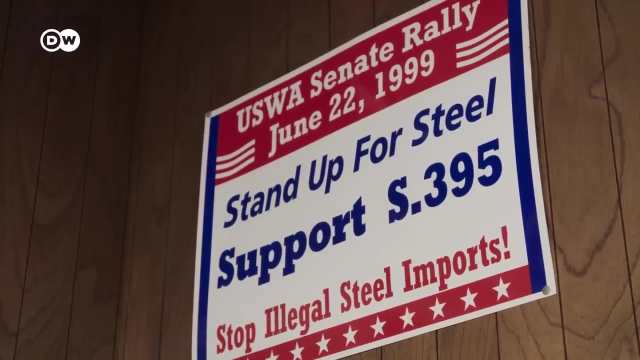 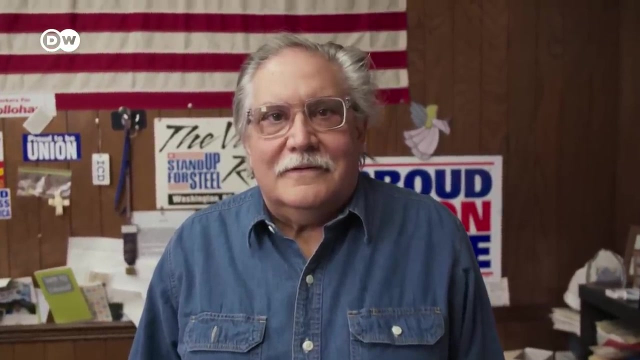 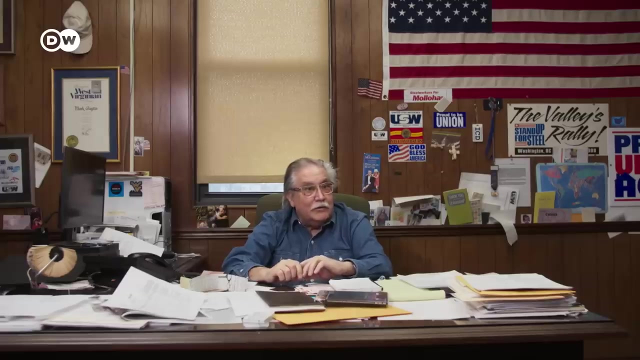 so that the instruments we have, the rules we have, are a little bit outdated. They do not catch some of these developments. So that's absolutely right. I was a strong advocate to get out of the WTO trade organization. Ultimately, you're not going to be able to do it by yourself. 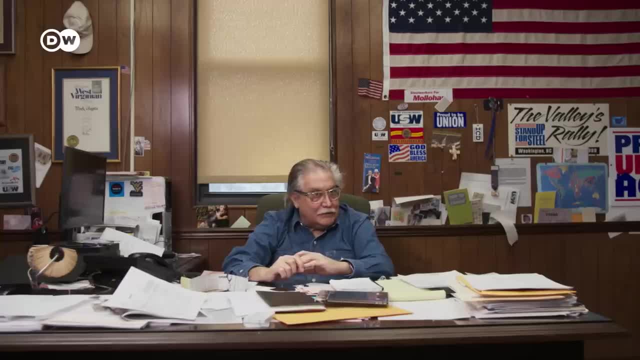 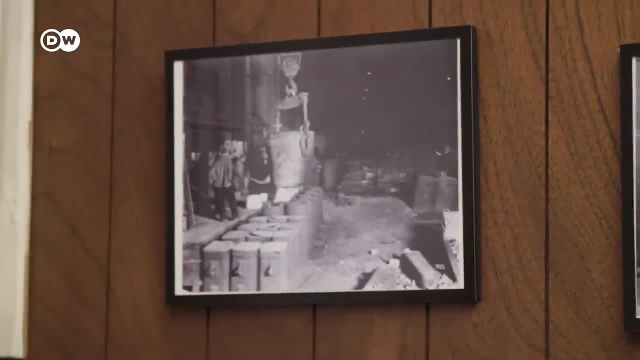 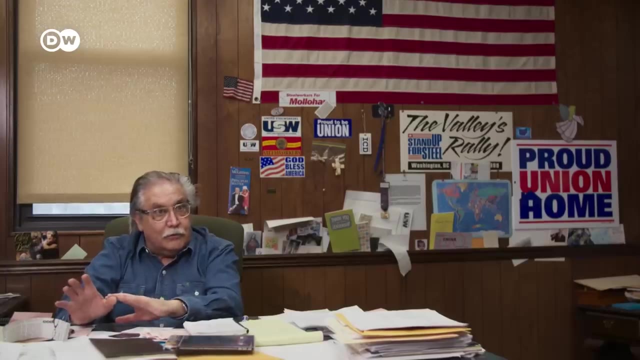 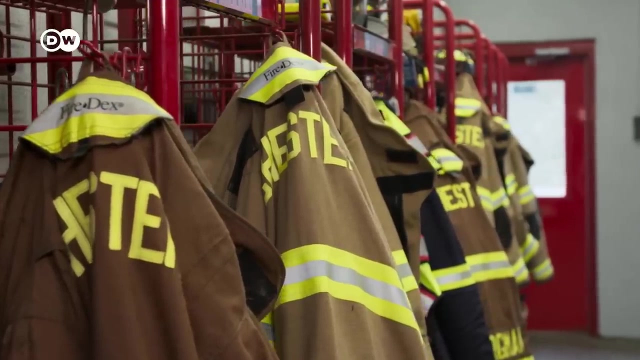 Okay, Because there has to be exports. There has to be a system of trade. Okay, On a global basis, But you can't protect certain industry within a global economy. Still should be one of them, But why subsidize a mass market product like steel? 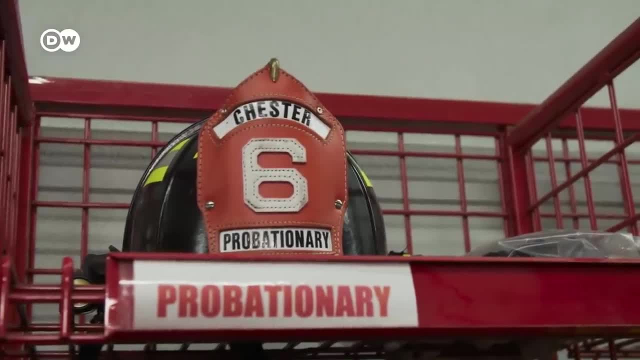 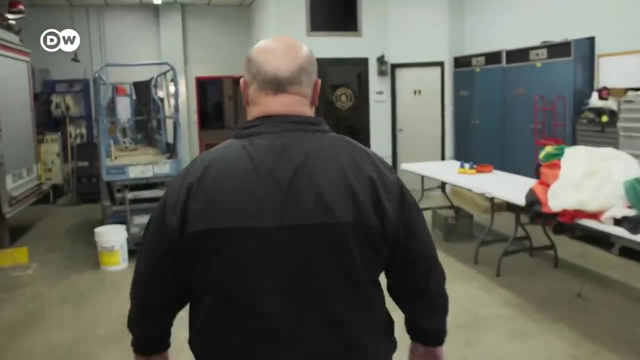 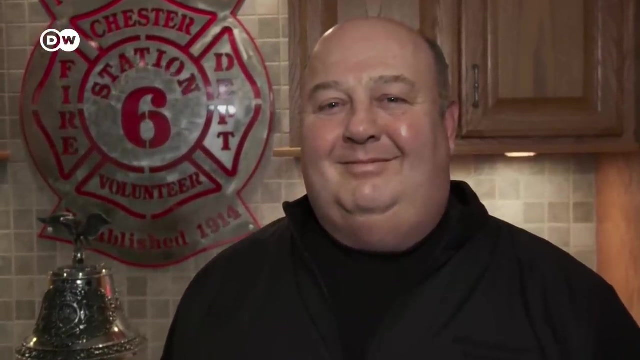 when it has no chance on the global market. It's time for a new approach. Enter into specialty and niche markets is a direction. They kind of had that with tin plate, that WTO. It was a global reduced tin plate they made years ago. 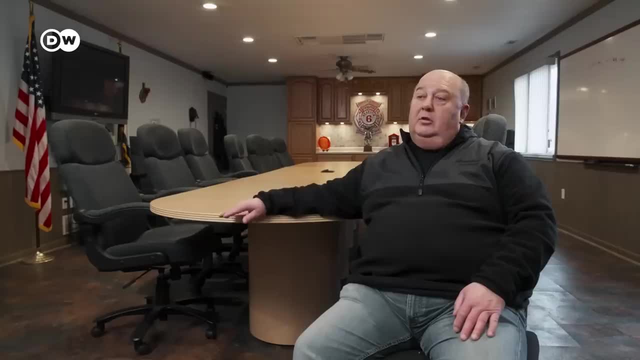 It was the best in the world And that's what kept Weirton Steel afloat. And even in hard times Weirton Steel could stay ahead of the other steel mills in this country because of their quality tin plate that they put out. 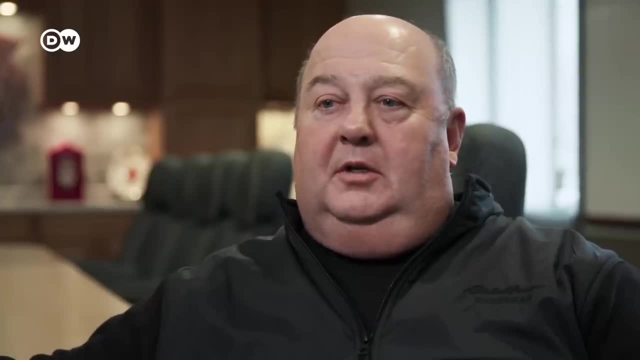 It is a global market out there And to compete in the long run it's just not selling your product within the 50 states. We're going to have to be able to go out there, to go into that worldwide market And whether you like them or not, the crossroads end up at the WTO, So we've got to be able to play the game as well as everybody else. Washington DC: Home to those responsible for subsidies and protectionist tariffs. The people governing protect, not just the steel industry. 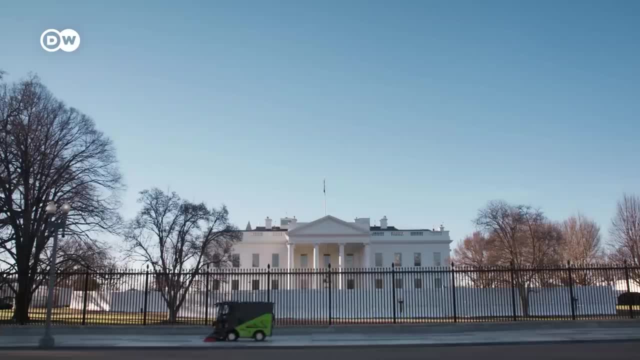 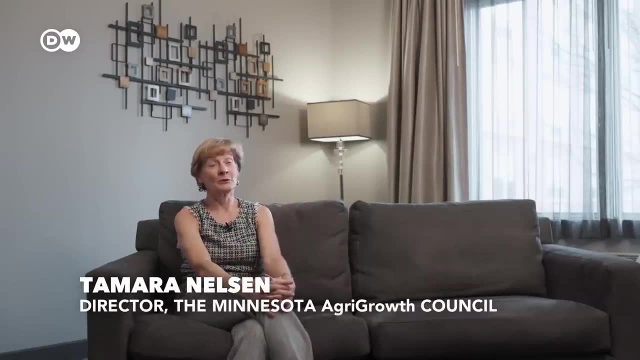 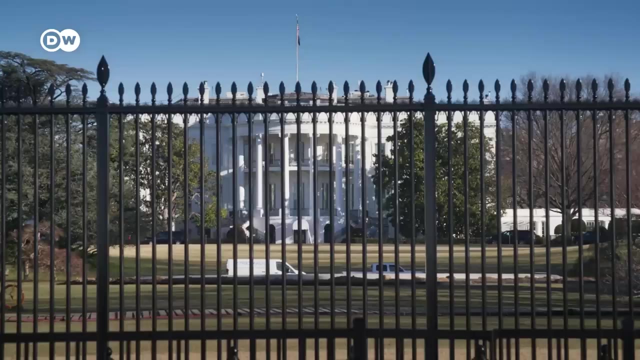 but the agricultural economy as well. And then the hammer really came down when President Trump rewarded agriculture by giving tens of billions of dollars to American farmers, essentially to offset their trade losses. Trump somehow came up with a way of distributing subsidies to American farmers. 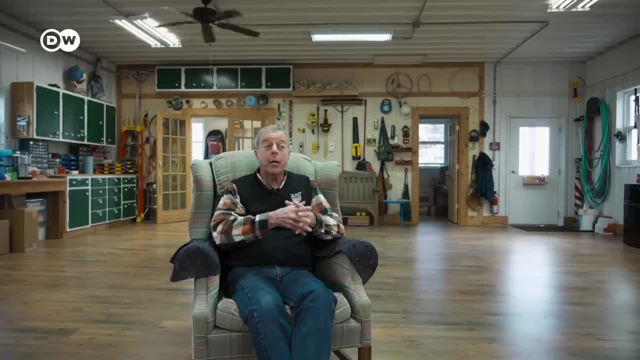 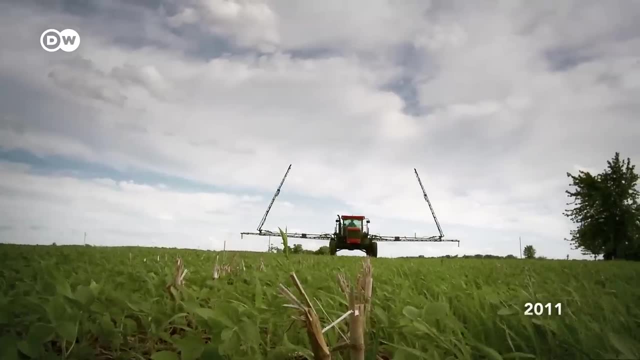 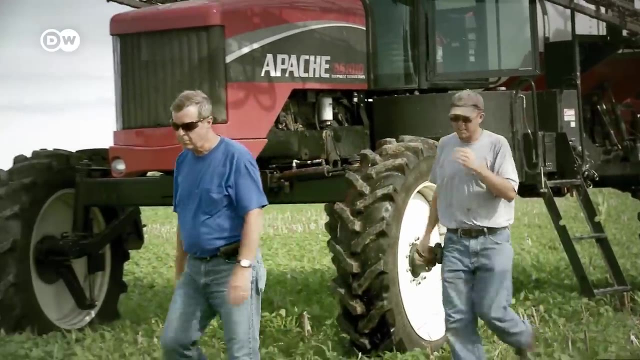 He said: you know we're going to be able to give to farmers without going through Congress. We just get cheques in the mail, so to speak. 2011,- Illinois, the farm of John and Aaron Phipps. Even then, America's farmers benefited from farm subsidies. 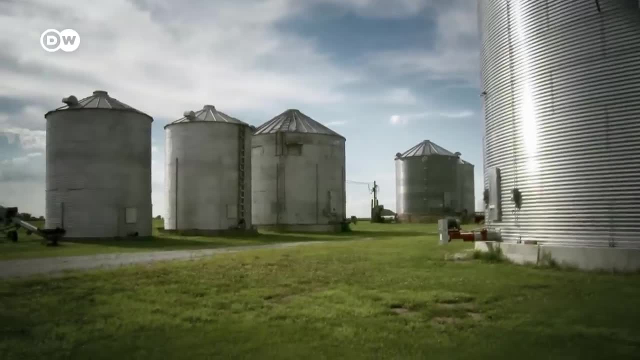 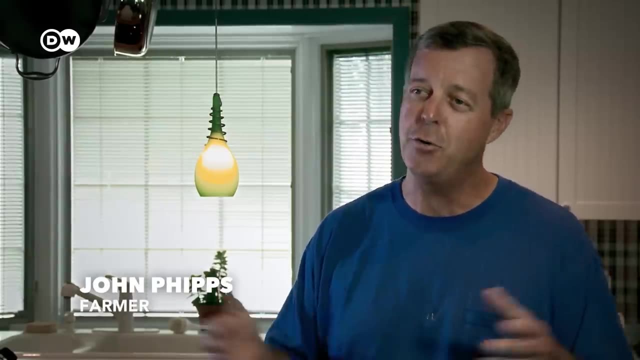 Agricultural subsidies to be morally irresponsible And I mean there is simply no justification for it. I just get that for having a body temperature somewhere close to 98.6.. Not because I do anything, not because I'm worthwhile or any deserving factors, simply because I have those acres. I get $24 for every acre. Well, once you hand that $24 out to every farmer, then the first thing he thinks of is: I know I can afford to spend $24 more to bid on this extra 200 acres and make my farm 200 acres larger. 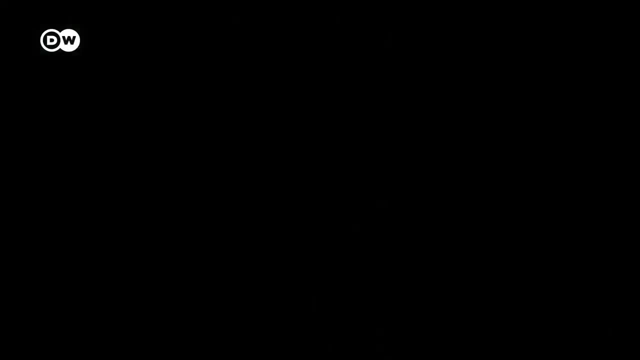 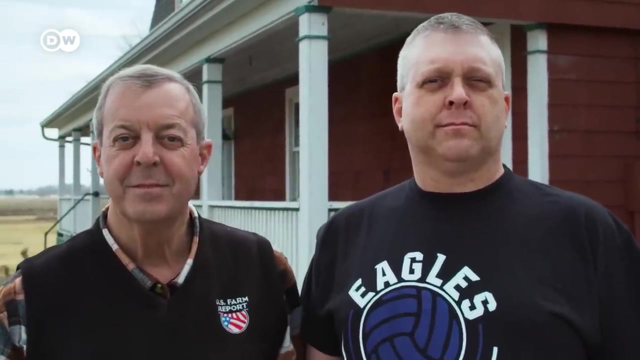 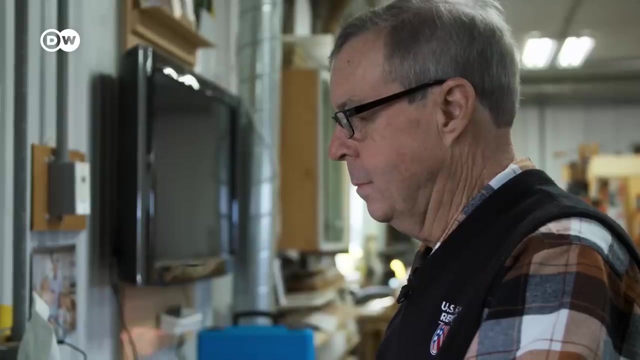 because that's what we're all doing. We're trying to. We're trying to grow. Welcome to US Farm Report this weekend. I'm Tyne Morphin and here's what's in store: Just moving from field to field. 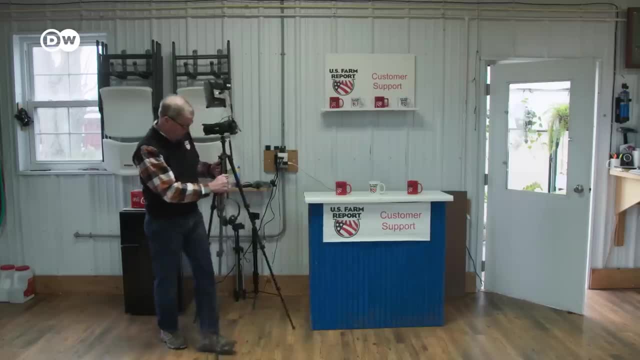 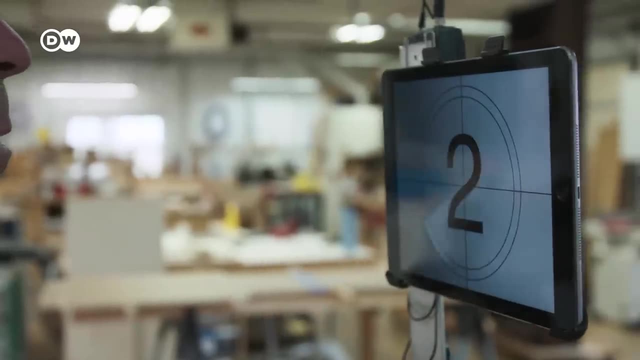 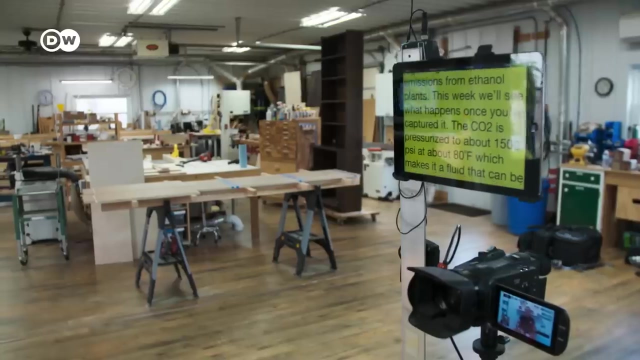 John Phipps is now retired. He's a commentator for US Farm Report TV, a weekly TV show. Last week I began an answer to a question- The answer to a viewer- regarding carbon dioxide emissions. I have people who just can't stand me. 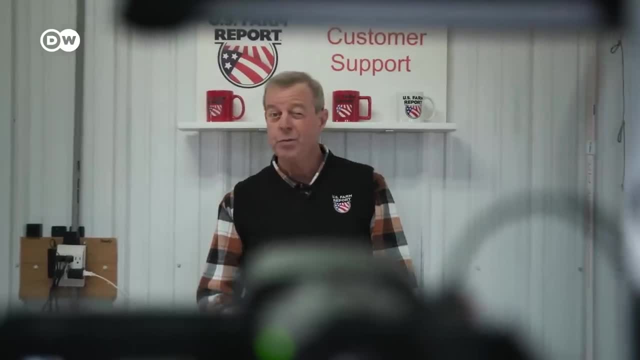 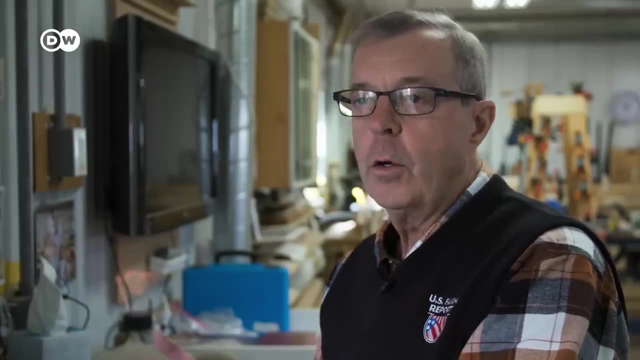 And actually they're my favorite. And the other half are people who just got up early in the morning- generally on the stations early in the morning- and they're looking for something to watch and they've gotten hooked on what's happening in agriculture. 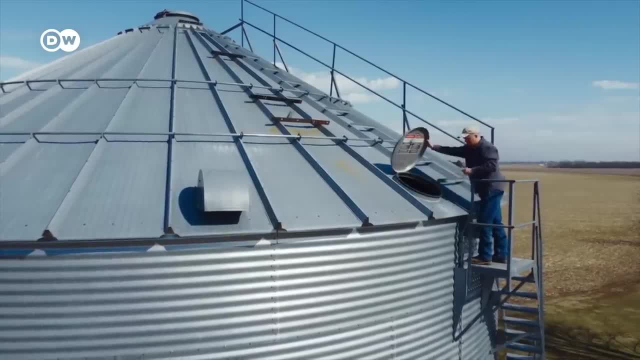 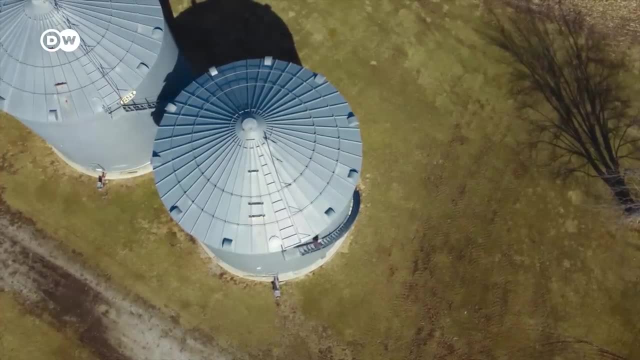 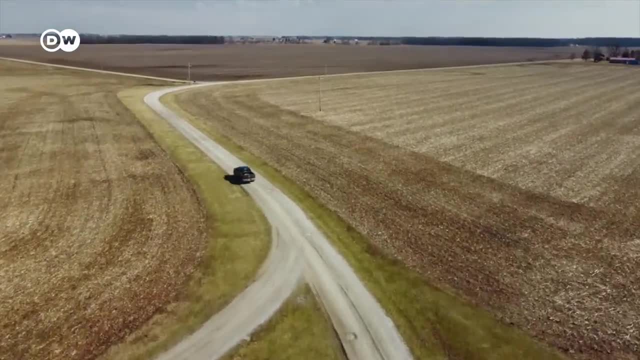 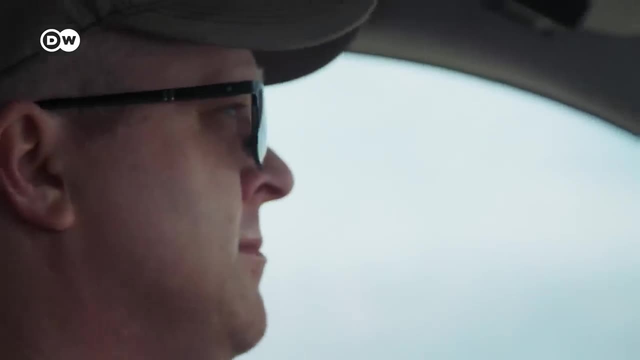 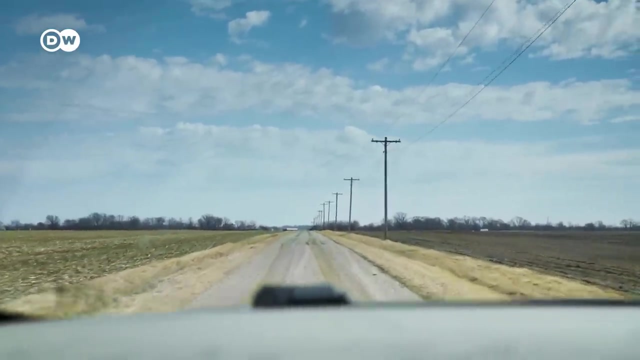 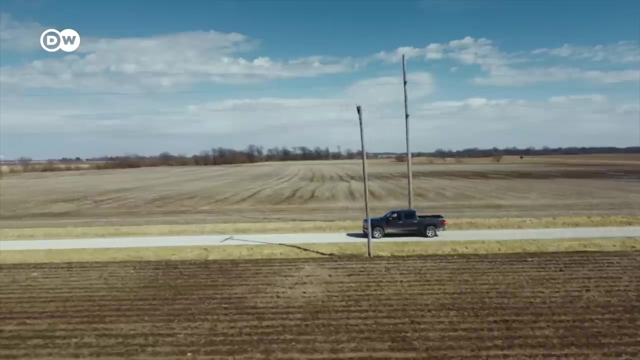 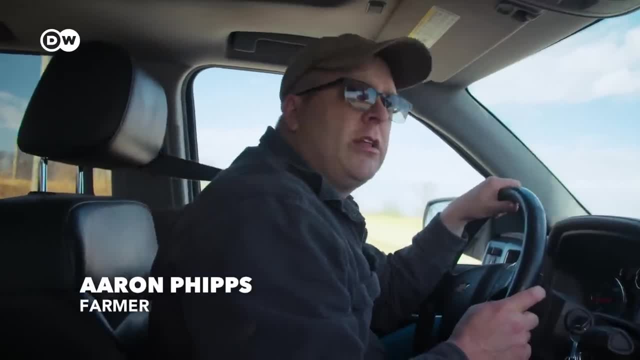 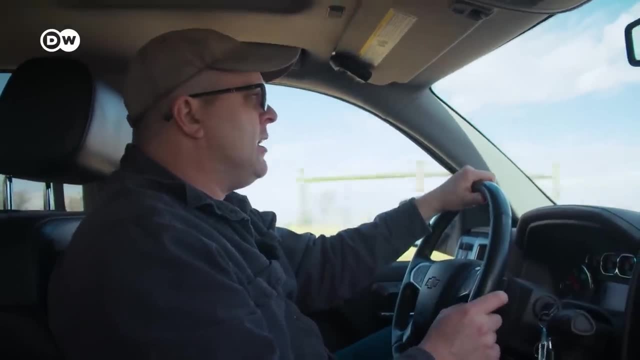 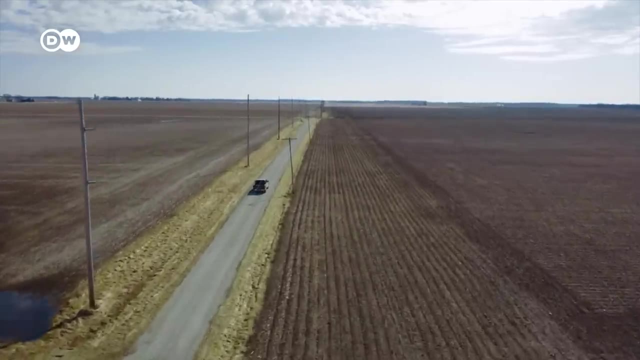 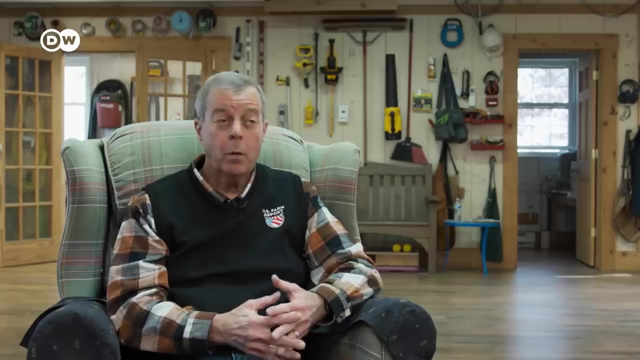 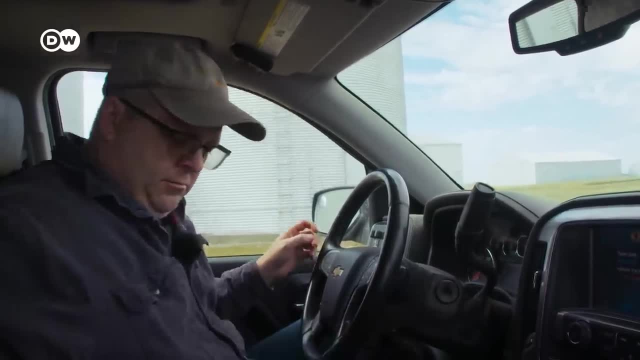 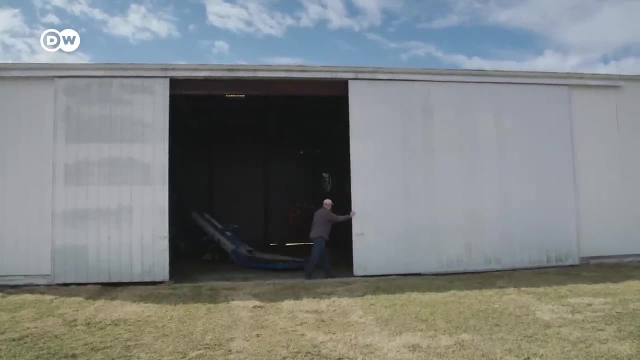 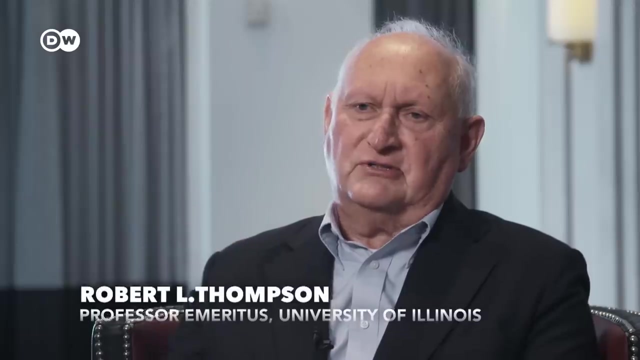 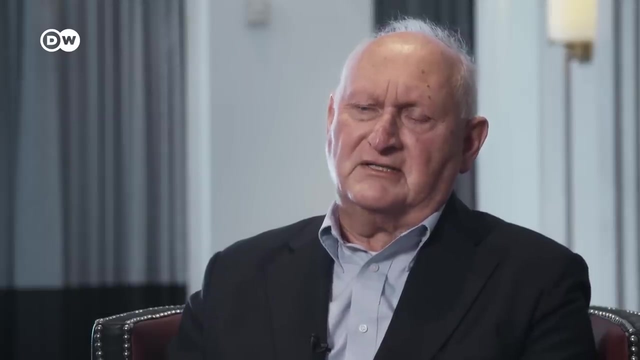 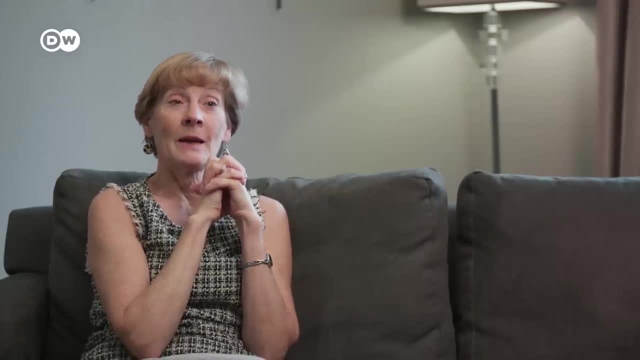 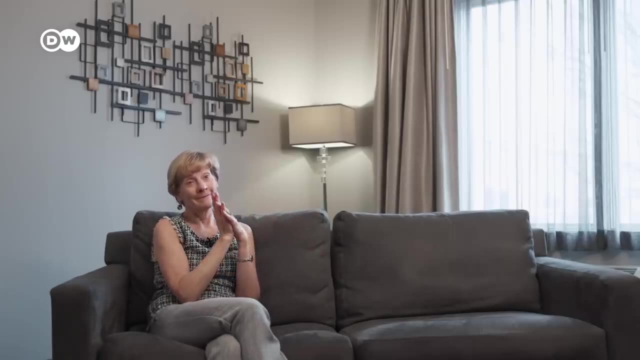 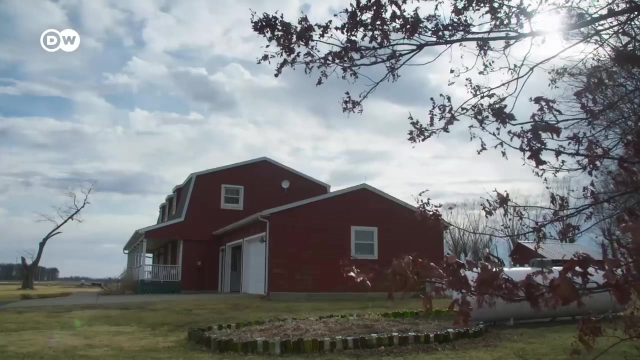 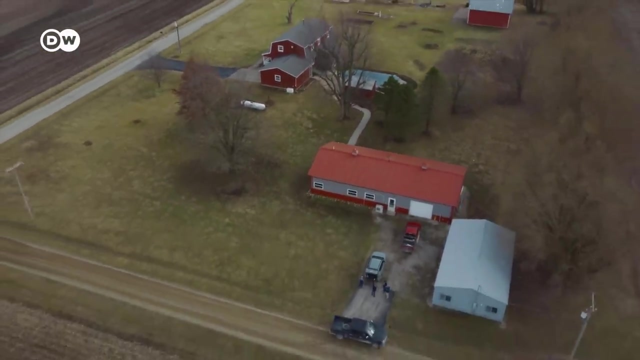 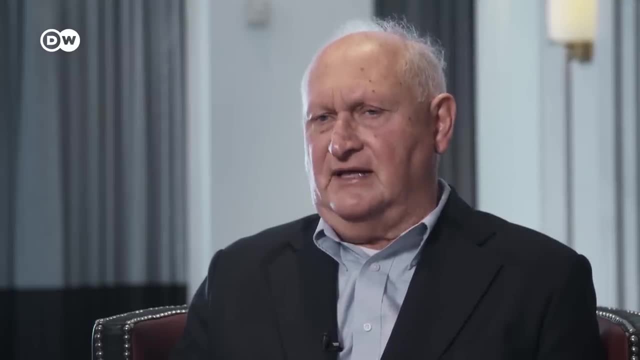 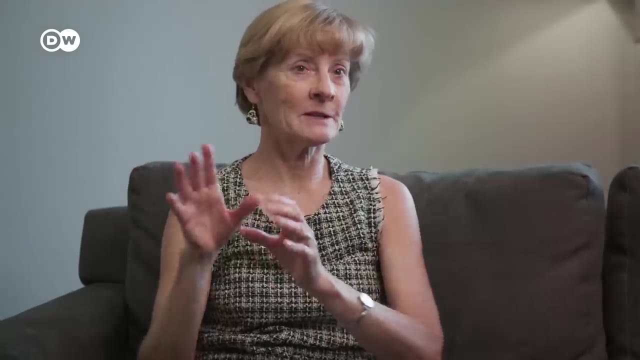 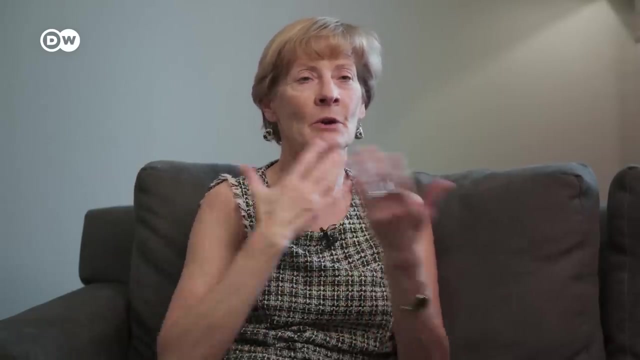 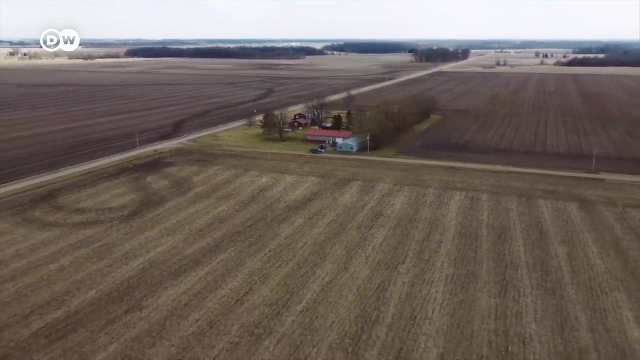 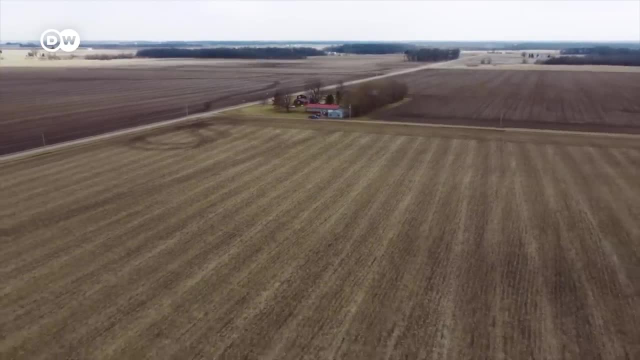 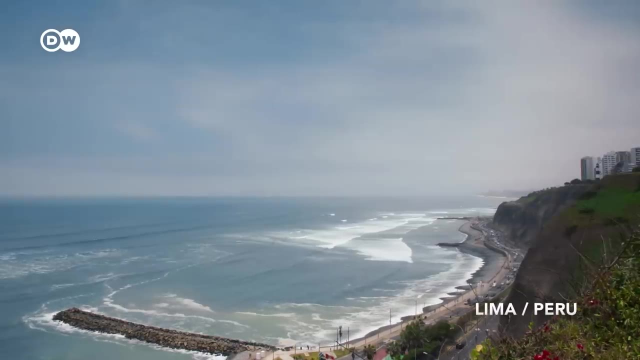 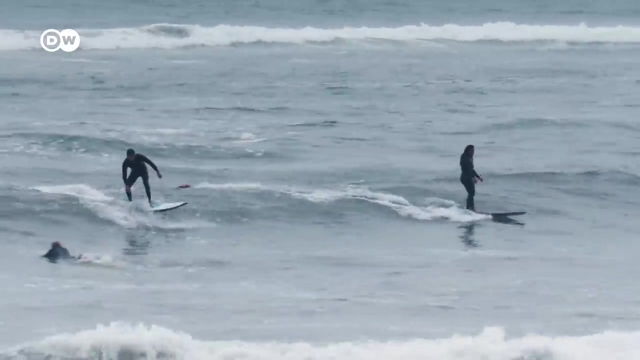 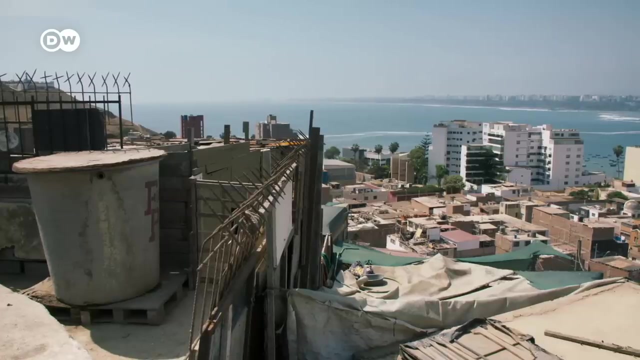 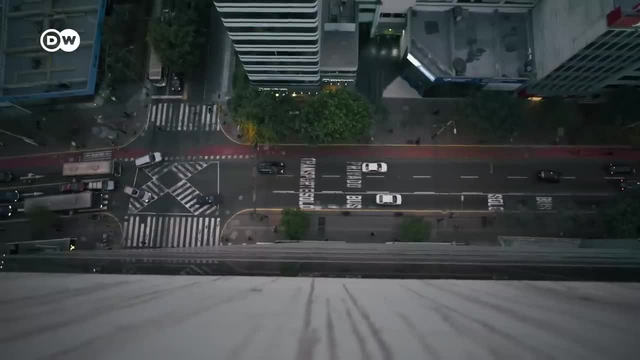 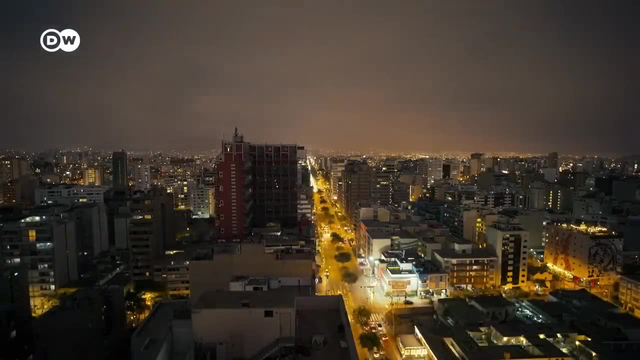 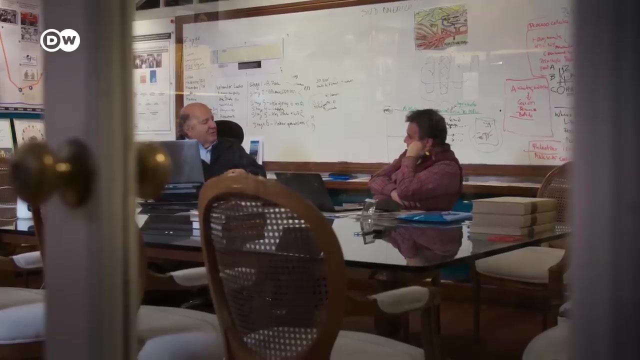 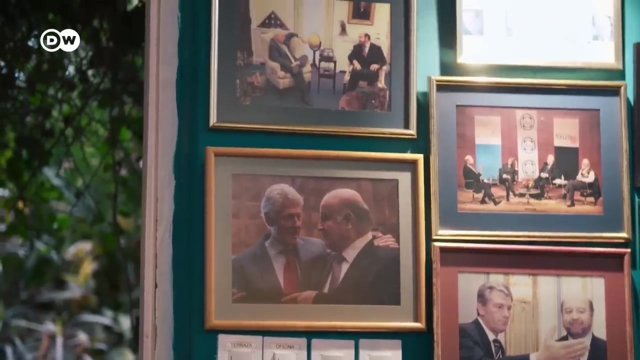 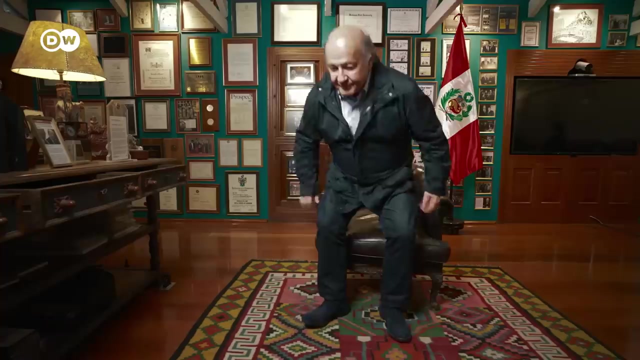 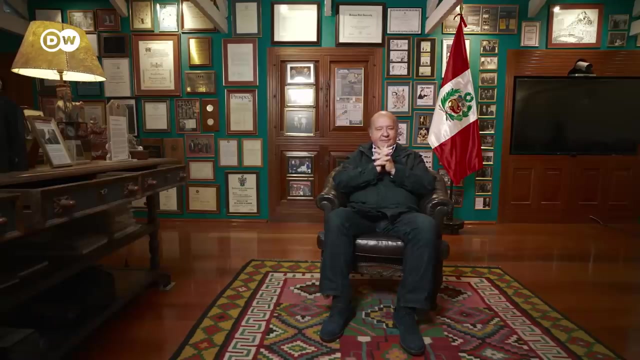 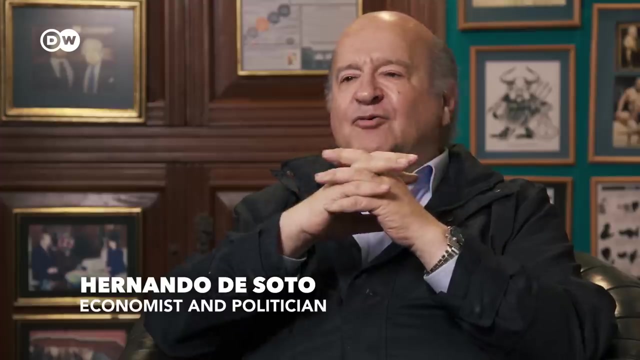 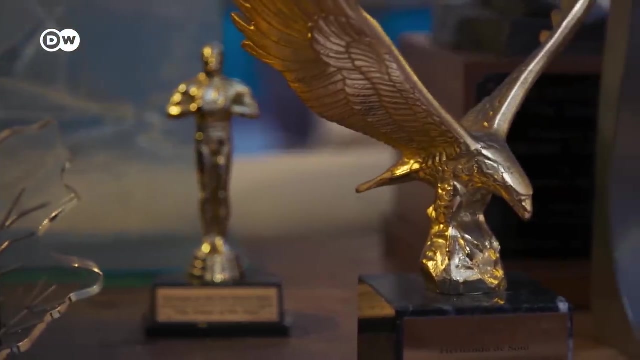 ¶¶, ¶¶, ¶¶, ¶¶. Even though official statistics say that Peru is probably at the end of the worst of all developing countries, the fact of the matter is, we're probably even worse than the statistics say. Between 2016 and today, we have had four presidents. 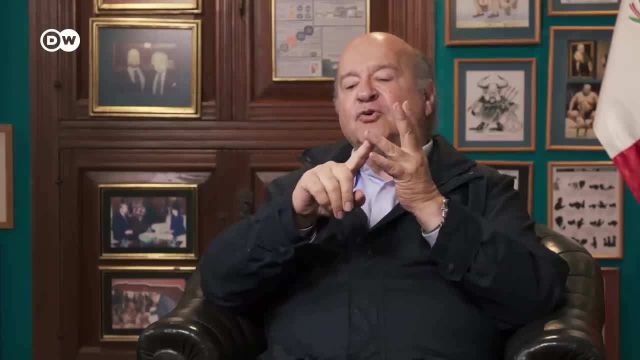 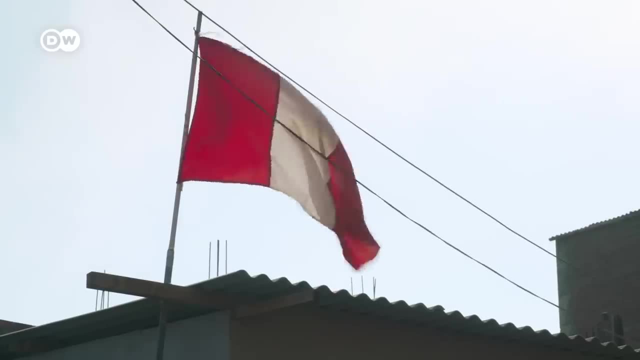 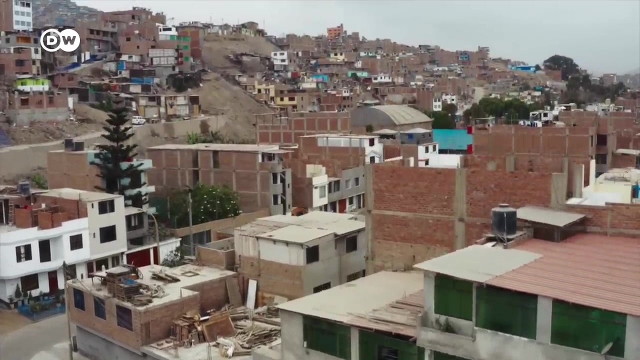 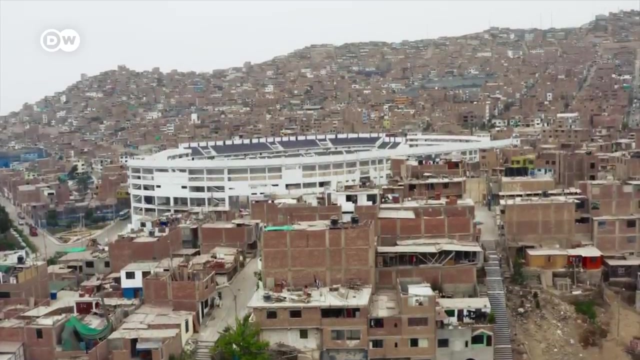 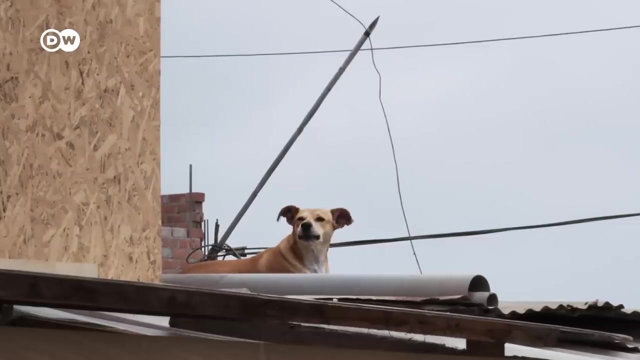 Four presidents ¶¶, And one, two, three parliaments, Because the system has collapsed. Peru has one of the highest COVID-19 death rates in the world. The pandemic helped the informal economy expand even further. ¶¶, ¶¶, ¶¶. 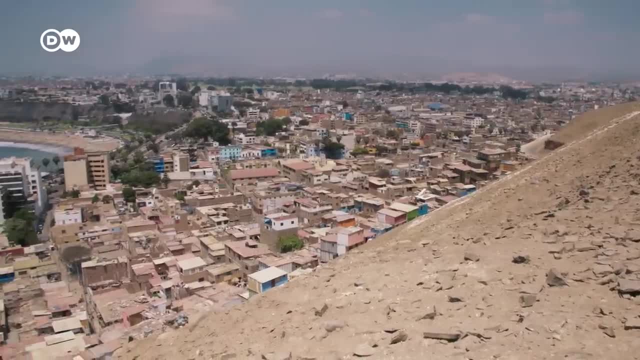 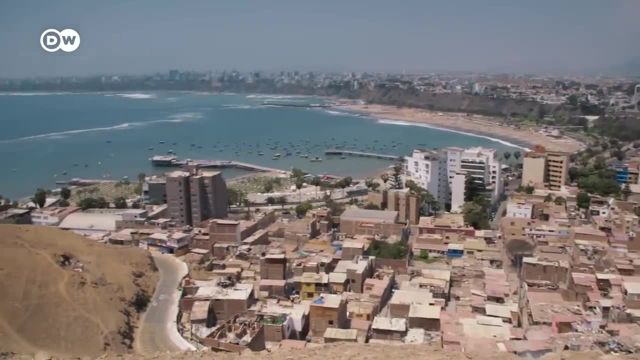 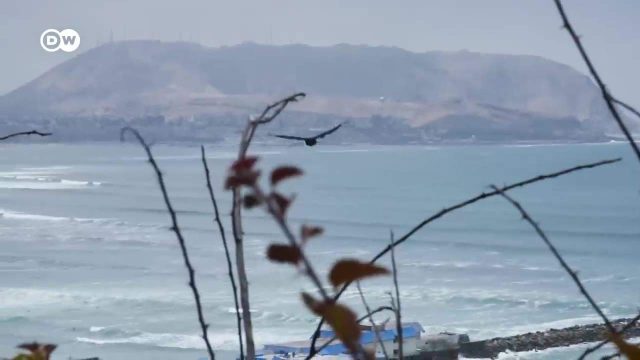 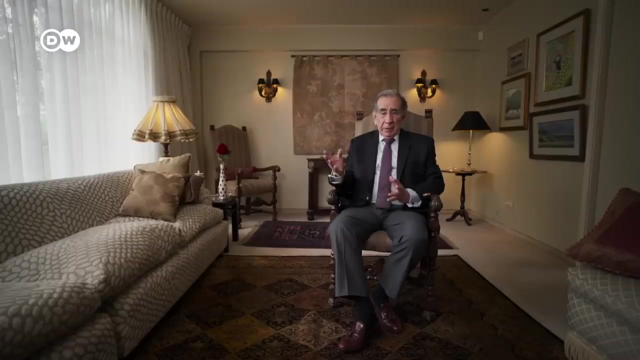 ¶¶, ¶¶, ¶¶, ¶¶. The country is rich in raw materials, but they're mined mainly by foreigners, particularly by the Chinese. ¶¶, ¶¶, ¶¶, ¶¶. We have been mining lithium in mines near Chile, in the south of the country, for many years. ¶¶. The product has great potential. Lots of countries are interested in it. China, for example, is the first country that wants to benefit from it. China is investing in all of Latin America, including Peru. The Chinese want to build a port in the north, which will help them expand in the Pacific. 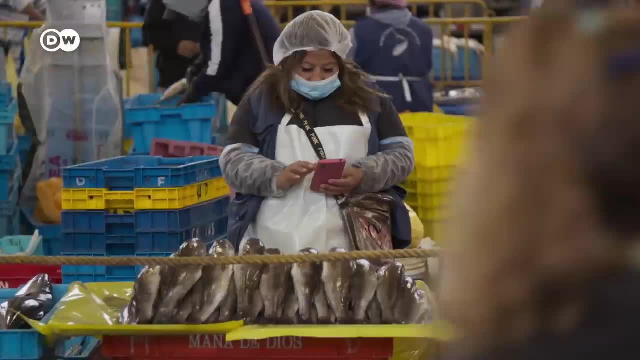 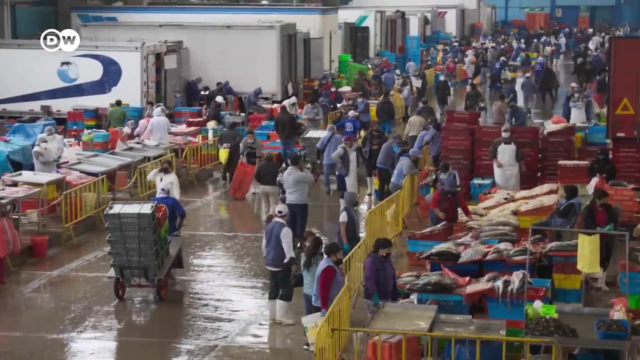 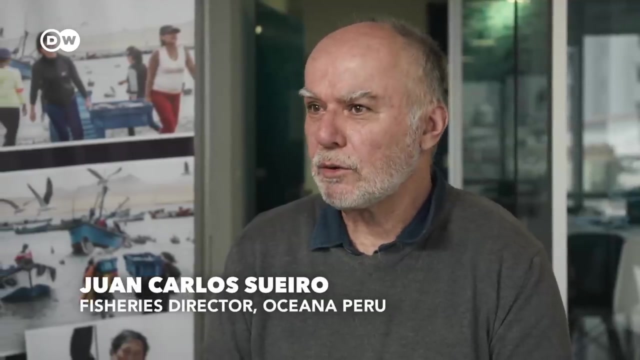 Fishing is also crucial to the local economy, But so far there's been very little foreign investment in major fishing companies, not even from China. China is investing massively in mining and hydrocarbons, as well as in other sectors of the economy, but not yet in fishing. 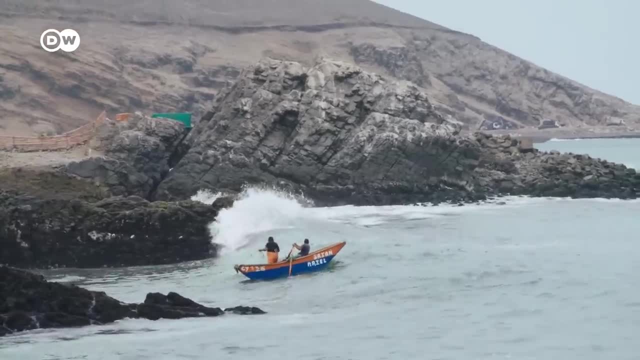 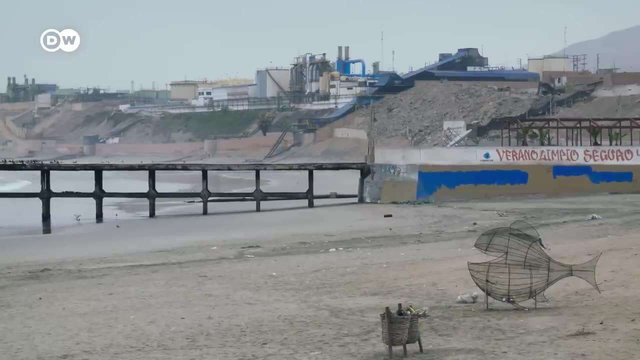 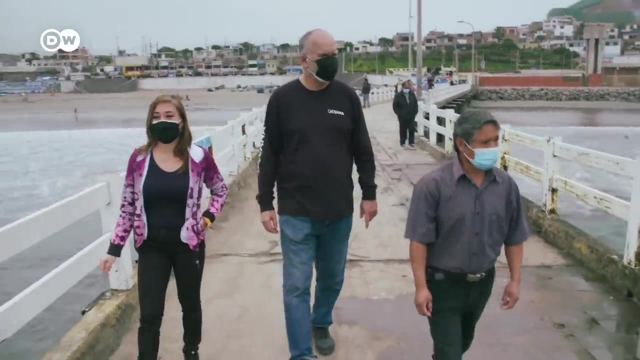 The small town of Chancay depends on fishing and on a fishmeal factory. About 90 such plants can be found along Peru's more than 2,000 kilometers of Pacific coast. Miriam Aceh and Juan Carlos Suero know the area best. 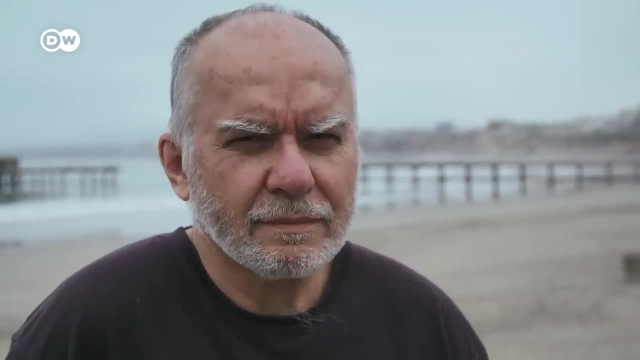 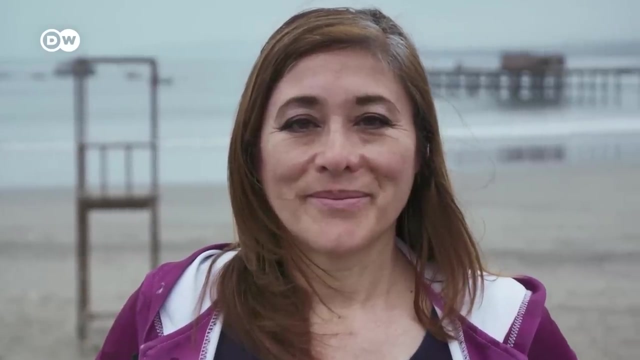 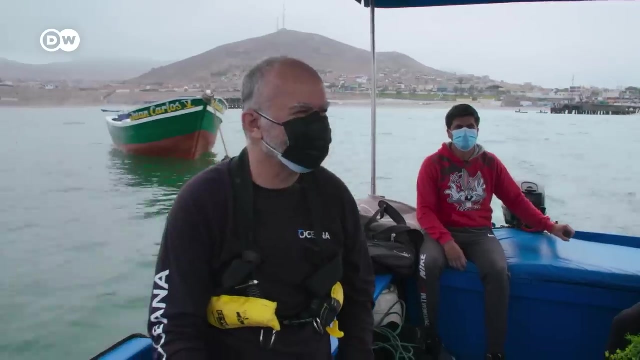 Juan Carlos Suero is an economist and fisheries expert for Oceana, an international marine conservation organization. Miriam Aceh is a member of the Oceana Association of Fisheries. Aceh is fighting the construction of a megaport. Industrial fishing is on a break. The season won't begin for another two weeks. 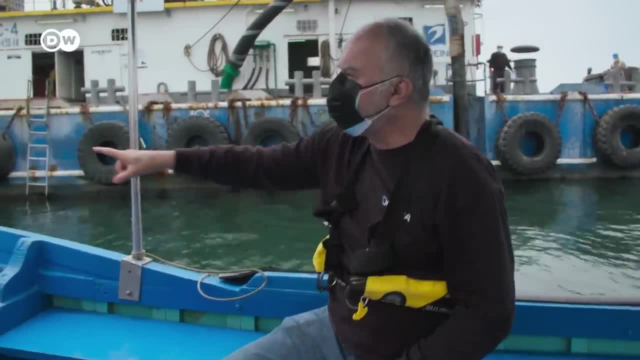 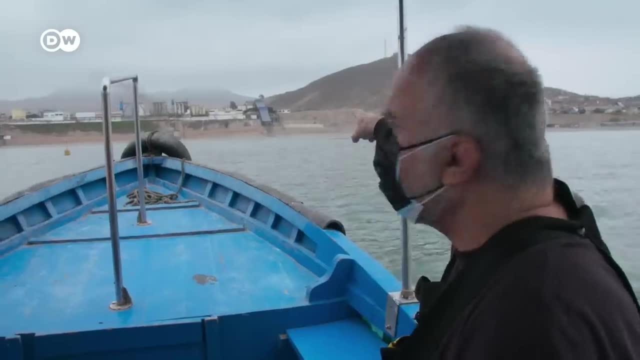 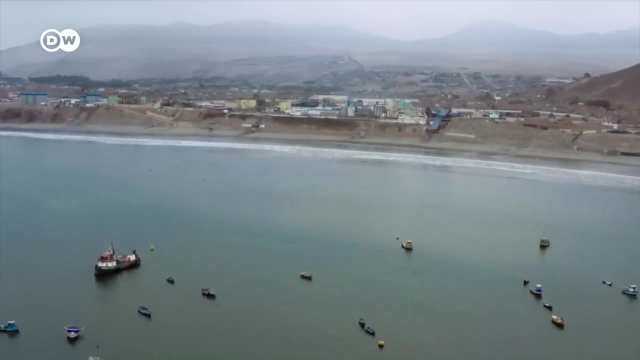 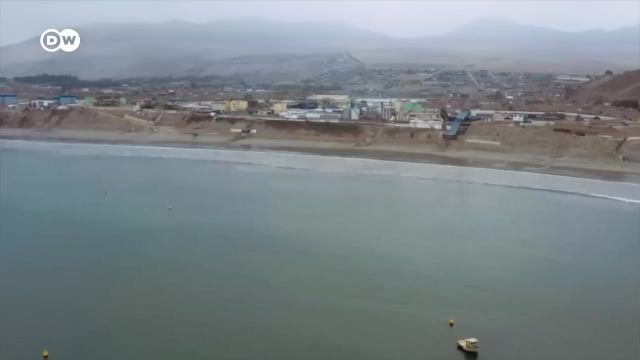 The platforms are anchored in the seabed so that they don't move. They are connected underwater to the fishmeal factory. This blue conveyor carries the fish directly to the factory for processing. We catch four to six million tons of anchovies a year. 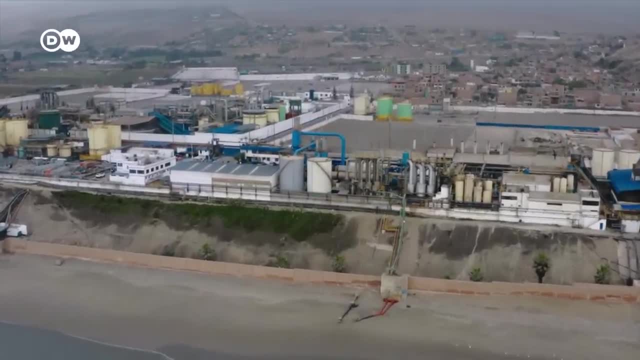 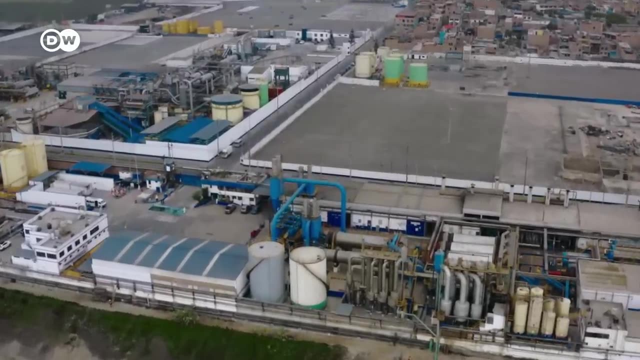 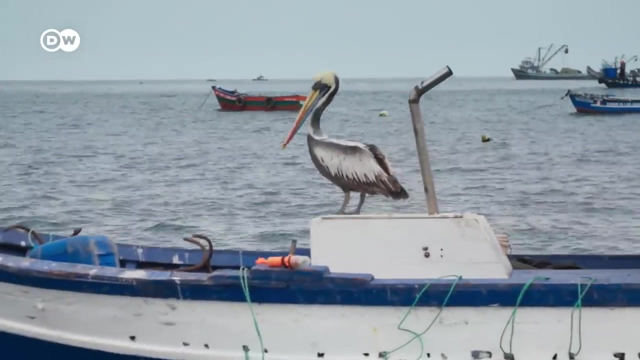 They are made into fishmeal and fish oil. 97 or 98 percent of the fishmeal is exported, 70 percent of it to China. That means that China is one of the biggest buyers of fishmeal. China will make a grab for Peru's fish resources. It's just a matter of time. 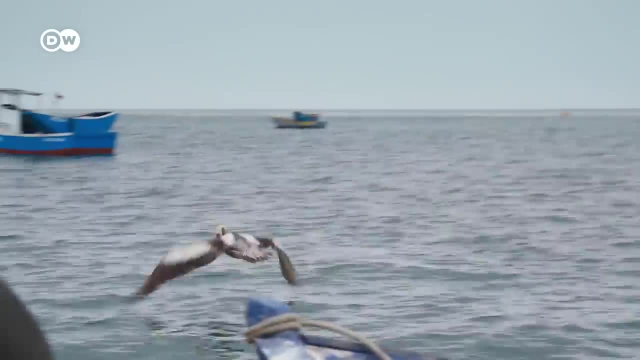 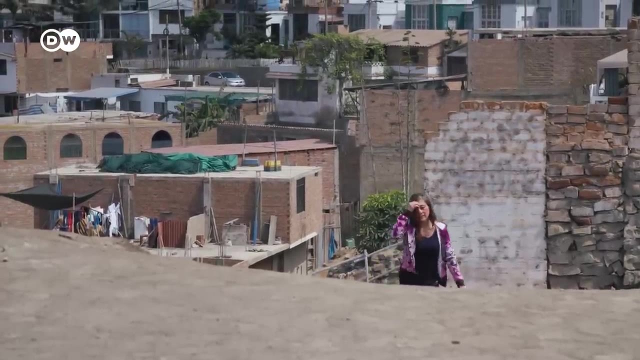 Next to the town and adjacent to a nature reserve, a new port is being built. The port is being built in the area of the Oceana, which is the largest fishing port in the world. China will make a grab for Peru's fish resources. It's just a matter of time. 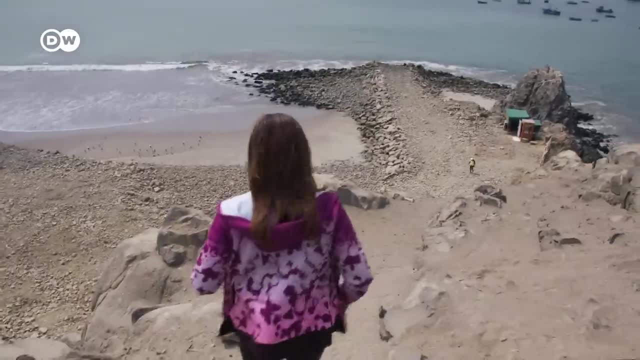 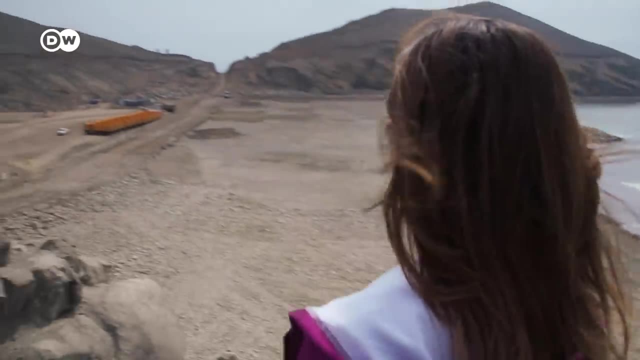 Next to the town and adjacent to a nature reserve, a new port is being built. China will make a grab for Peru's fish resources. It's just a matter of time. Chinese investors are behind the mega puerto or mega port under construction here. 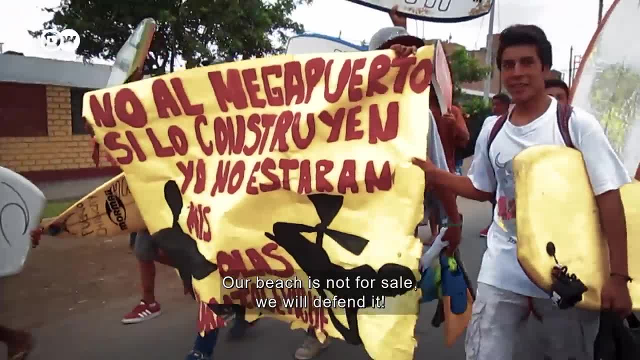 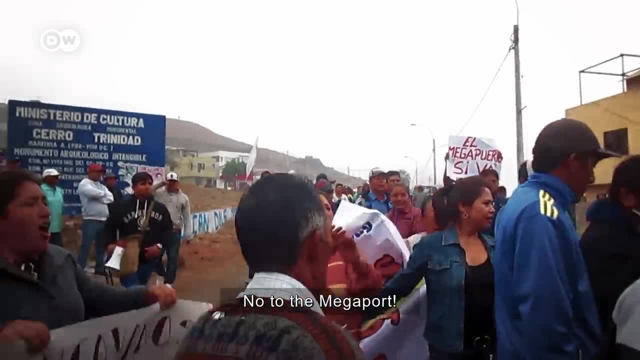 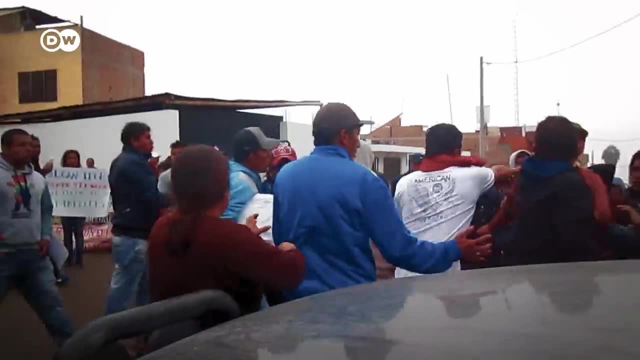 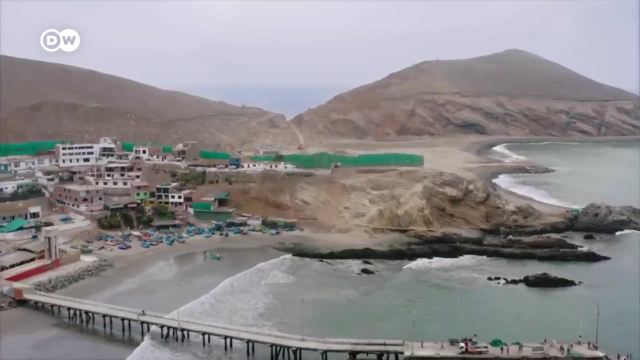 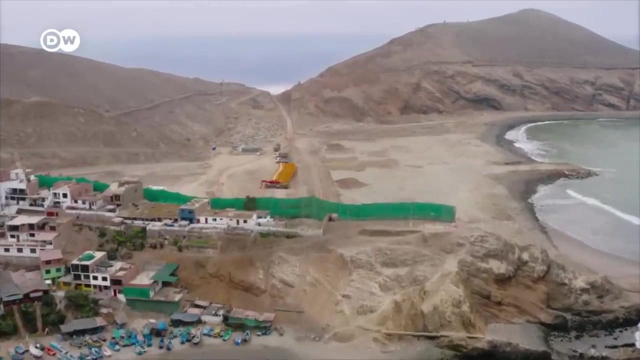 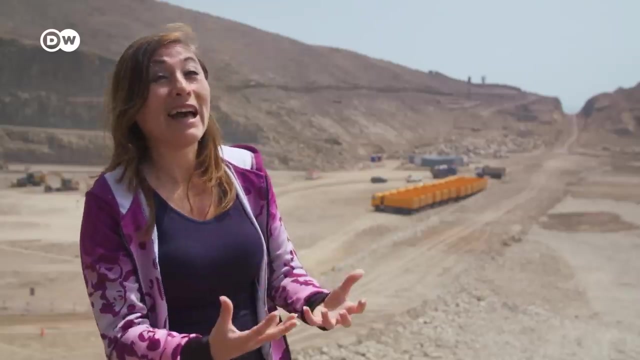 The port's construction has been the subject of debate for years. Ecological and economic arguments balance each other out. The new port is dividing the people of Chiang Kai. Worst of all, they want to steal our identity And they're creating conflict between neighbors. 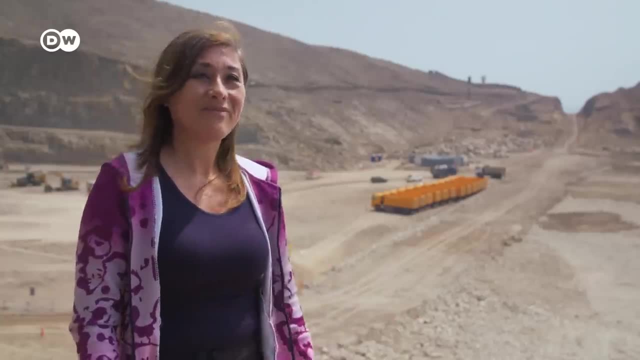 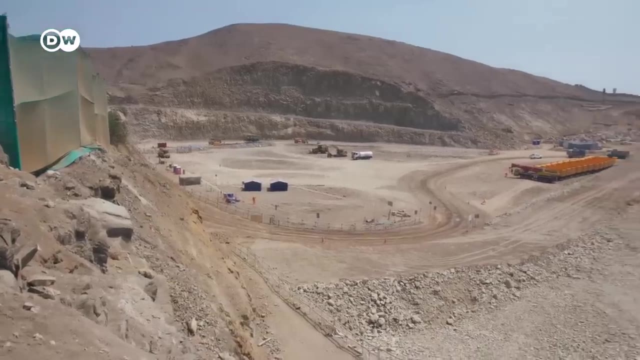 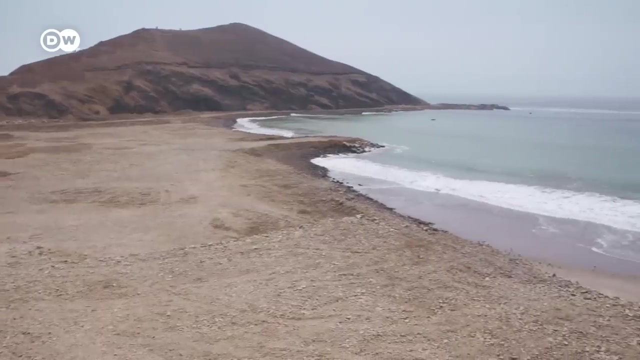 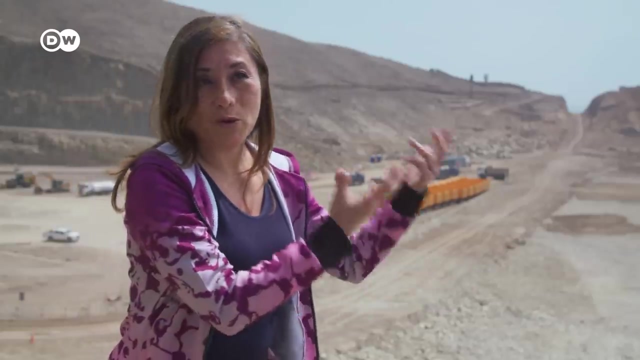 It hurts me because I was born here. The location is great for the Chinese because they aren't just exporting fish meal, They can also export minerals to China and bring their goods directly from China to Peru. The port will be just for them. 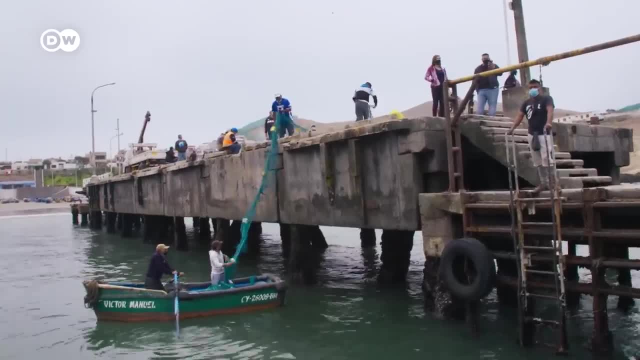 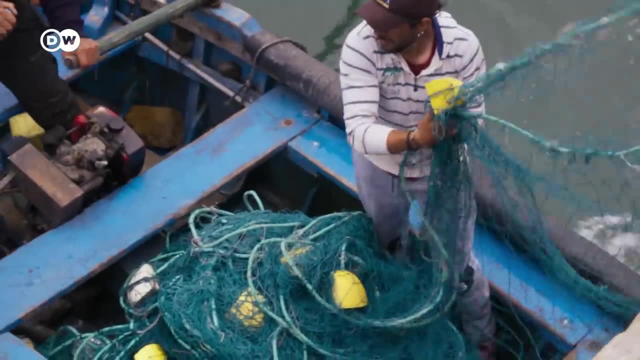 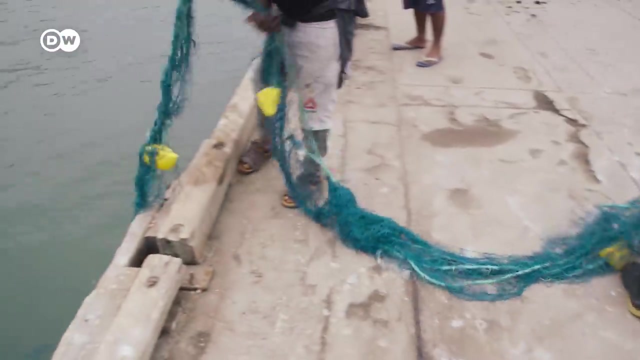 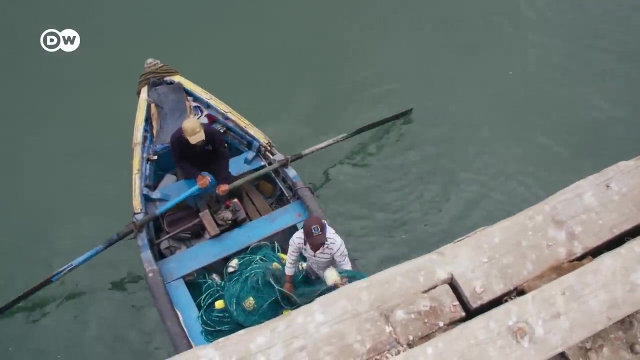 The new port will also compete with the local fishery in Chiang Kai. Chinese deep-sea trawlers will call there and fish the coast, And the Chinese are already illegally tampering with Peru's fish stocks. There is already a conflict. 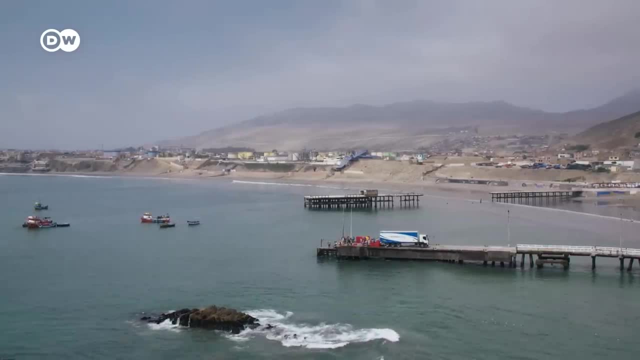 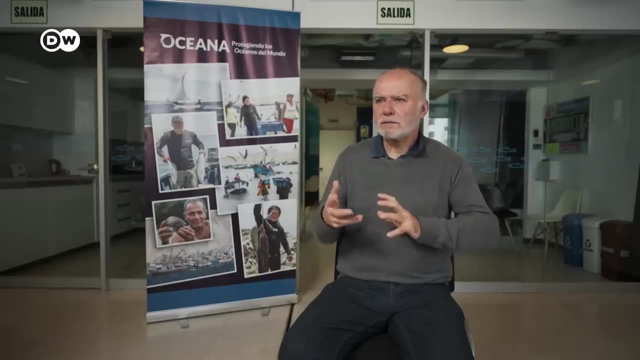 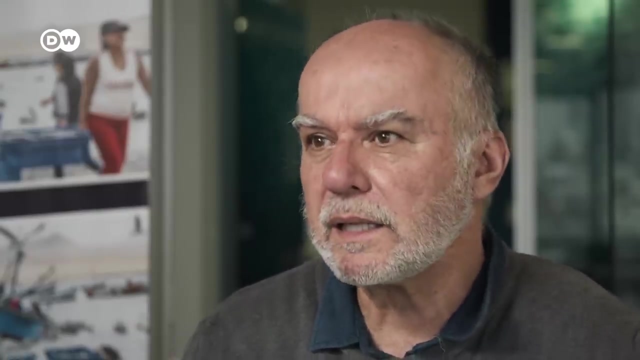 The Chinese fleet is fishing our giant squid, Even though they don't have authorization. They don't have authorization for Peruvian territorial waters. The Chinese fishing fleet has grown massively. Within a decade it has become three times bigger. The platform Global Fishing Watch shows the movement of the Chinese fleet very well. In July the Chinese stay south of the Galapagos. Then they go down the coast to Peru and Chile and even as far as Argentina, And that's part of this conflict with China. The Chinese are going south of the Galapagos. 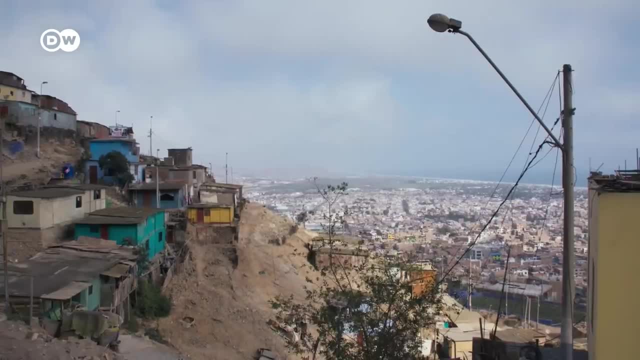 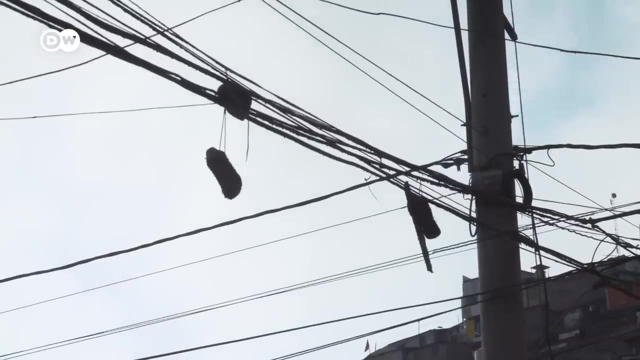 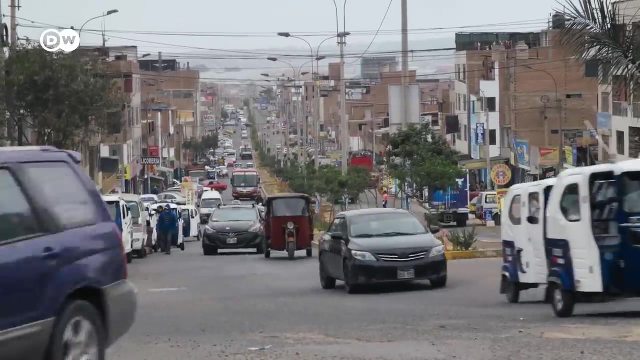 Then they go down the coast to Peru and Chile And even as far as Argentina, And that's part of this conflict with China. Peru is a developing country. Three-quarters of Peruvians work off the books on the grey market without any state social. 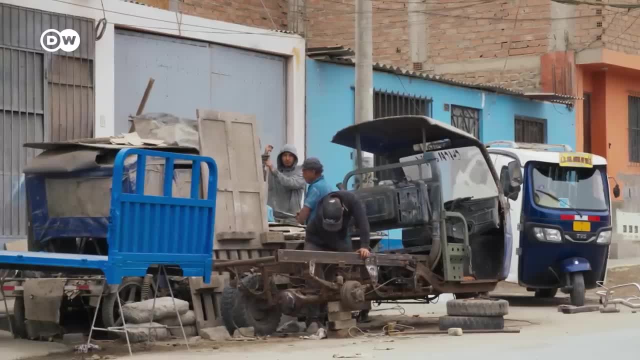 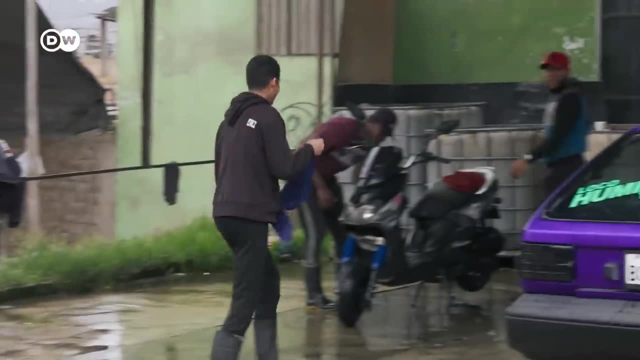 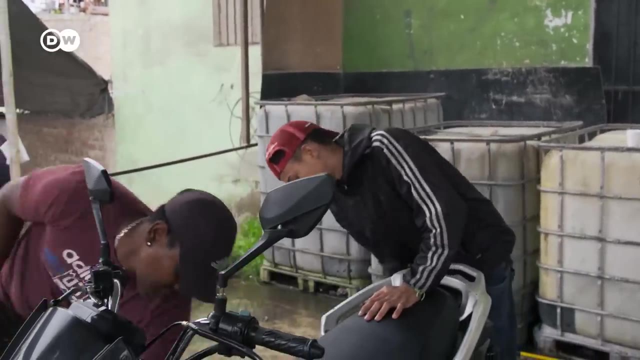 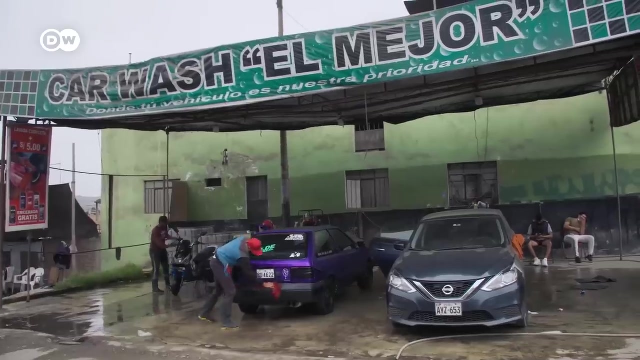 net. No government has been able to create an orderly and sustainable labour market. The well-educated are leaving the country, Another blow to Peru's economy as it struggles to profit from globalisation. No, of course I cannot be satisfied with a system that's left 70% of the population behind. 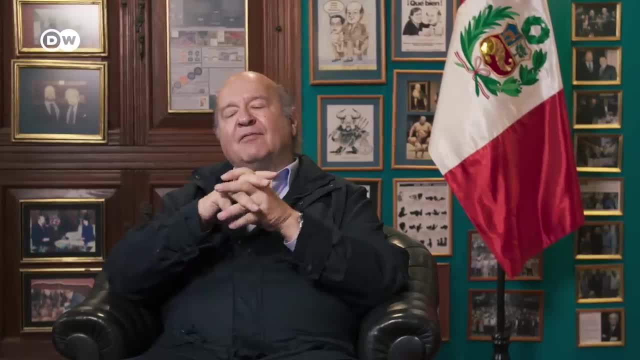 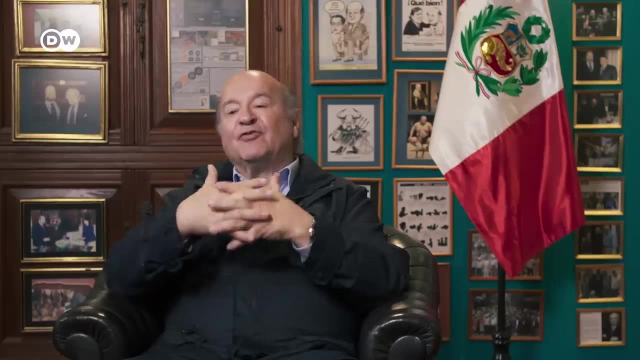 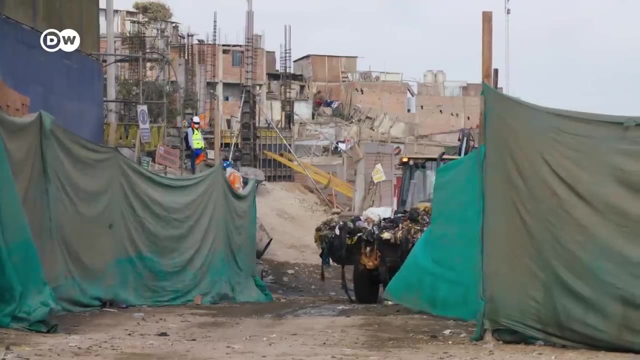 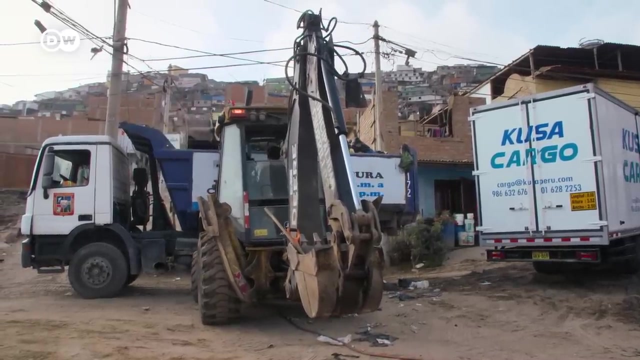 Well, what has changed is that we have now an awareness that globalisation is not and its virtues are not accessible to everybody in the world in the same way. Remember that we always talked about the informal economy, the first being that economy. that. 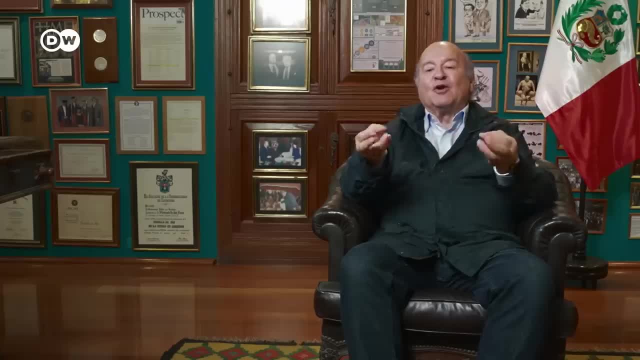 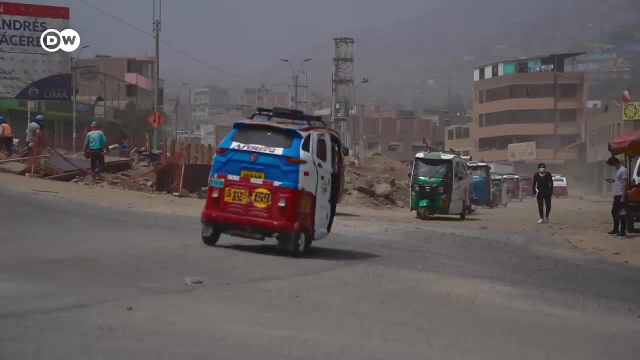 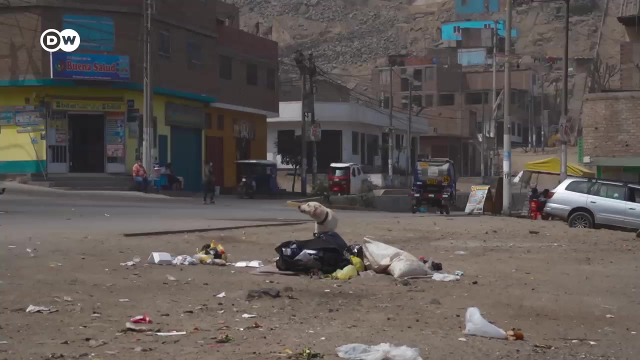 didn't have rules that were connected to the global system. They had local rules, but they were not connected to more global rules. However, Peru has achieved some small successes in the fight against poverty. In 2000, Mi Banco was the first bank in Peru to grant loans to the very poor, no guarantee. 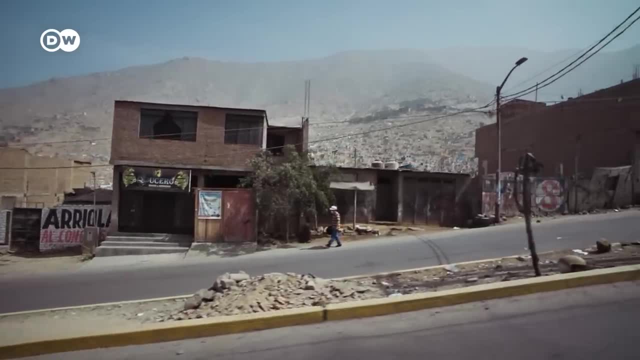 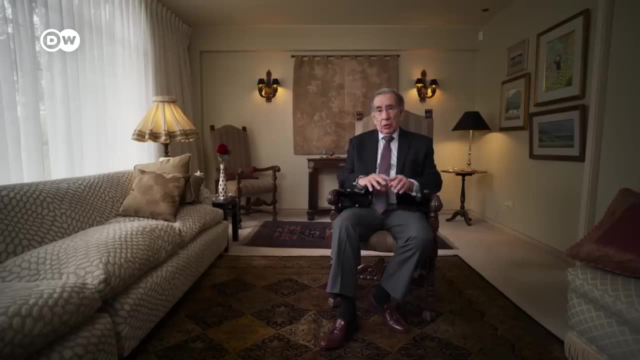 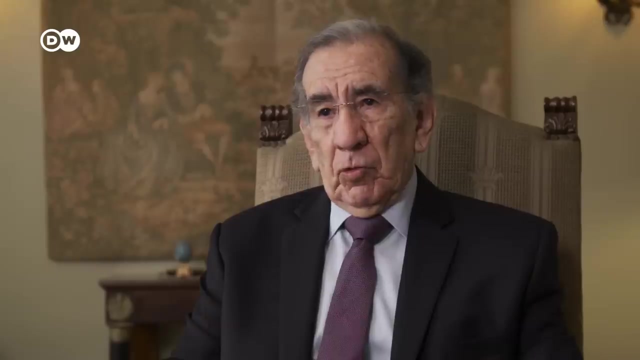 required So-called micro-loans. The informal economy is a major problem in Peru. It is a consequence of migration, with many people coming to Lima from rural areas and the Andean region. That's why we started giving loans to the rural population. 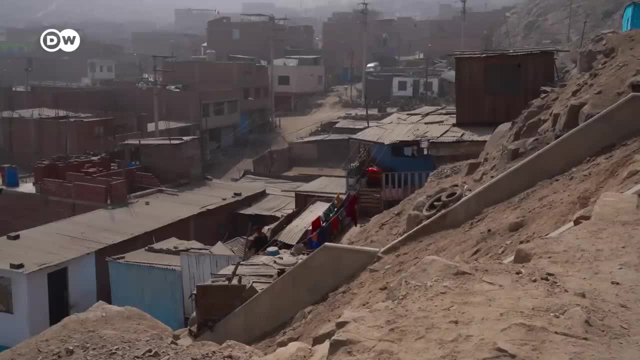 That's why we can now give loans to the rural population. That's why we can now give loans to the rural population. That's why we started giving loans to the rural population: Helping people to help themselves while integrating them into the national economy. 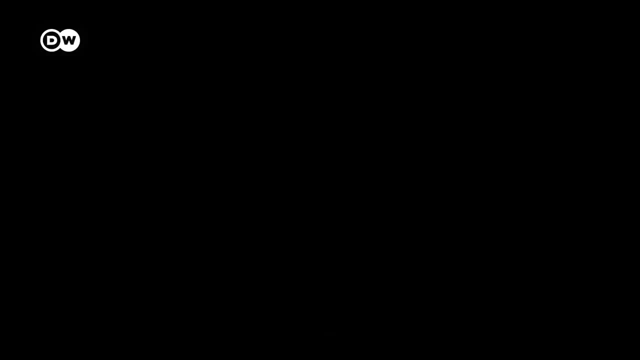 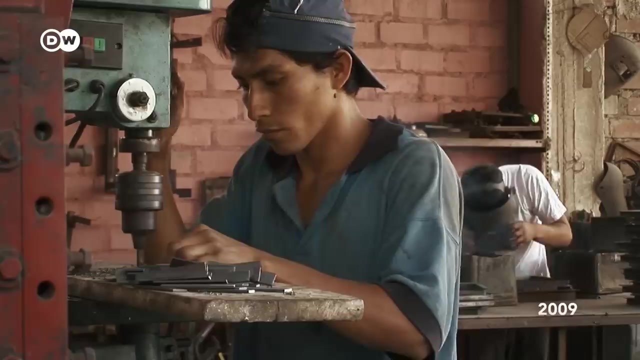 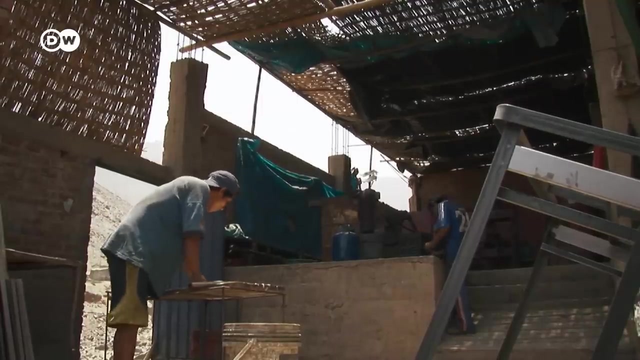 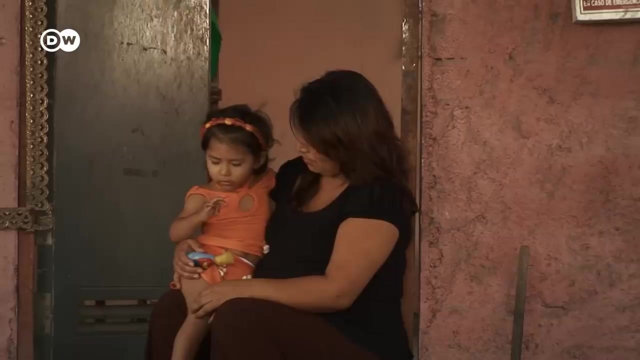 That was and is the goal of Microloans 2009.. A visit to Julio Solis: His company makes gas stoves. A loan from Mibanco allowed Julio Solis to expand. I couldn't get anywhere because I didn't have any money. 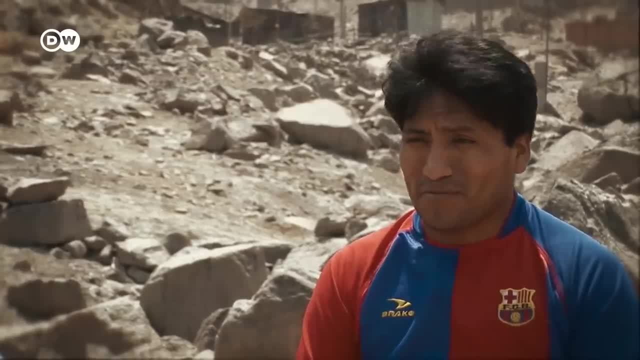 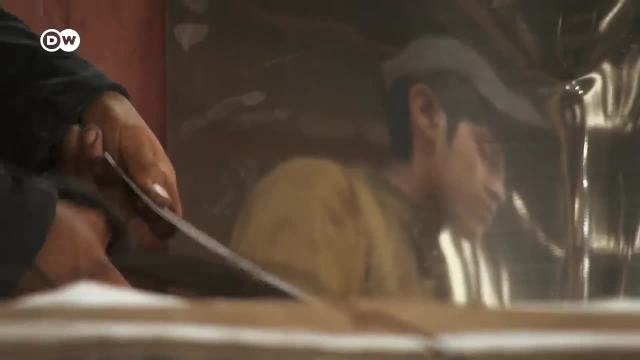 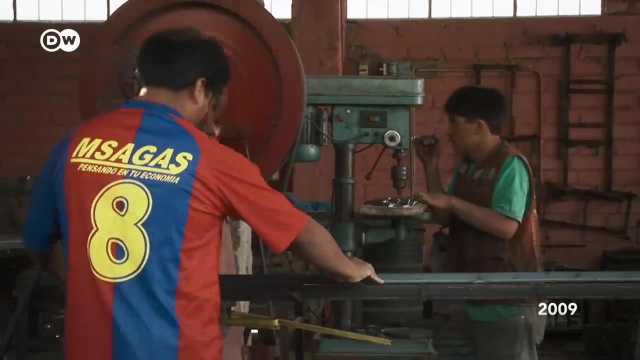 So I knocked on the doors of several banks looking for financing, But they refused and gave me nothing. A lot of young people are looking for work in the factories. By hiring five or six people, I can help my country and give something back. 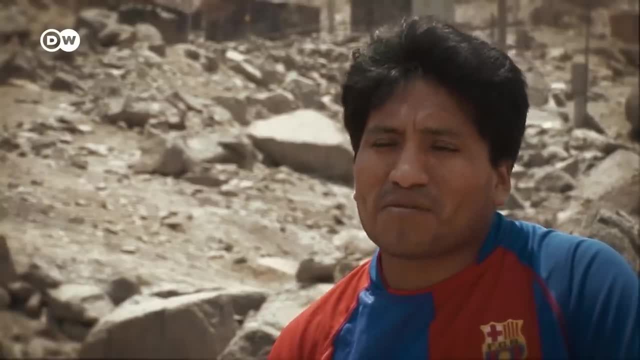 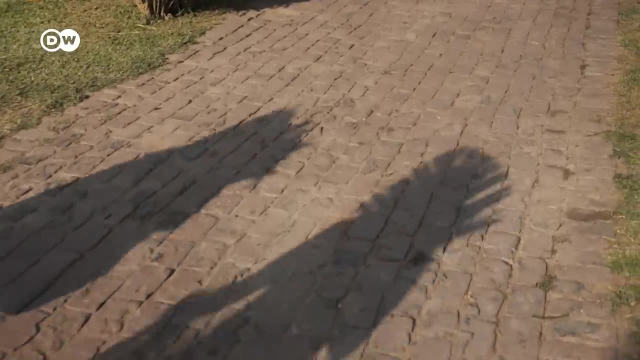 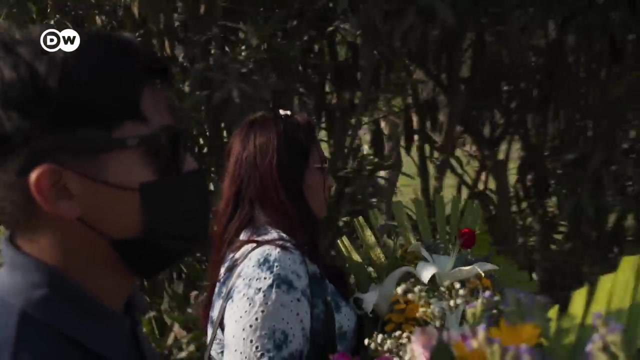 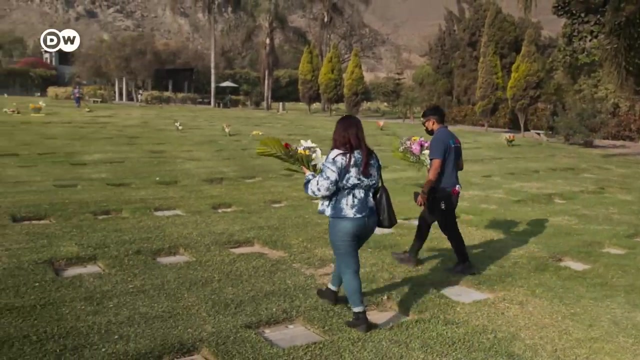 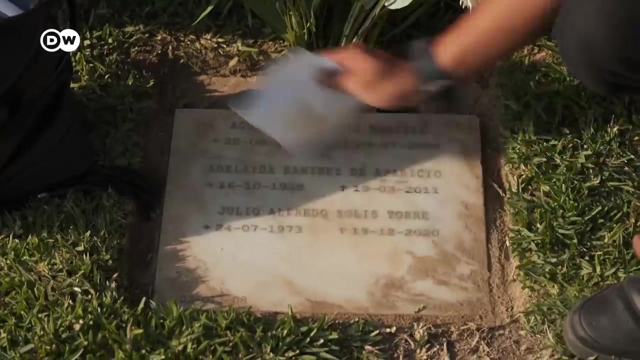 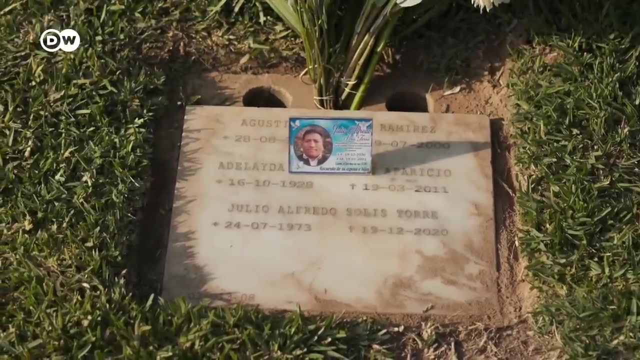 That is my dream. Twelve years later, Marleny Aparicio and her eldest son, Franco, take us to a cemetery near Lima. Julio Solis died in December- December 2020, at the age of 47.. He died a year ago. 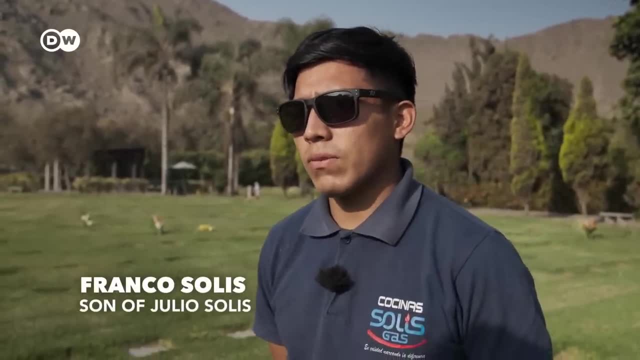 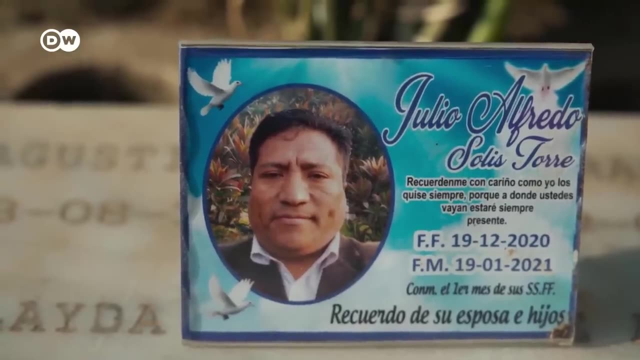 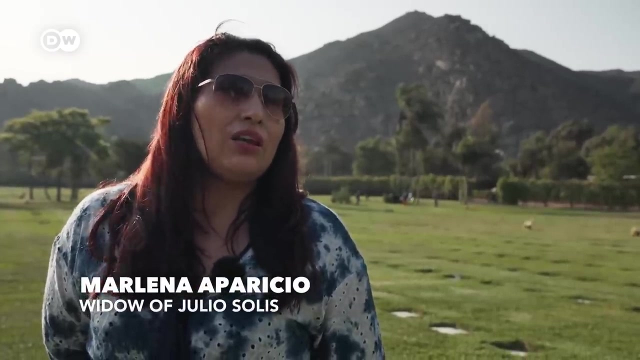 A lot of families have been affected by the pandemic in Peru. The virus took our father too. We will continue his work. He was a man of integrity who was determined to make a difference. He did everything for his family, for his children. 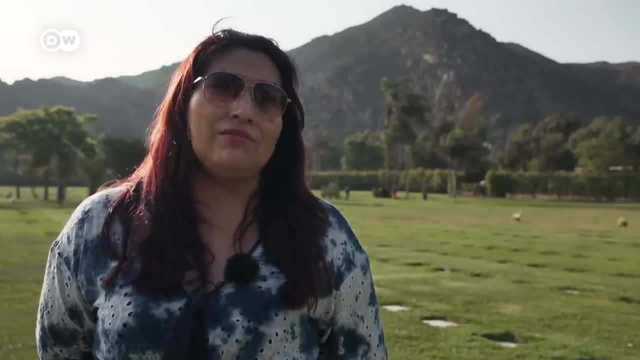 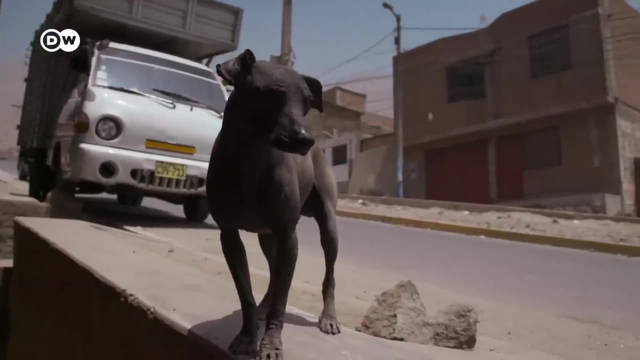 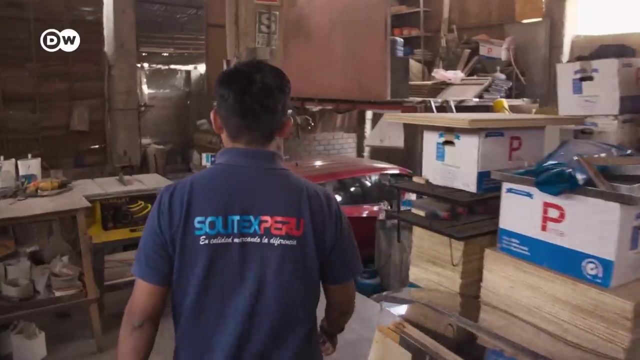 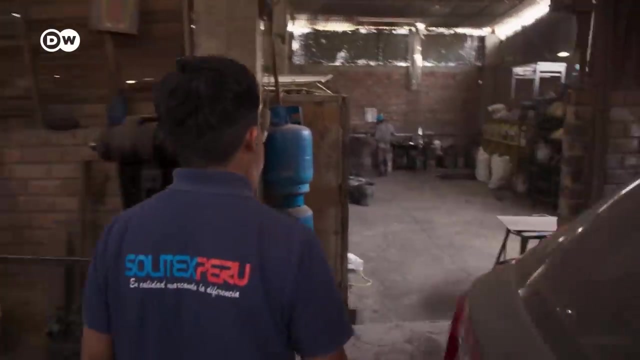 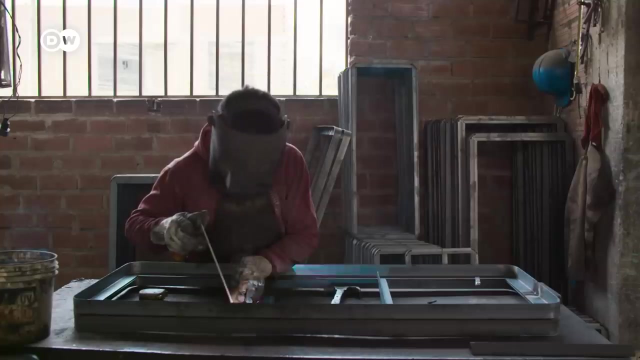 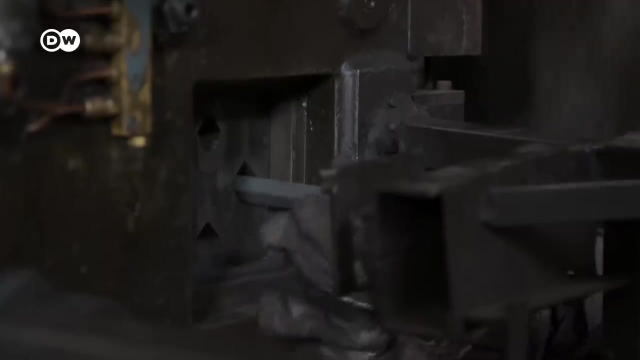 His family was always the most important thing to him. I sent him a kiss in heaven. The small factory hasn't moved, But now it's twice as big. Fifteen men and women are permanently employed here. I want to tell you something. 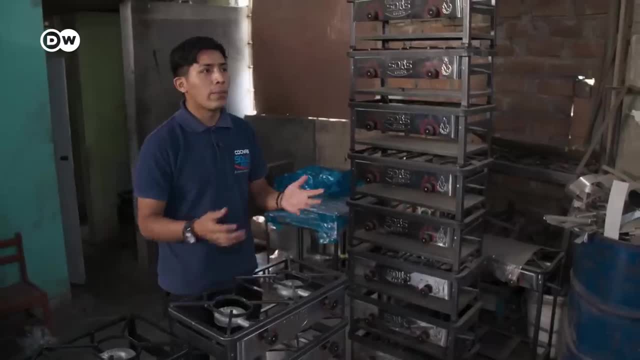 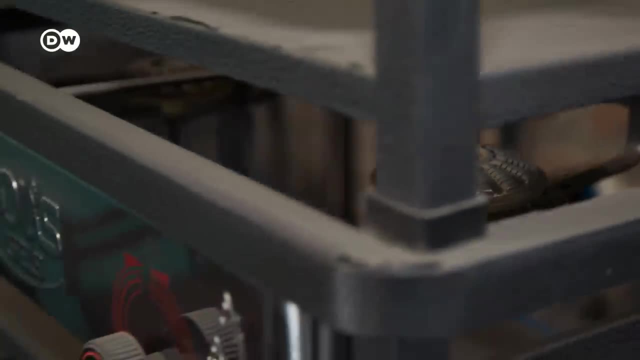 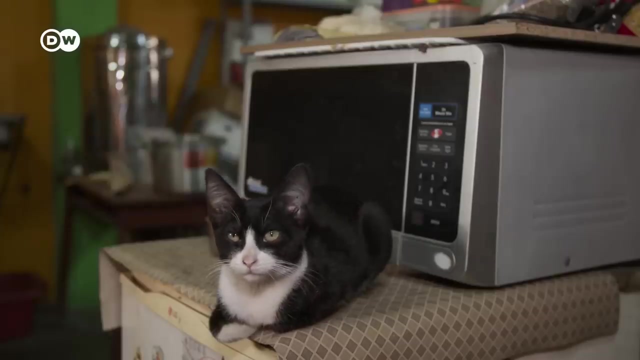 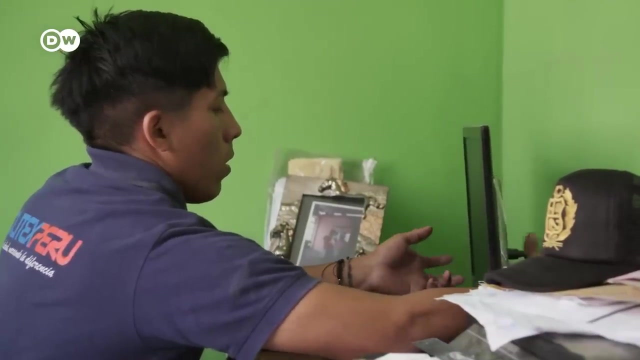 I was in a restaurant in Lima. They were cooking with our stoves. It's nice that they use our products to cook. They are using them to prepare food for people. That makes me happy. My father wanted to sell our products on the international market. 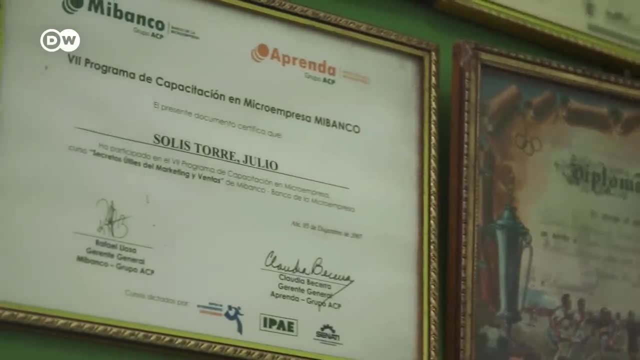 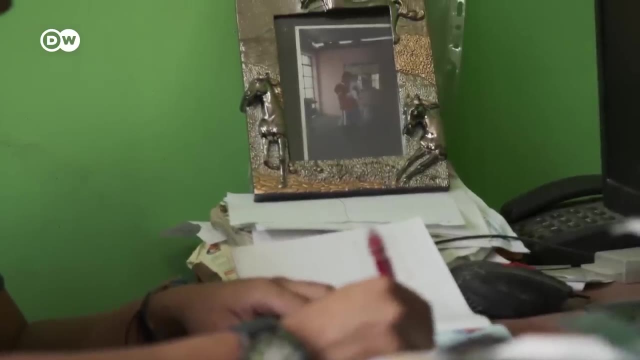 He wanted to do it for his family. My father wanted to sell our products on the international market. His goals were Chile and Bolivia. We want to make his idea a reality. Me, my mother, my brothers and sisters, we all want to try". 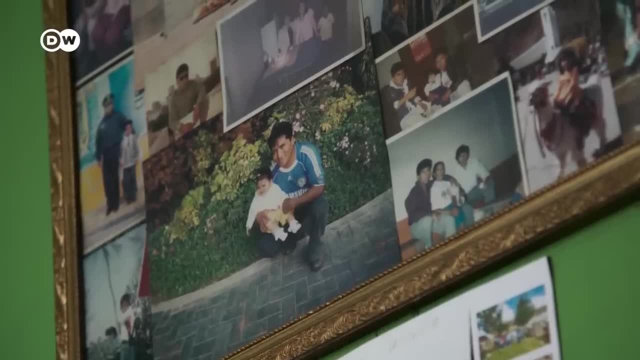 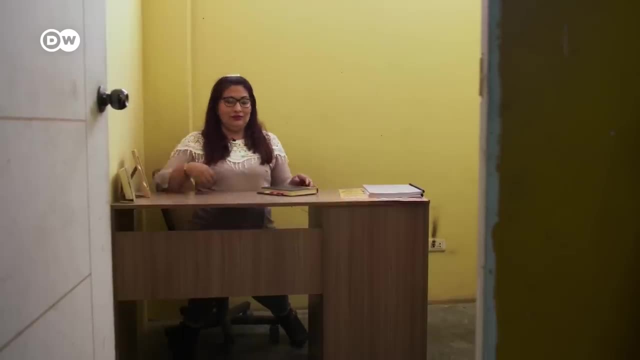 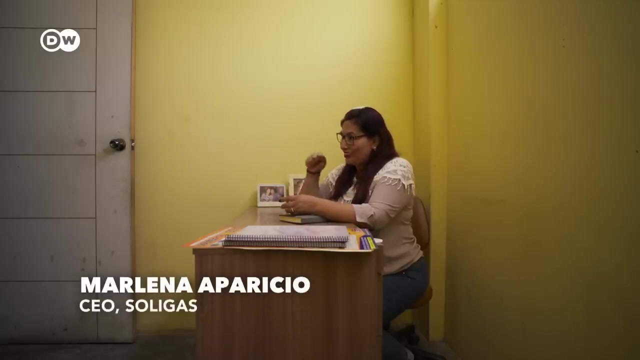 It was our first loan. Just a small amount, about a thousand Peruvian sol, which is about 250 US dollars. Hundreds of banks slammed the door in our faces back then. Now they keep knocking on our door, wanting to give us a loan. 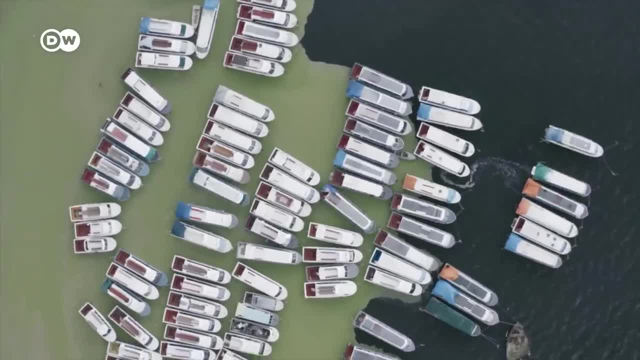 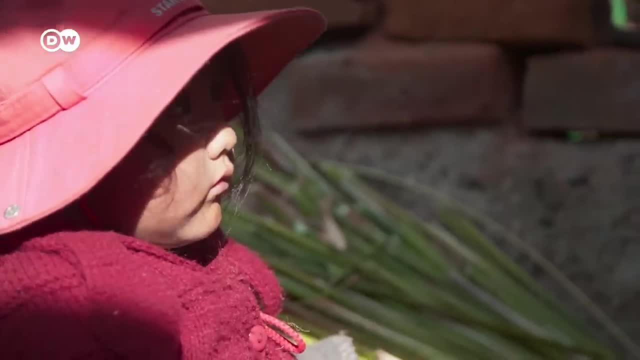 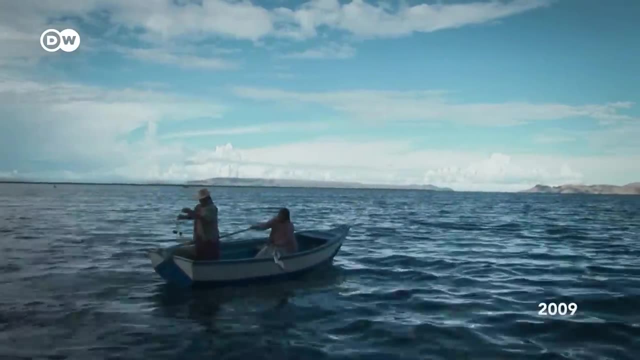 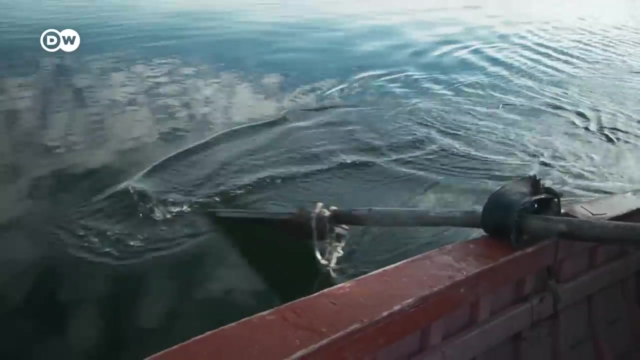 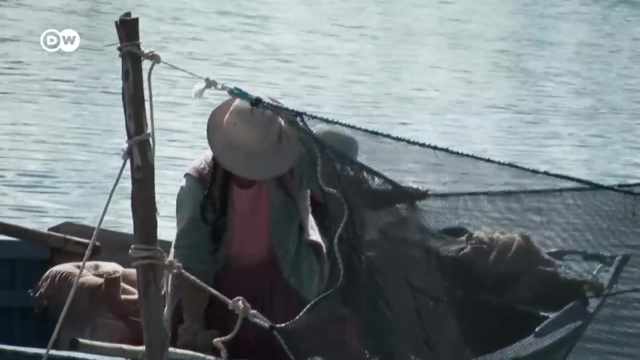 But we don't need a loan now. The region around Puno is one of the poorest in Peru. In 2009,, Pro Mujer, a development organisation, offered microloans to fisherwomen. The aim of Pro Mujer is to encourage women to improve their lives. 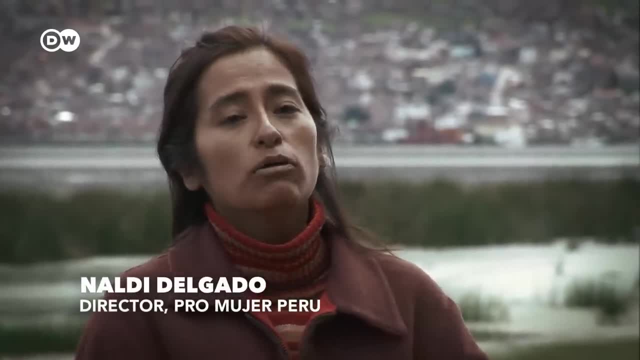 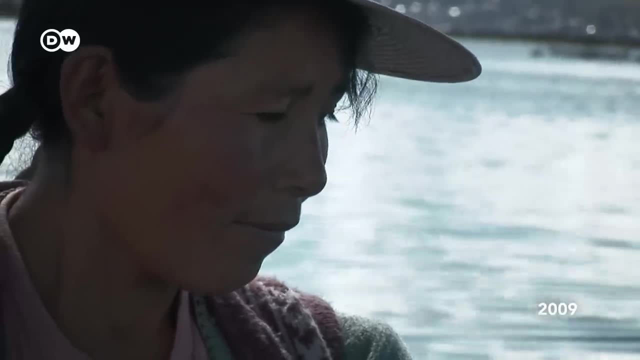 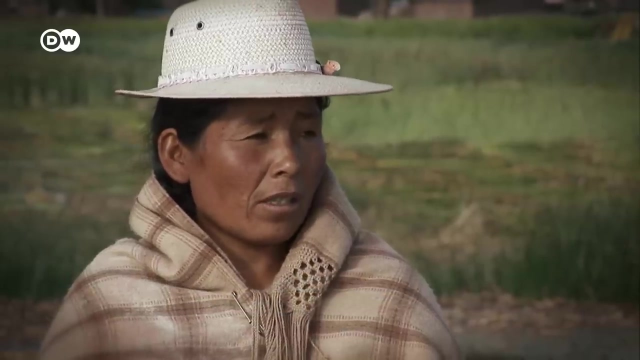 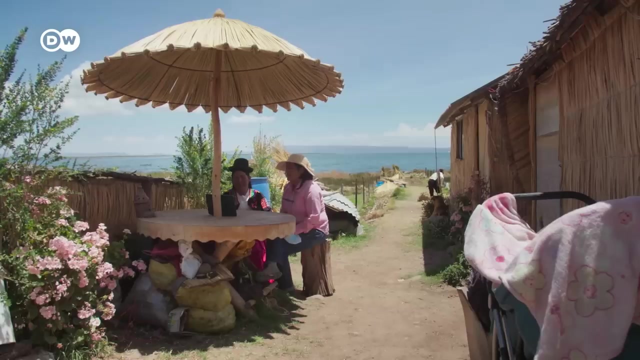 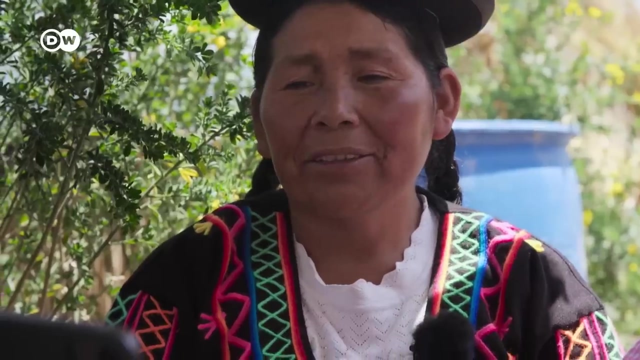 giving them loans based only on their worth". My life has improved. I used to often lack money. Now I am happy. My children can go to school. I can help my family. Thirteen years later, Gloria has given up fish farming. 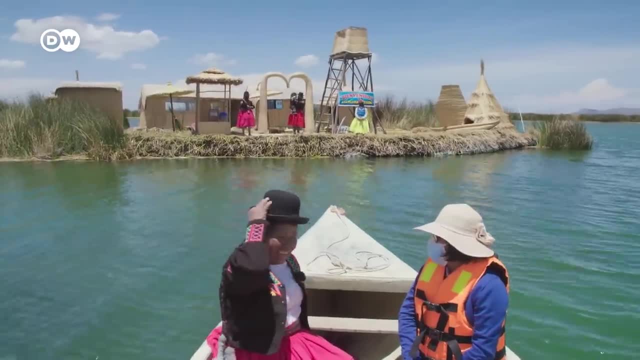 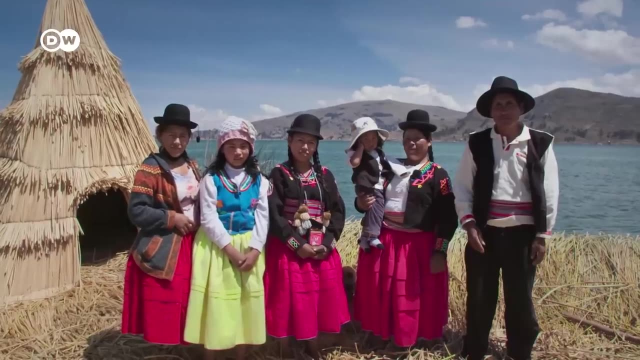 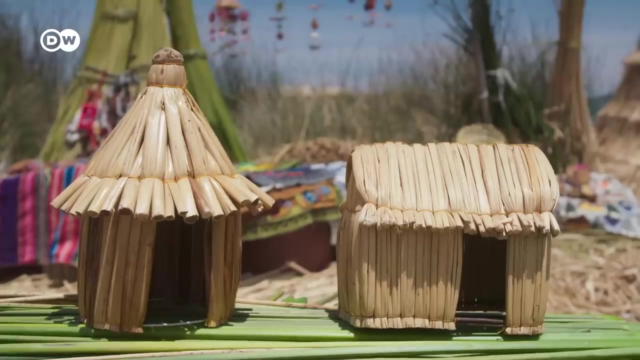 The polluted waters of Lake Titicaca constantly killed her fish. Her family now wants to go into tourism with an island made of reeds. They've invested the money they earned from fish farming in the new project. A loan of about 100 US dollars is still making a difference today. 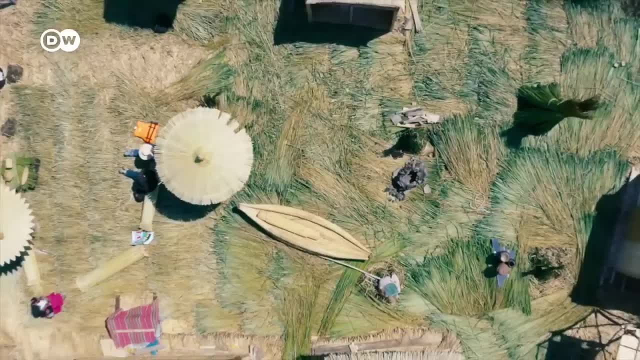 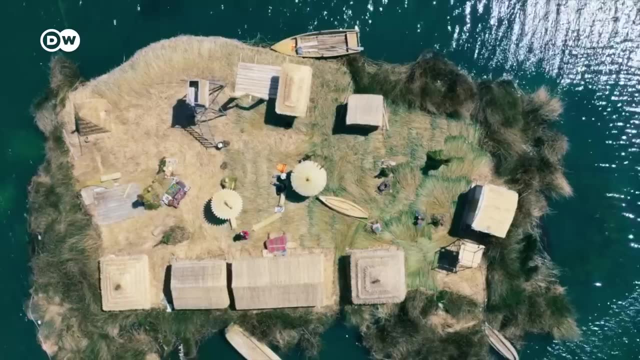 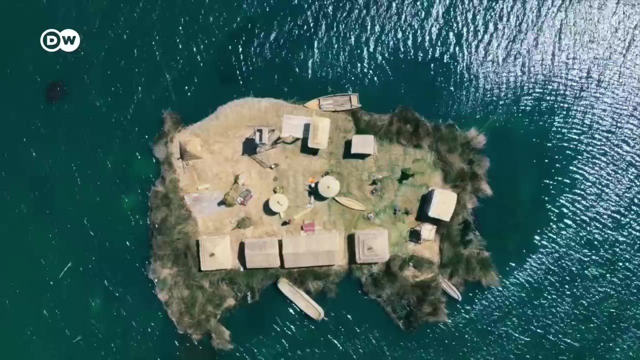 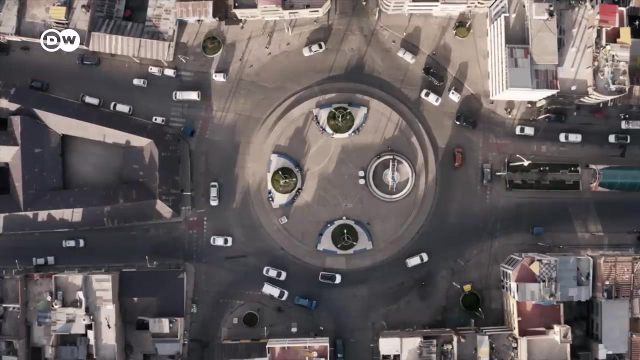 The organizations, the NGOs that started the microcredit programs caught the attention of the big financial institutions. In the beginning, they took big risks. This is a very good example of the need for innovation to promote development and improve the living conditions of the most vulnerable populations. 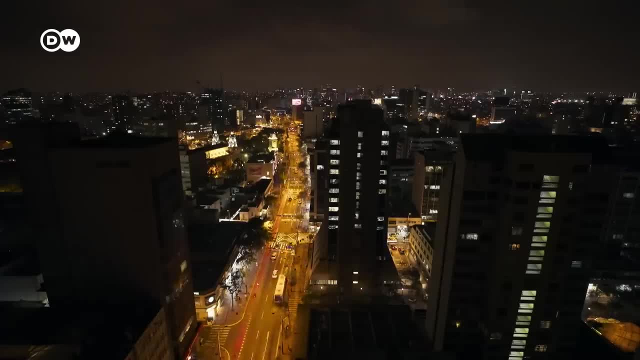 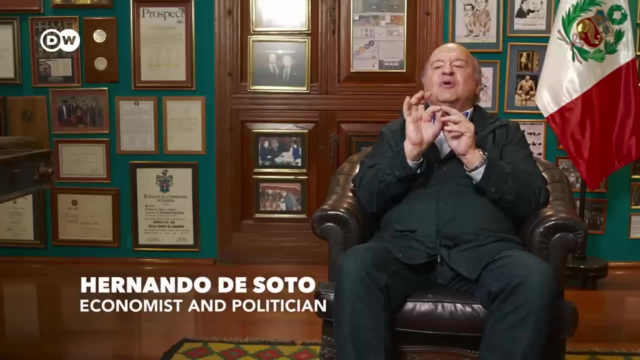 What I like about microcredit is that it is one way of getting to the solution. I mean, first of all, it is that people do want credit, And the fact that you adjust to help poor people is good. Microcredit is a step in the right direction. 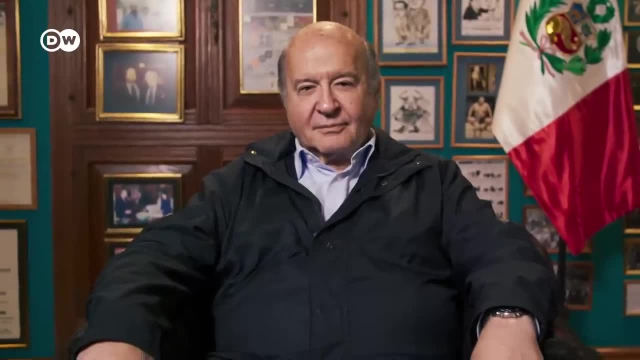 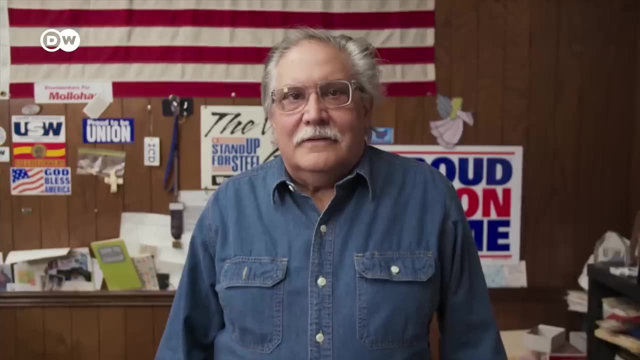 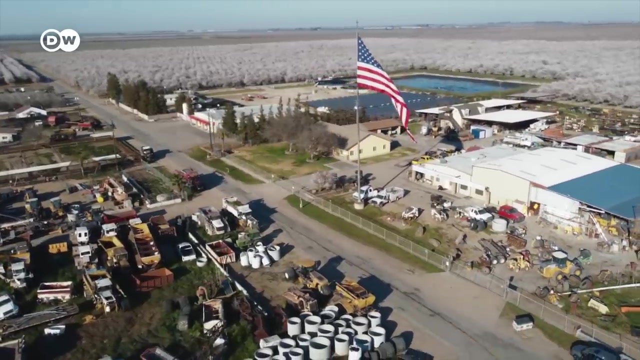 It alleviates, but it's not a final stop. Globalization is in crisis. The world trade system has led to fewer and fewer winners. Protectionism and nationalism appear to succeed, but it's not the best who win, but the richest. 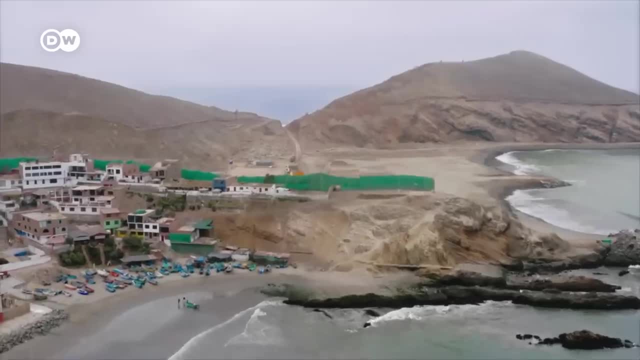 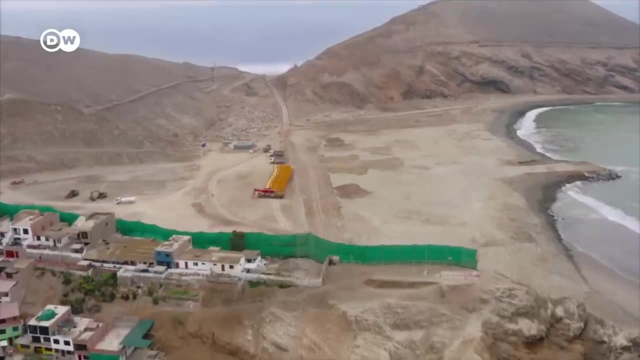 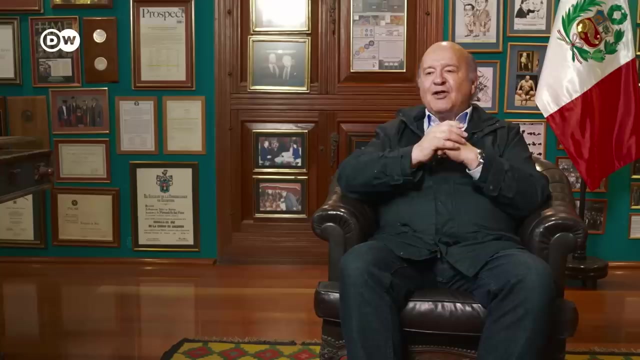 The geopolitical goals of the powerful mean that many poor people are the losers. Yet globalization seems to be the only alternative. Globalization, in other words, is still a good thing. Of course it is. It's a division of labor, It is the bringing together of humanity above nationalism, above religion.